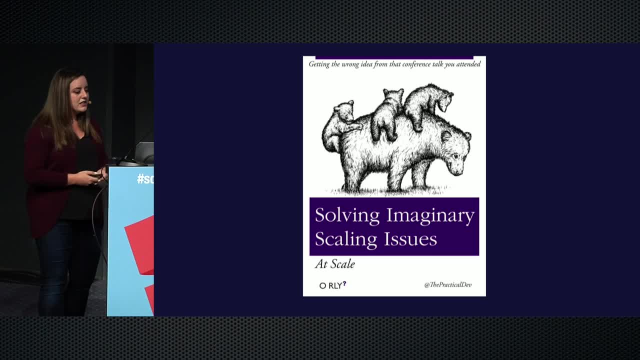 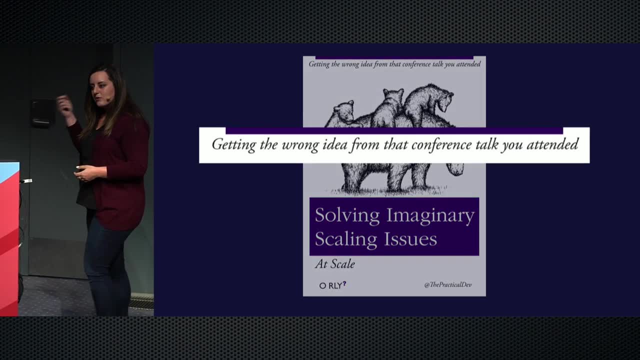 about syntactic sugar and fancy abstractions out there. So if you reflect on the talks that you've already seen and the ones that you're going to go to today, you're going to hear a lot of things. Keep this in mind so that hopefully this doesn't happen By. 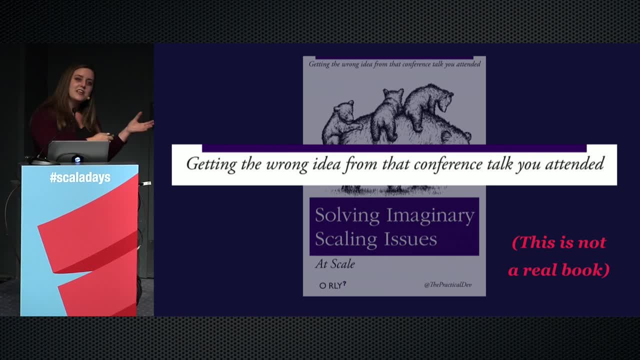 the way, this is not a real book and I had to mention that because the last time I gave this talk, somebody asked me where they could buy it. so just for the record, this is farce, All right, Despite the fact that functional programming has been around for over 50 years. 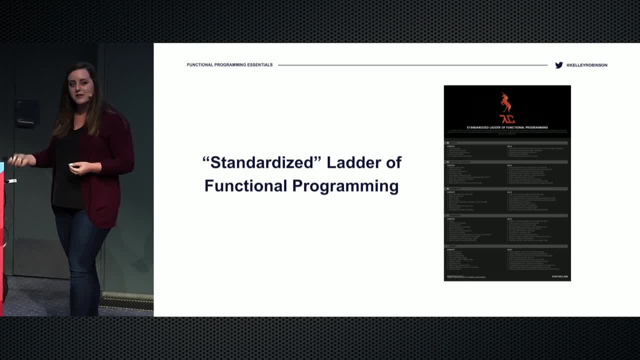 we're still arguing about how to define it, and this is especially relevant because last year this so-called standardized ladder of function was removed. We're still arguing about how to define it, and this is especially relevant because last year this so-called standardized ladder of function was removed. 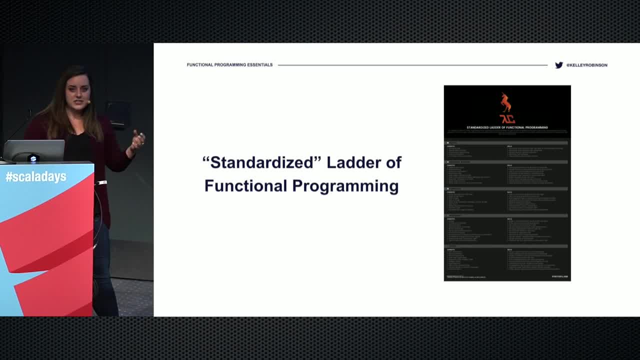 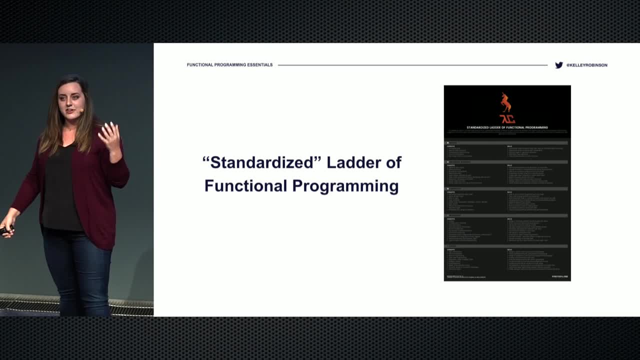 functional programming came out, and I was talking about this with someone yesterday and if any of you were in the keynote this morning and woke up for it, this is somebody that was trying to be provocative by creating this ladder. You can't read it, but it goes. 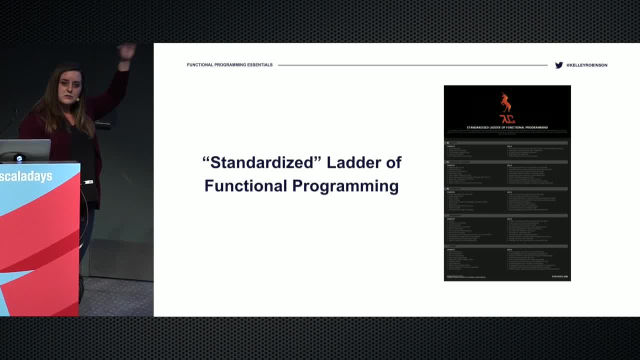 from beginner skills at the top, with skills like immutable data, all the way down to expert with skills like graph reduction and profunctor optics. That's cool, but people were basically trolling and here I am up here having the emotional reaction to it. 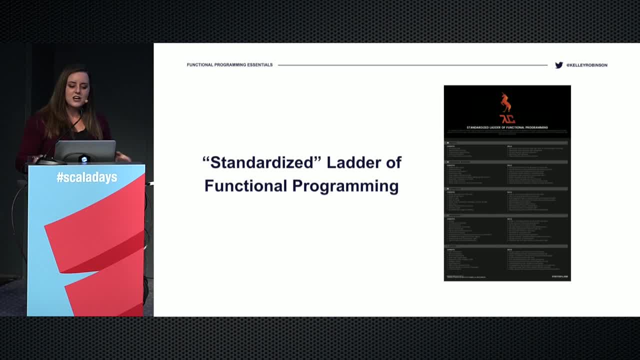 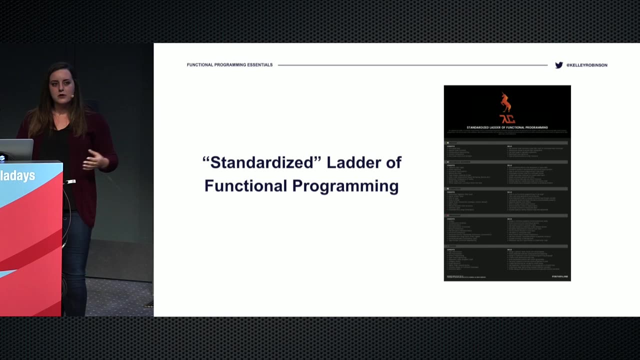 But this is all in support of having a discussion around these topics. So we'll come back to this, don't worry, but I introduce it now to frame our discussion around the idea that there are a lot of these so-called skills and topics that we use and talk about when we talk about. 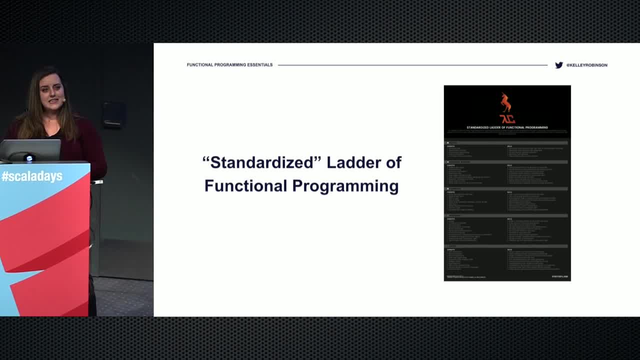 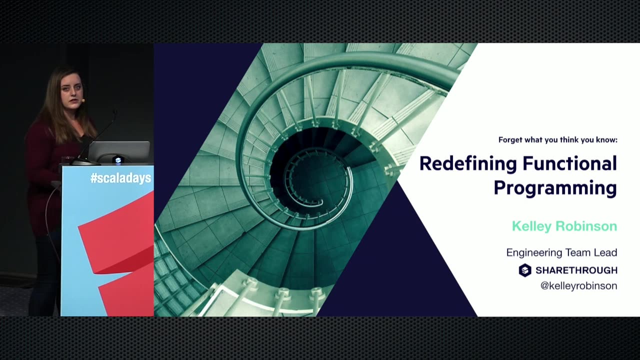 functional programming, And I think it's really easy to get caught up in the jargon and forget the core principles that really make functional programming what it is. And that's what I'm here to talk about: the essentials of functional programming and why that matters to our community. My name is Kelly Robinson. I'm an engineering manager. 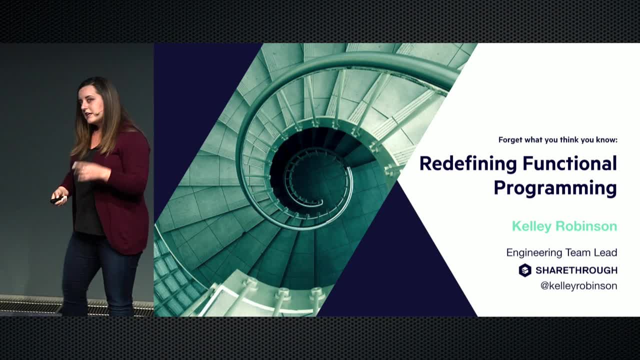 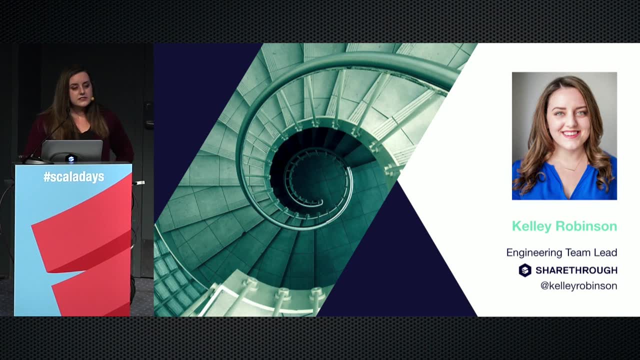 at Sharethrough in San Francisco. We are an ad tech company keeping the internet free. You're welcome. So I've been programming in Scala for about four years. These days, I work mostly with a team of Scala developers. We're bringing data science into the organization. 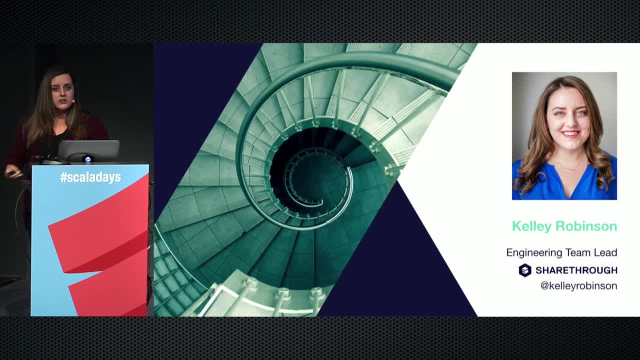 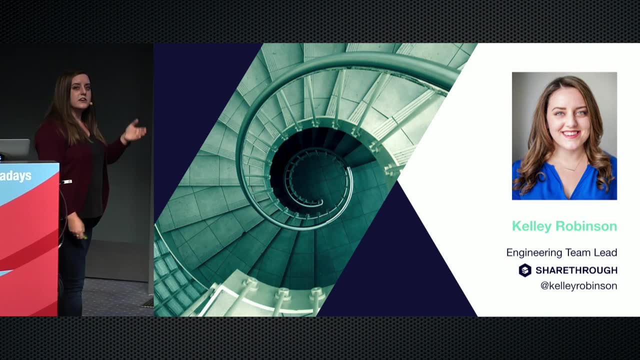 so if anybody's in a similar role and wants to talk about how you use Scala and Spark Science, I'd also love to talk about that. I also like complaining on the internet. That's my Twitter handle. Be warned: my Twitter right now is a mix of rants about tech, US politics. 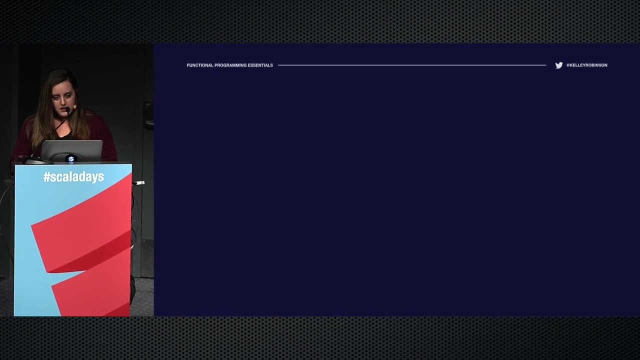 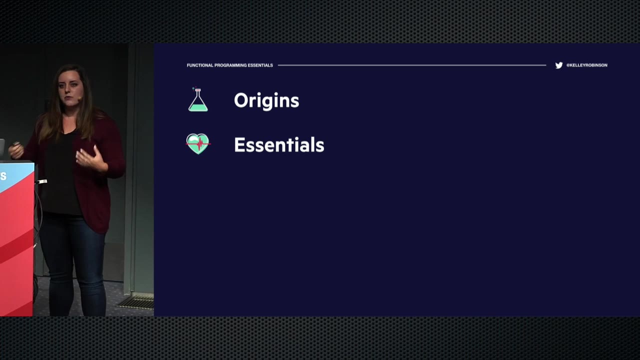 and the like. So you've been warned. Okay, Let's talk about what we're going to learn today. So we'll start with some origins. look at a little bit of history for what functional programming is and how we got to this point, define the essentials and then we'll talk. 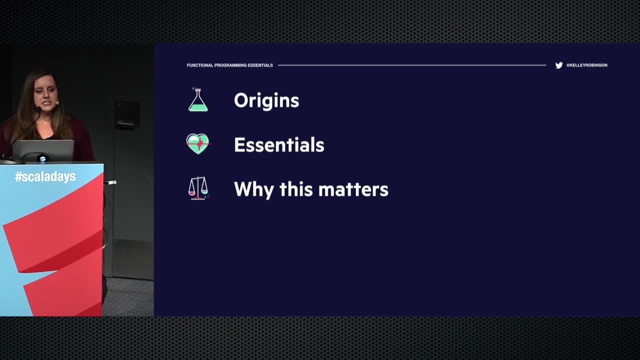 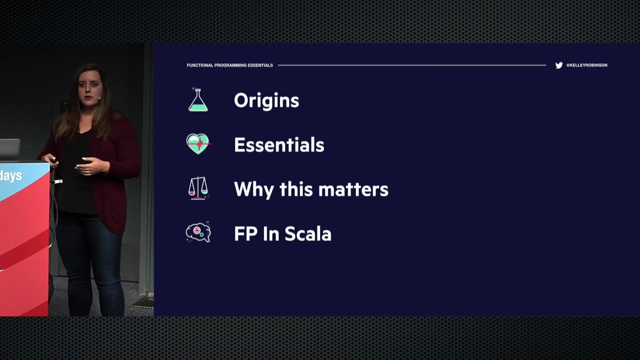 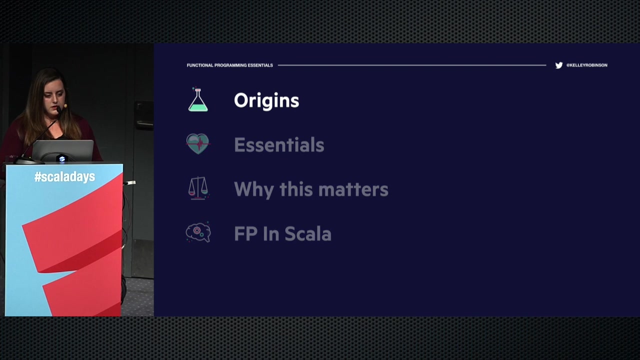 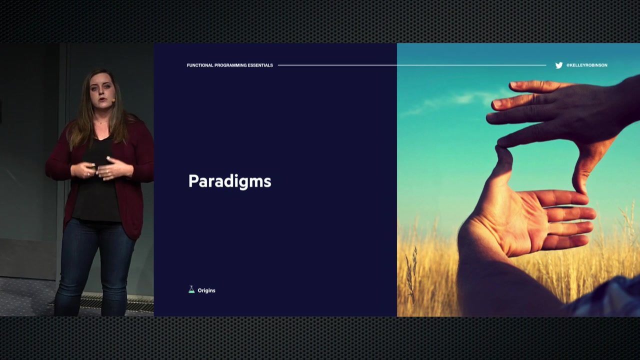 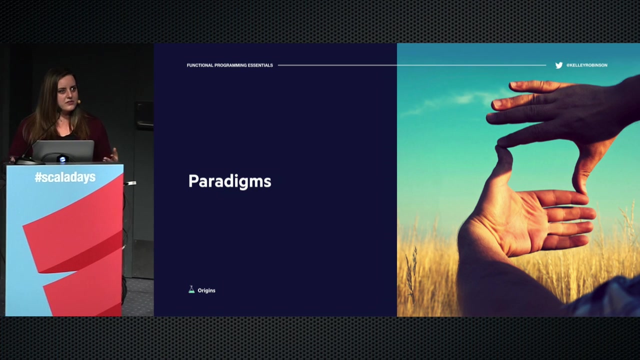 about why this matters. So, first of all, when we talk about functional programming, we call functional programming a paradigm. What do we mean when we say paradigm? A paradigm is a style or a way of doing something. It is not a concrete thing like a language. You can program in a style, like functional. 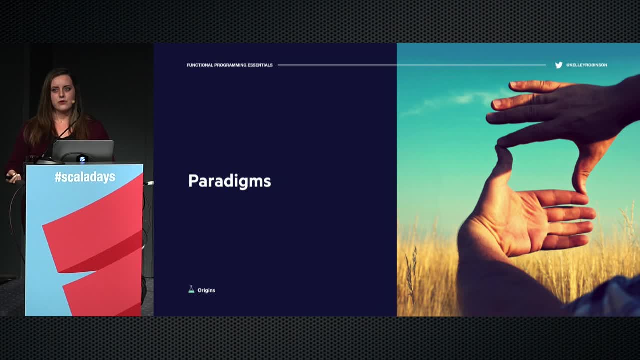 programming in any language, but some languages make it easier to program in that style than others do, And that's an important distinction to make right away. Like I mentioned, it's just a style and you can do it in whatever language you choose. Scala is an example of 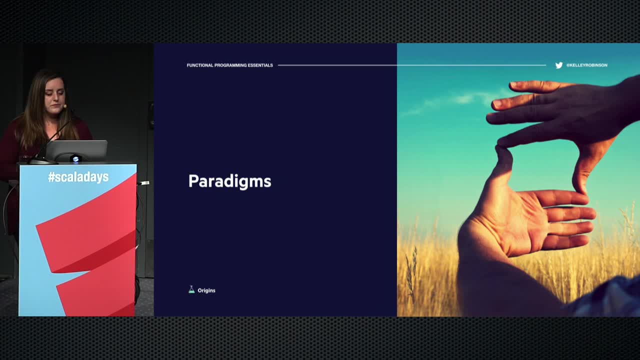 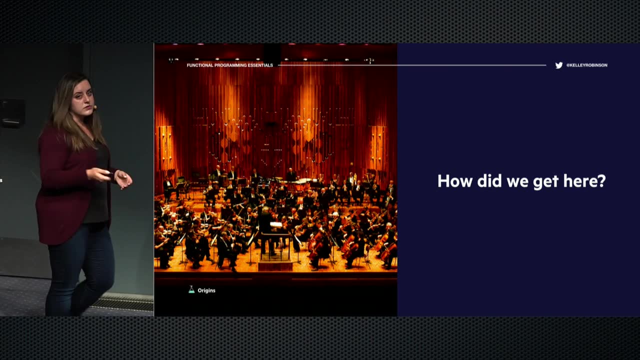 a language that makes it easy to program in the functional programming paradigm, And we'll talk about reasons for that later. How do we get here? How do we get to this paradigm? So José Calderón, who helped me a lot with this talk, put it very well. He said in the: 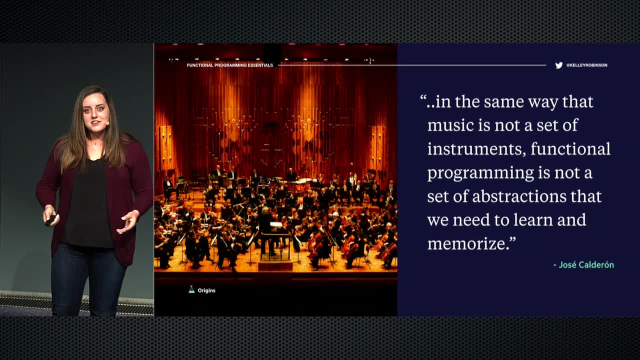 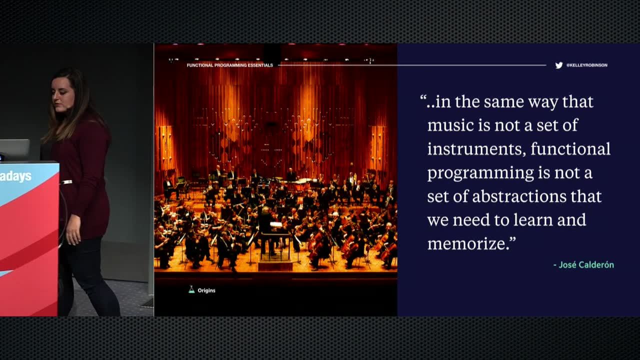 same way that music is not a set of instruments, functional programming is not a set of abstractions that we need to learn and memorize. And he goes on to say that functional programming is an approach to solving computational problems. an approach to solving computational problems. 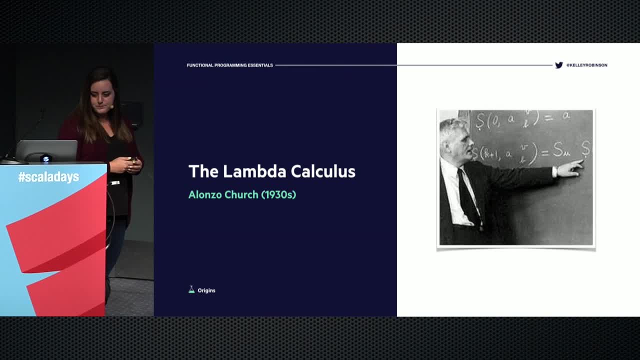 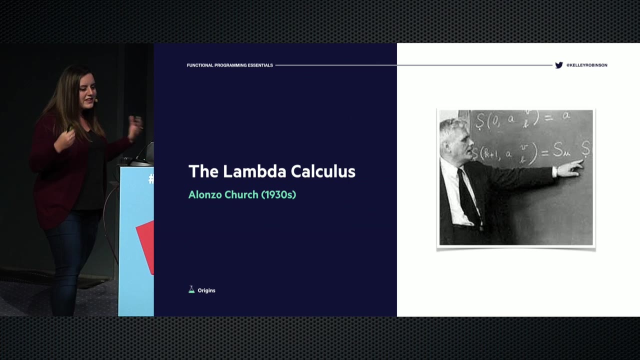 approach. Let's look at some of the history that led us to this approach. Dating back to the 1930s. we can look at the lambda calculus. This is when Alonzo Church, pictured here, introduced this idea of the lambda calculus. And Church was a mathematician, and so what? 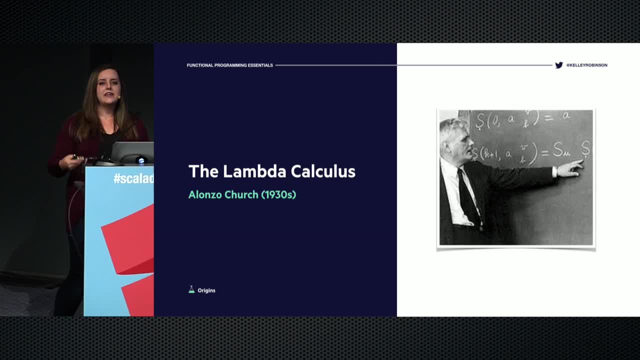 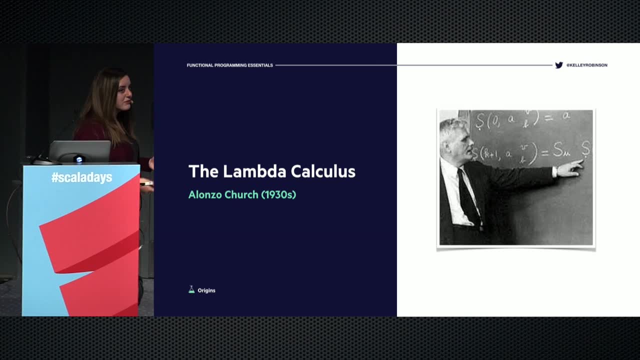 he figured out was a way to represent computation using what we now know as functions, And the lambda calculus is one of those buzzwordy things that might sound a little intimidating. To be honest, I didn't really know what it was until recently, except for that it was. 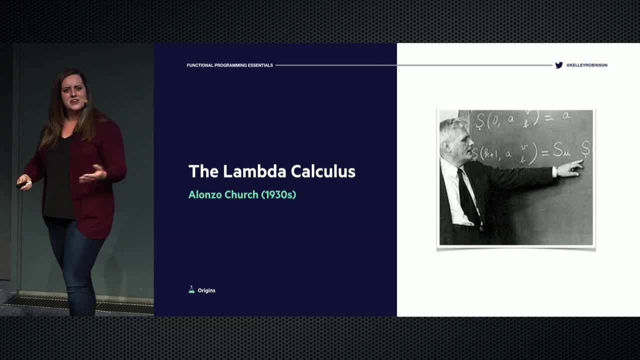 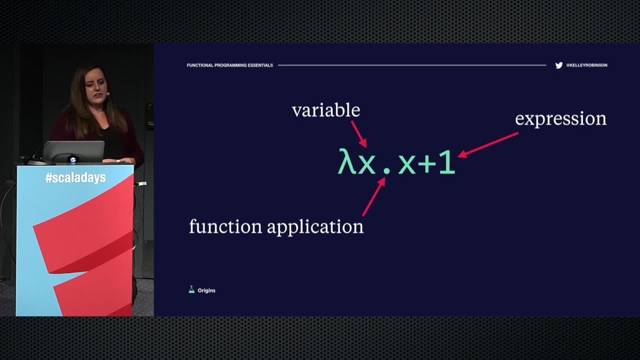 one of those things that we do actually know what it is. We might just not know that it's called that or be able to define it off the fly for someone, But this is the syntax for the lambda calculus, and Church created the syntax to represent his model of computation. 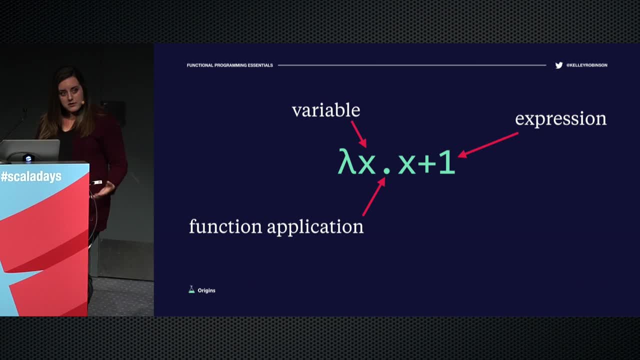 And the lambda calculus has three parts. It uses the notion of variables. it has a way of building functions that take in those variables and a way of applying the function to return a result. In Church's formal definition there are no types. It's the simplest and most basic way. 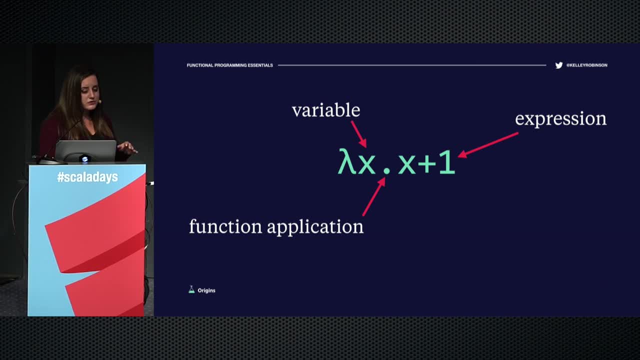 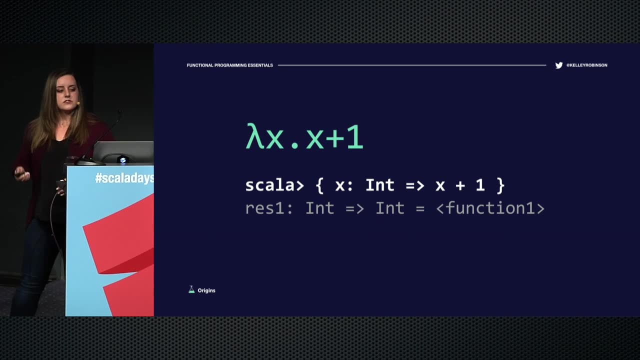 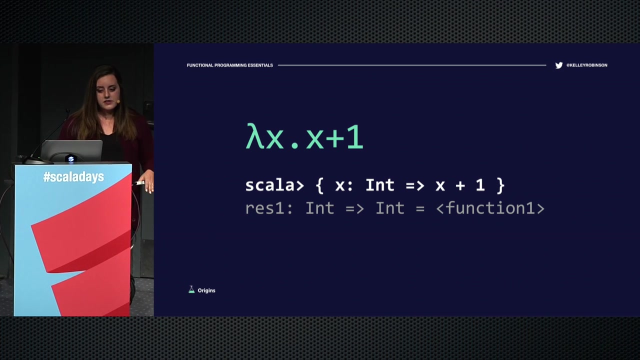 to represent computation that there could be. There's no internal state, all functions are pure and have no side effects. And here that is translated to Scala. The Scala version is a little bit of a red herring because, like I said, there's no types in the lambda calculus, but it's the most simple. 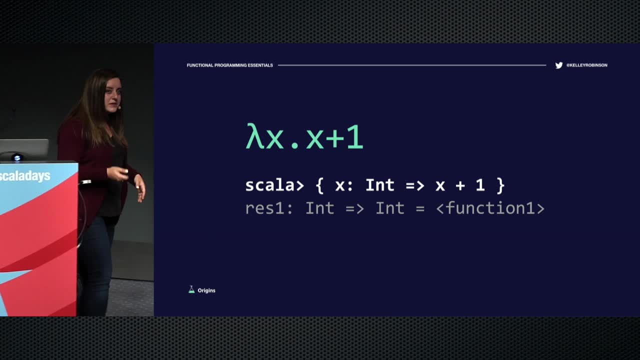 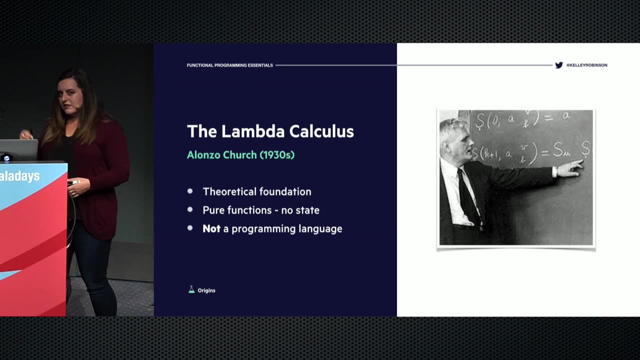 and general definition possible. It also doesn't name its functions, which is why we often associate lambdas with anonymous functions. The lambda calculus could be considered one of the earliest functional programming languages, except for it wasn't a programming language, I guess, because it didn't actually run on any computers. But regardless it's a really 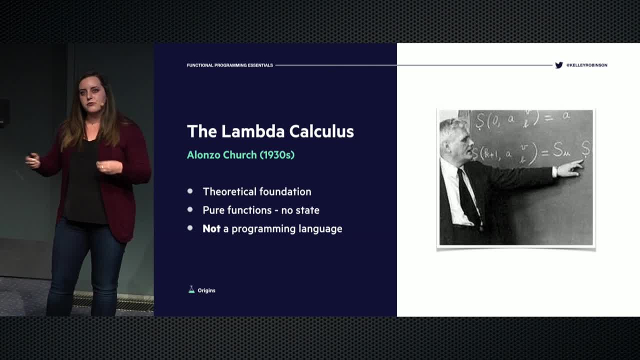 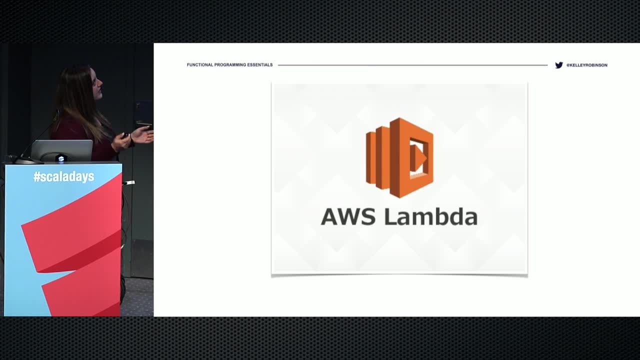 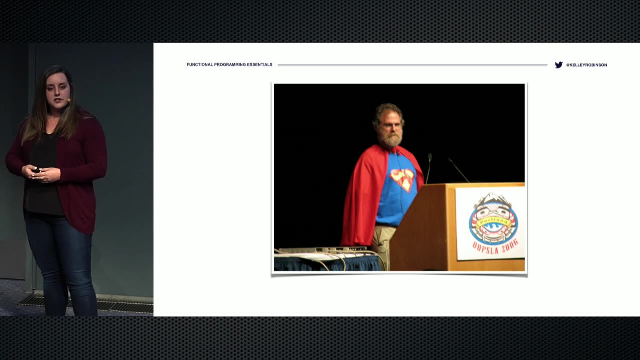 big foundation for theoretical computer science and for the eventual paradigm that we know is functional programming, And it's everywhere now, So from things like AWS lambda, which is basically Amazon's offering for functions as a service, and then here is Philip Wadler, who is a functional 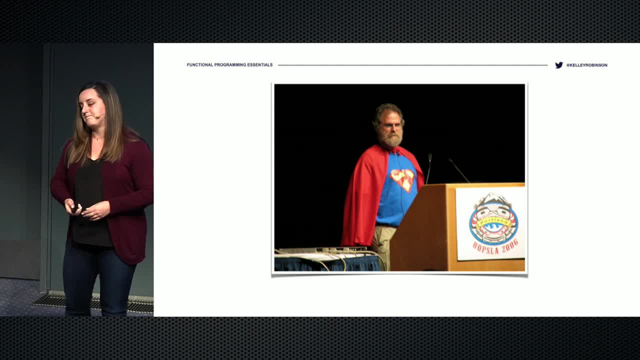 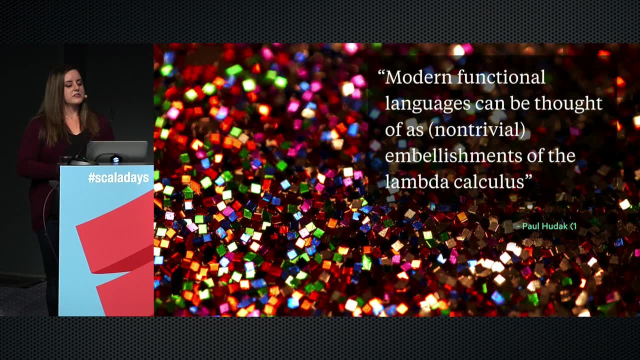 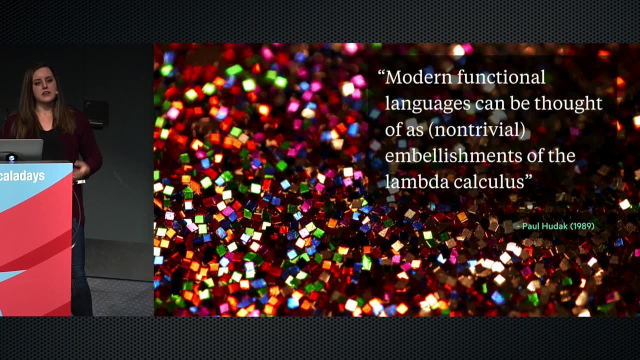 programming researcher and he is dressed as Lambda Man. Another computer science researcher later said that modern functional languages could all be thought of as non-trivial embellishments of the lambda calculus, And I think he would be right, because, at the core of it, when we think about the languages, 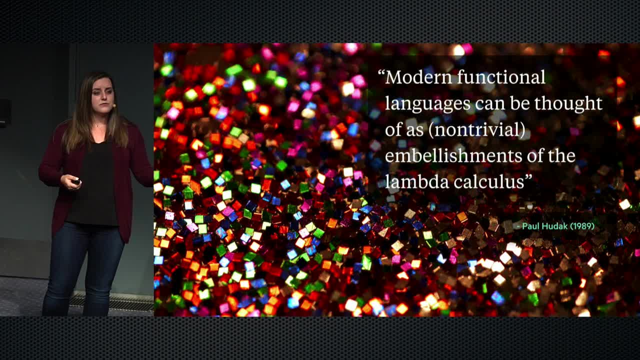 we use today, whether they're languages that we think of as using for functional programming or not. most of our modern languages have this idea of functions as a core abstraction to the language, And that's why Church's contribution of the lambda calculus matters. So, Church, 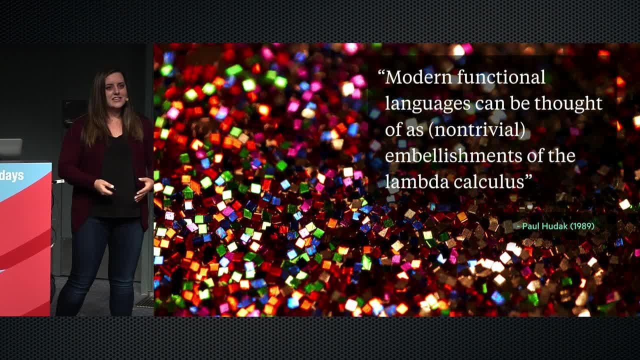 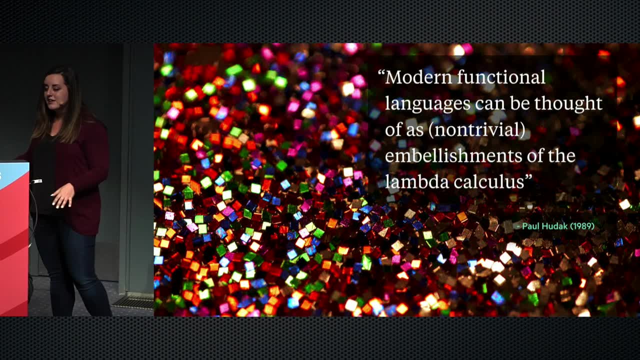 introduces this lambda calculus. but he's a mathematician so it was kind of intense. In his mind everything could be represented as a function, so he was even representing things like Booleans using functions. functions, and that's fine. but again, this wasn't a programming language. so when we 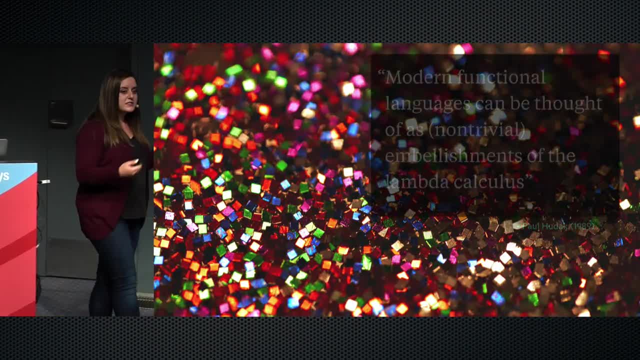 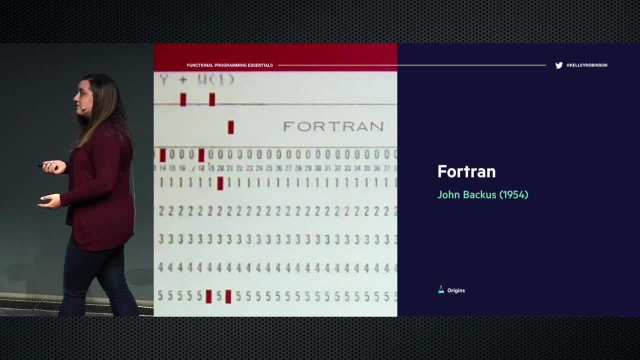 talk about introducing some of these concepts into actual programming languages. it might surprise you to learn that some of the first programming language use of functional programming was written in Fortran, So Fortran is also known as formula translator- that's where the name comes from and this 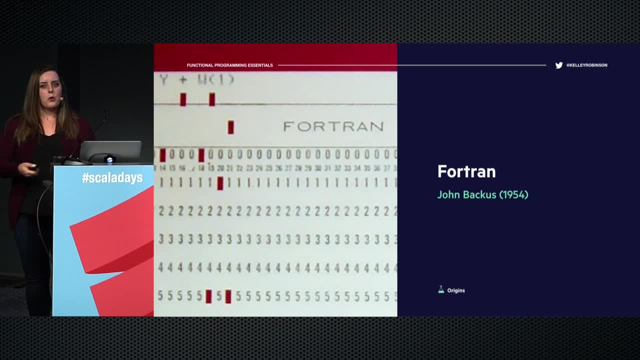 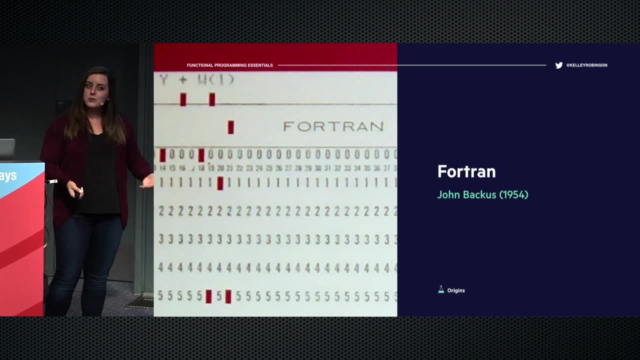 was invented by John Backus in the 1950s and there were a few important developments that came with Fortran, So it was popularised as a higher-level language. Before then most people were writing in assembly. so very procedural: do this and then that. 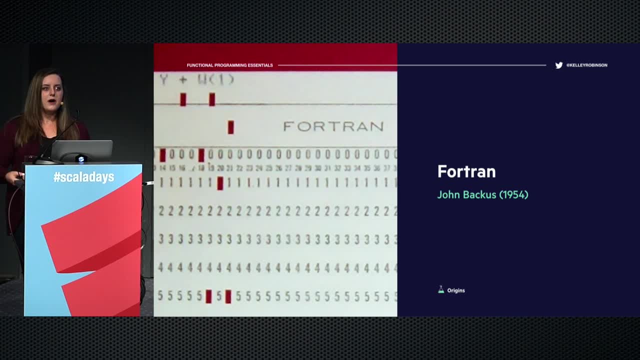 there wasn't a lot of abstraction that was happening, so Fortran became popular as that first higher-level language that provided some of these abstractions that we now take for granted. It's really hard to think about things like functions when you're programming in something. 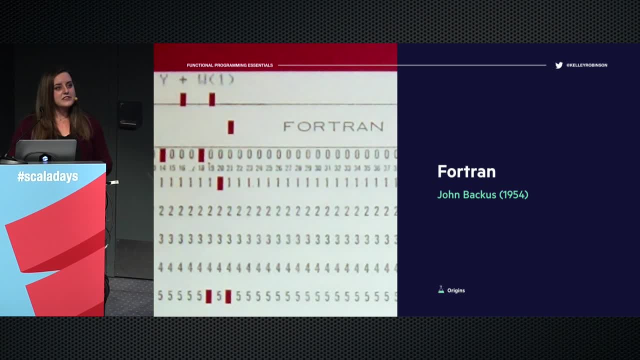 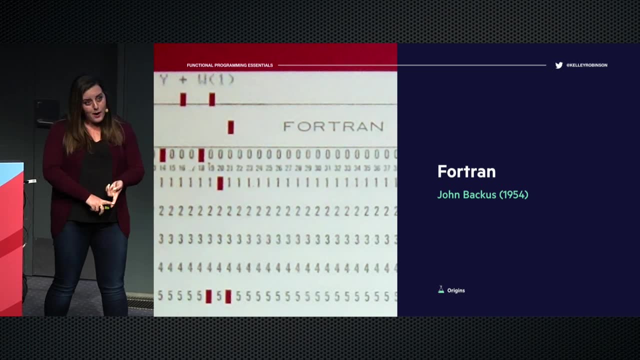 like assembly, you can't really do it. and some of the other things that Fortran allowed us was were introduced to for this paradigm were things like: it allowed mathematical operators inside of your syntax, so things like plus and minus were now possible, and it also allowed the nesting of function. 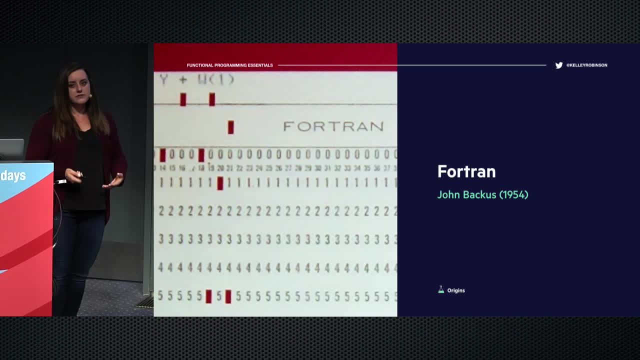 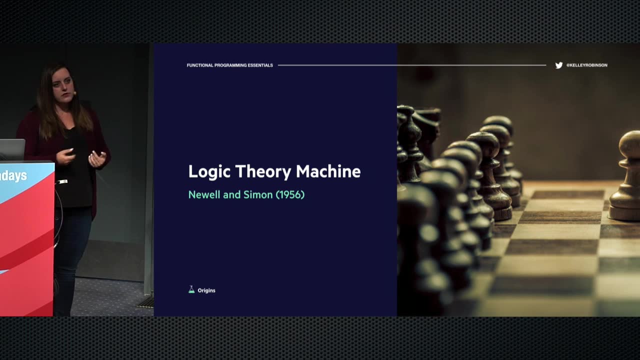 calls something we take for granted now again, but it was a big development at the time. Around the same time, a couple of other researchers were trying to invent some of the first AI programs, and so Alan Newell and Herbert Simon were trying to write a chess game. and what? 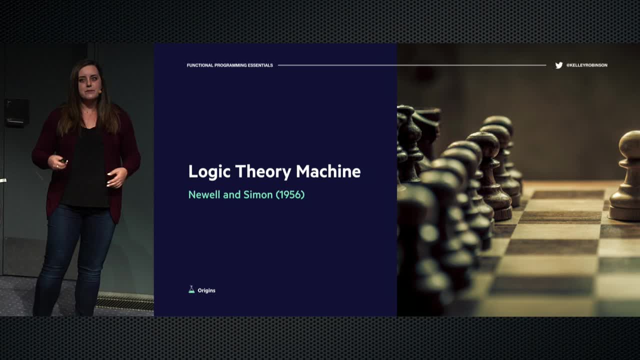 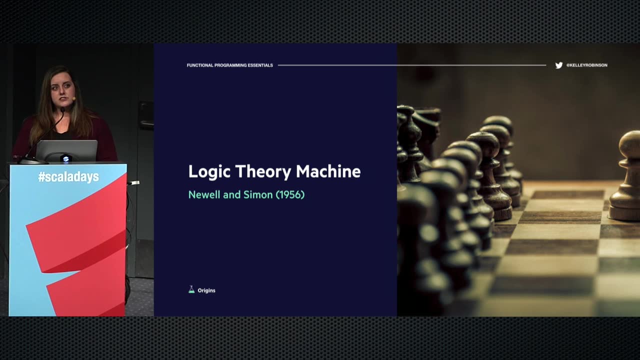 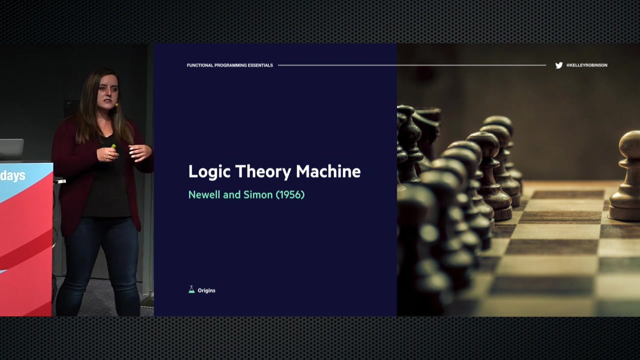 they figured out was in order to represent something like a chess game. they needed a new way to program and represent their logic, and they invented something called the logic theory machine to do this, and that worked by writing and combining many small and simple subroutines into larger and more complicated problems. 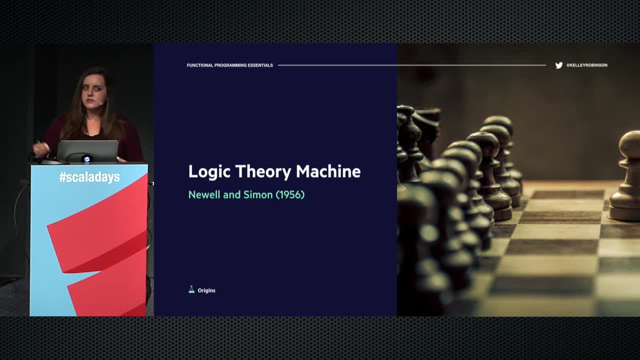 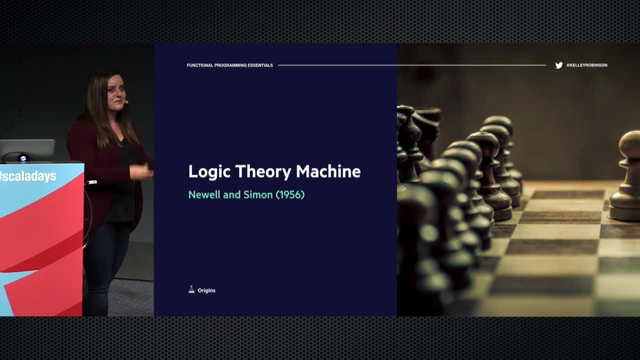 Before this point everyone else was saying that a program was a sequence of instructions and there weren't these kinds of abstractions. This was a time that it wasn't previously possible to just combine a bunch of simple subroutines. Combining subroutines takes a lot of processing power and in the 1950s the hardware was 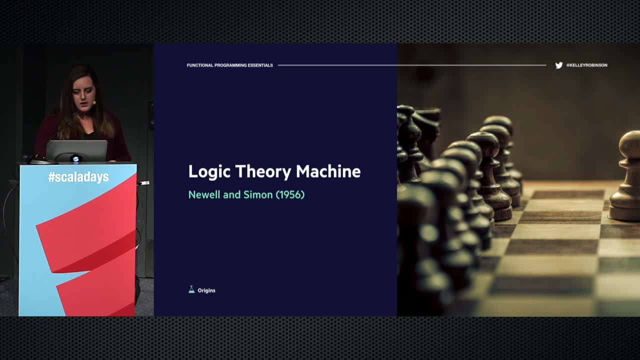 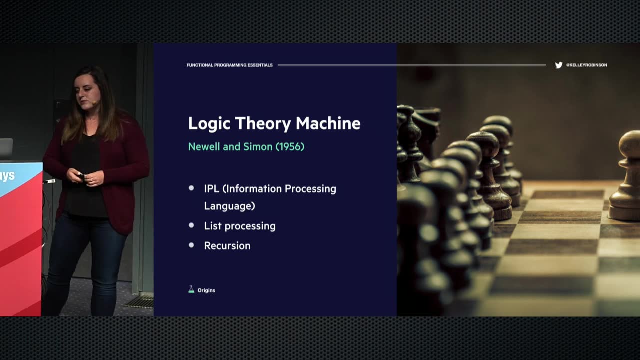 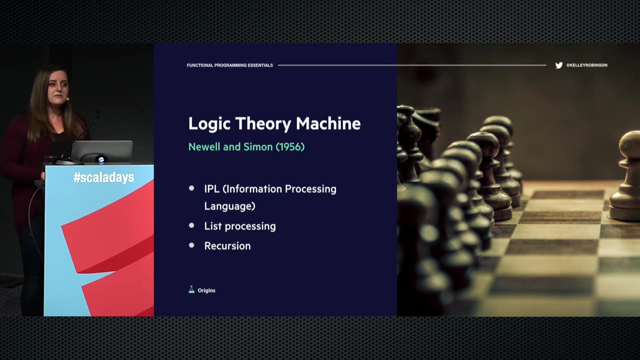 catching up to make this plausible and feasible. So Newell and Simon gave us something else with their research. What they realized was that, in order to process data using those subroutines, they had to find a way to store the data, and so they essentially invented what we now know as linked 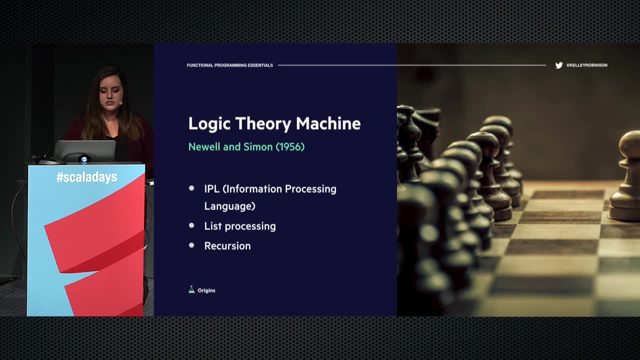 lists And they brought us list processing with this data structure invention. So they invented the IPL, the information processing language, and the IPL was able to do this list processing that we now use so often in many of the functional programming languages that we think of today. 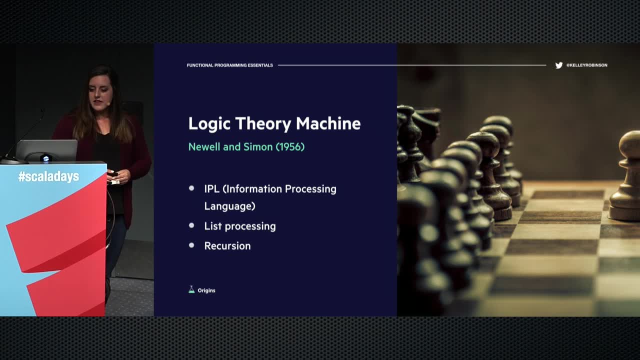 The data was stored, like I said, in what we think of as linked lists, and that allowed them to do list manipulation even in a very limited way, but it was a really big innovation for the time. IPL also introduced more data. 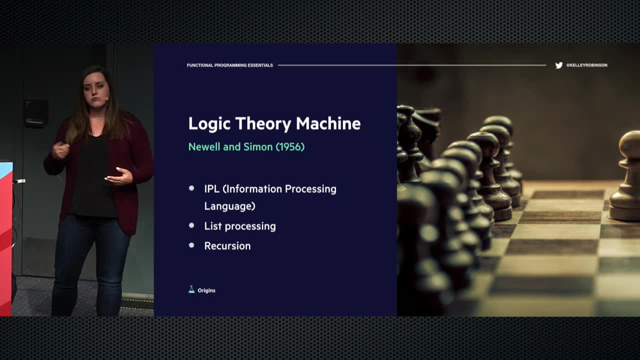 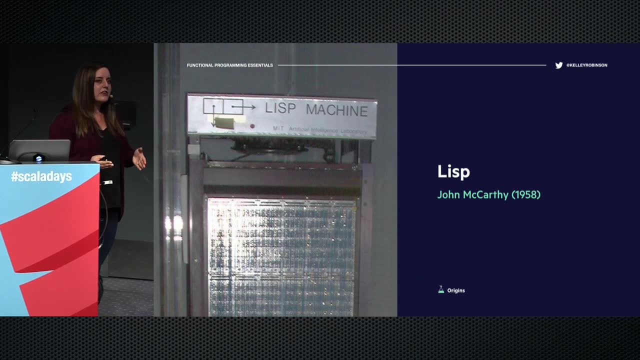 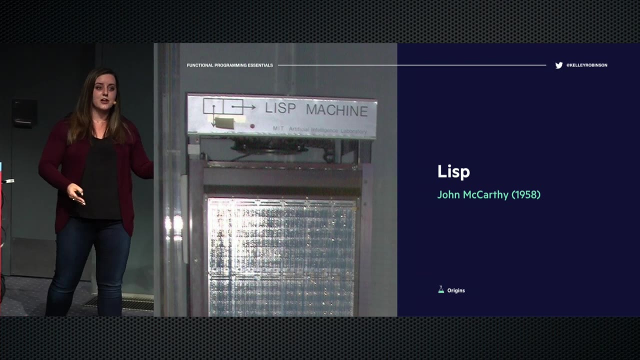 It was able to do more general, higher-order functions, which is something that enabled recursion. What happened next was Newell and Simon went to this AI conference with their friend John McCarthy, and McCarthy was already doing some stuff in the functional programming space. He had added some stuff to Fortran, some conditional operators to Fortran, and he was already actively. 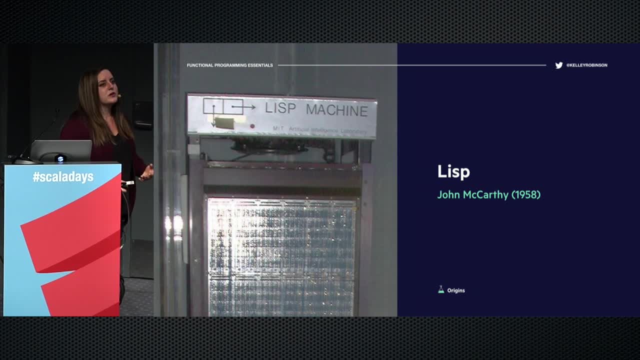 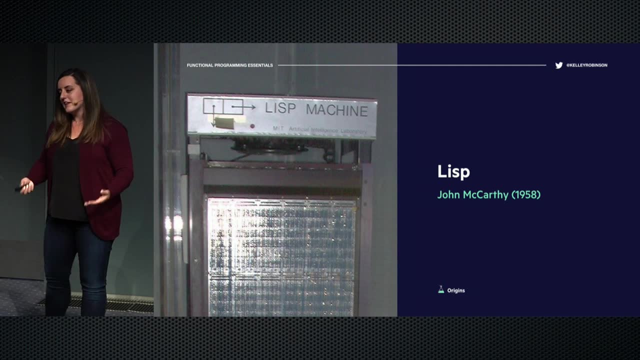 involved in the development of this paradigm. But McCarthy was listening to what Newell and Simon had been doing and said, hey, those sound like pretty good ideas. I'm going to take those and build them into my new language that he named Lisp. 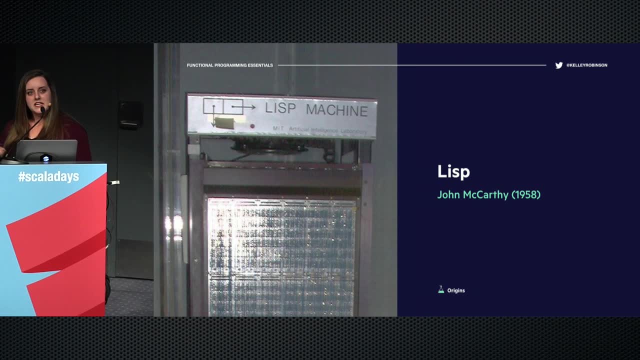 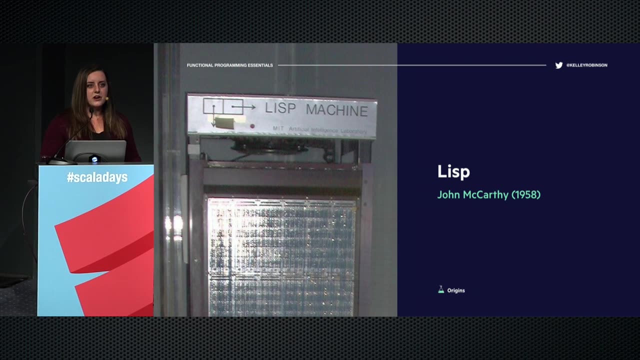 And Lisp is widely recognized as the first mainstream functional programming language, the first general-purpose functional programming language, and it took many of the ideas that we already discussed and put them into one package that made it easy to use as the programmer. It enabled the programmer to write in this functional style. 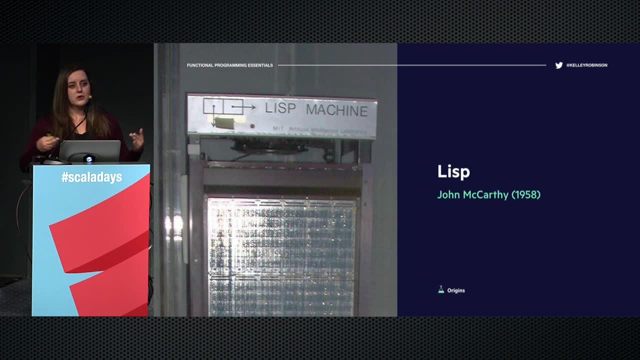 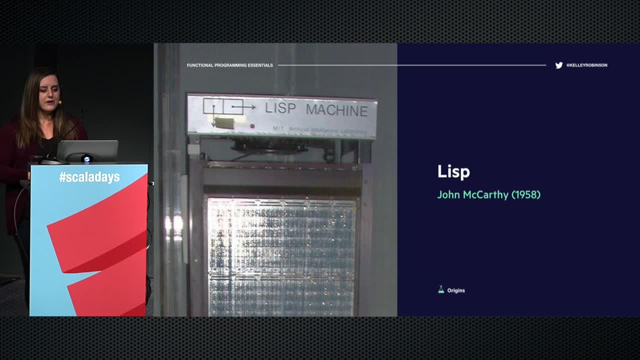 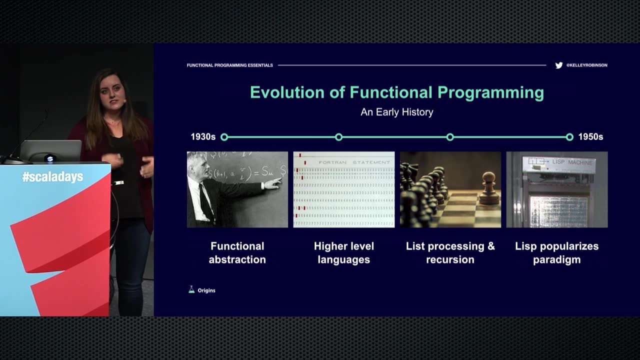 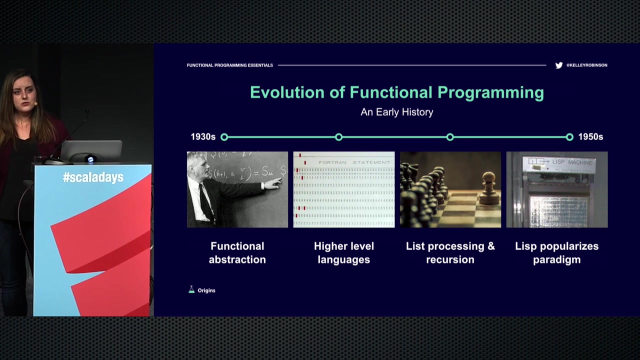 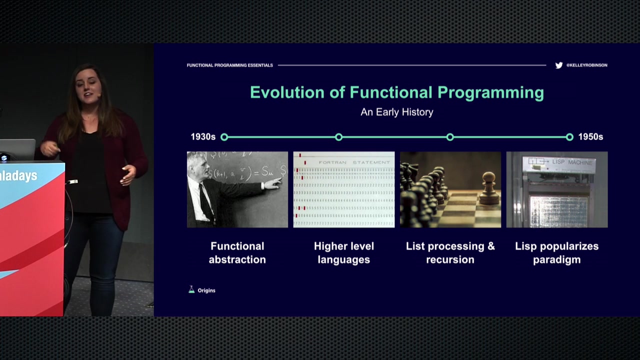 of these styles and really encapsulated this functional programming paradigm. Bringing all together this history that we mentioned, you can see how these concepts evolved into something that we recognise today, And this history matters because it shaped functional programming into what we now know- These concepts. so things as obscure as the logic theory machine may be or as dated as 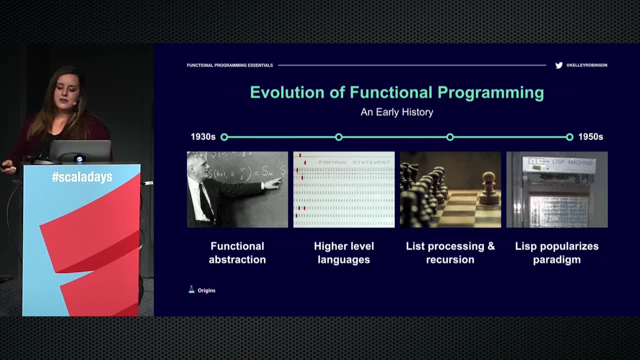 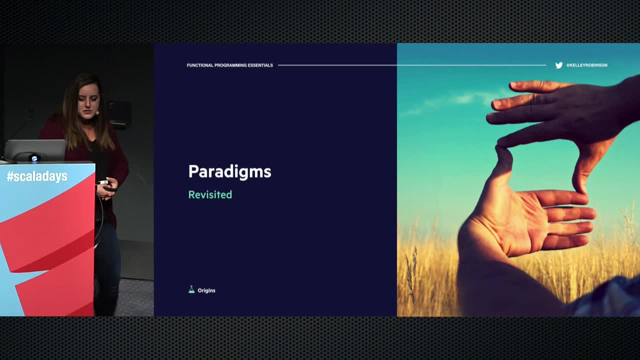 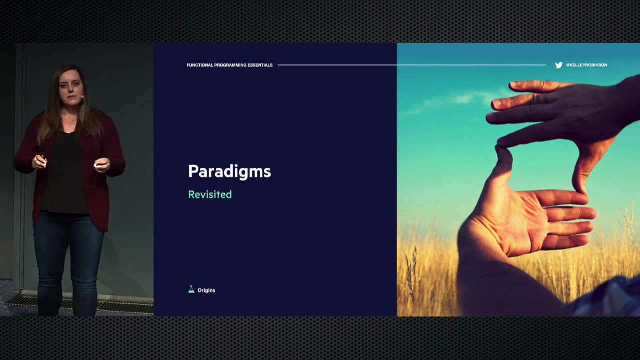 Fortran may seem. these concepts matter because they defined the paradigm as we know it. Now you have a pretty good idea of where some of this stuff came from. One thing I wanted to highlight is that in doing this, in inventing this new paradigm, 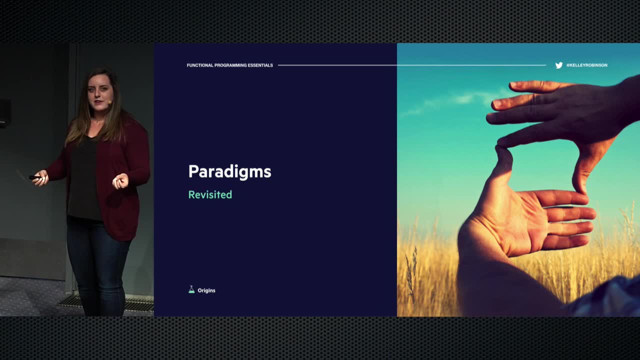 these researchers weren't trying to invent a paradigm. They did this, Or they discovered this paradigm. They did this, Or they discovered this new style of programming because they were trying to solve problems and they needed a new style, a new way to do things in order to make their operations. 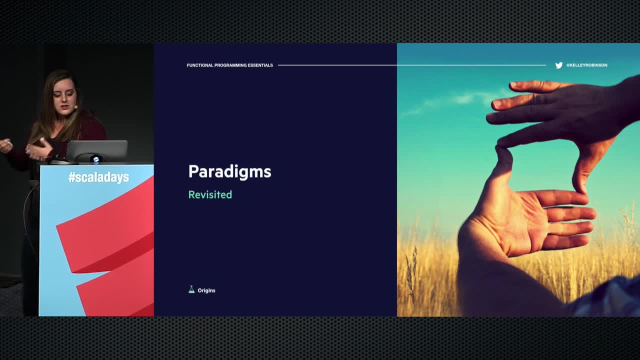 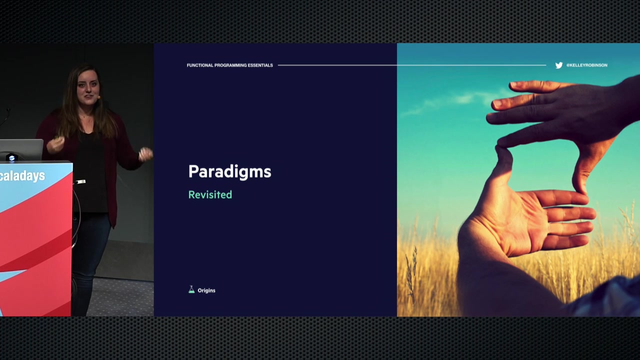 and their problem make sense and work, And much of that had to do with making programming easier and more understandable to the programmer, And I think that's a huge tenet of what functional programming is. From its very beginning, functional programming was about making programming more understandable. 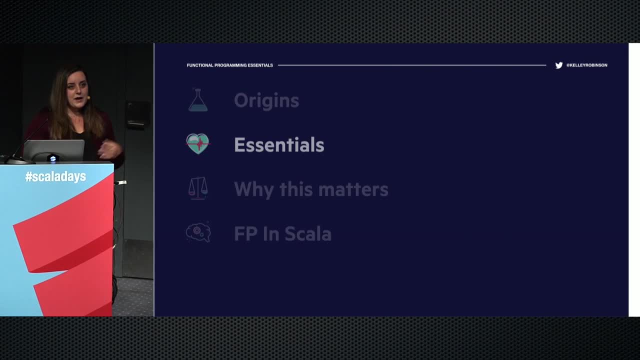 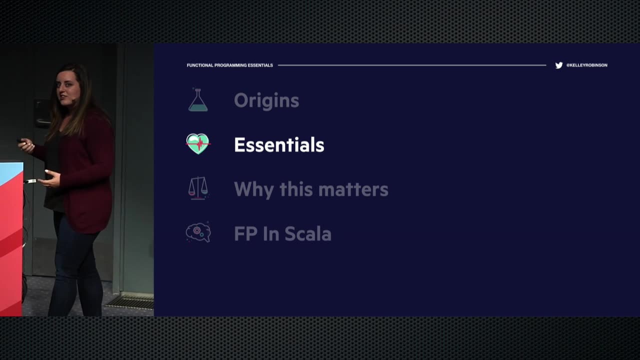 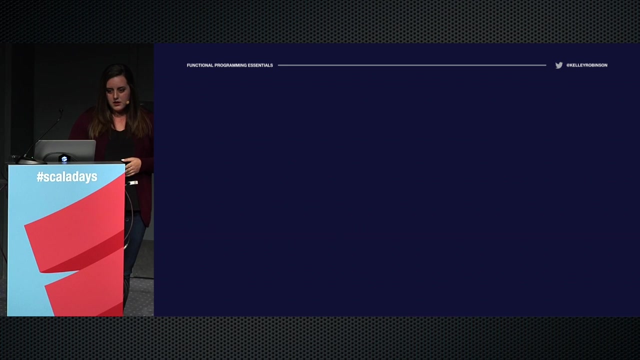 to the user. And that brings us to the essentials, and this is where I'm going to define what I want to talk about as the definition of functional programming. What are the essentials of functional programming And why that style that was formed plays into this. 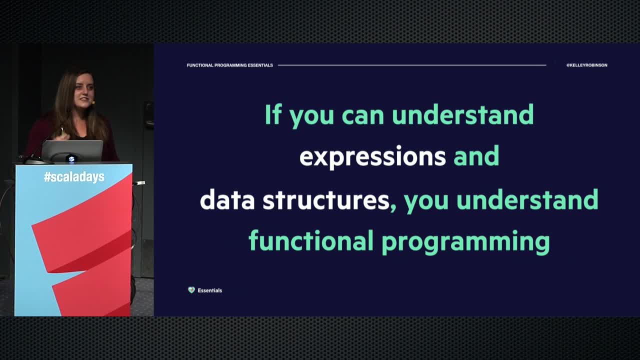 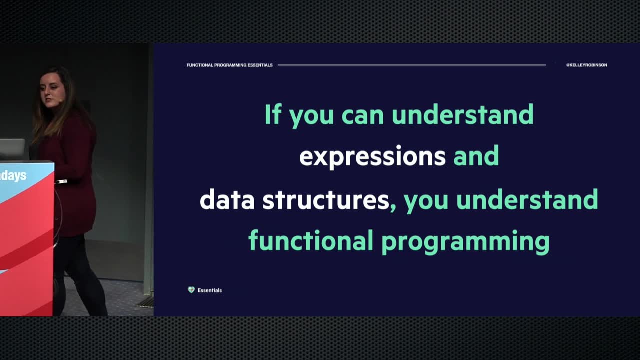 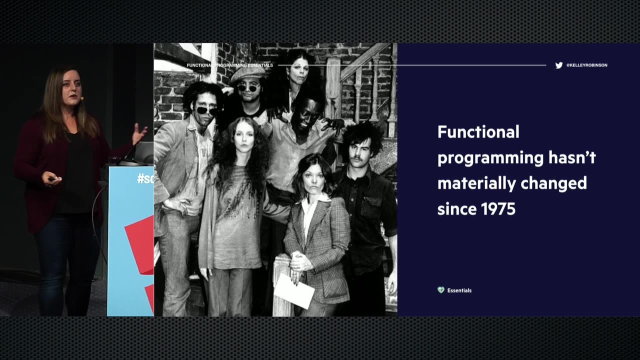 Don't want to bury the lead here. If you can understand expressions and data structures, you can understand functional programming. These are the two key components of functional programming: Expressions and data structures. Okay, And when we talk about this idea of contemporary functional programming, I'm going to talk. 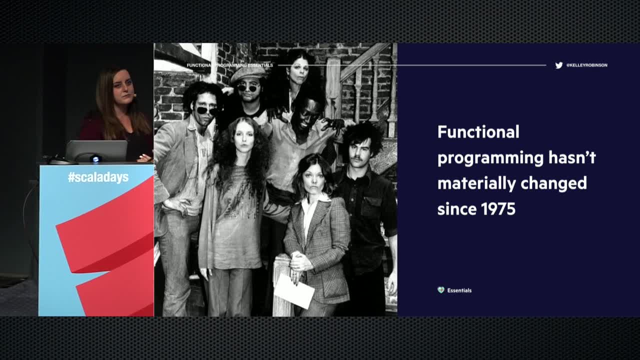 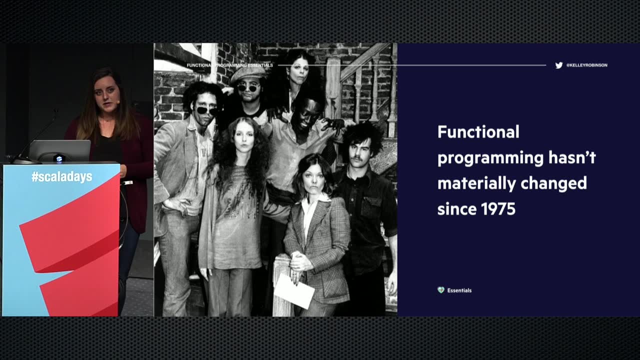 about it from the lens of 1975, and I'll mention why that date's important on the next slide. But for those of you that don't know, 1975 was also the year that Saturday Night Live premiered, so that was the best picture I could come up with from there. 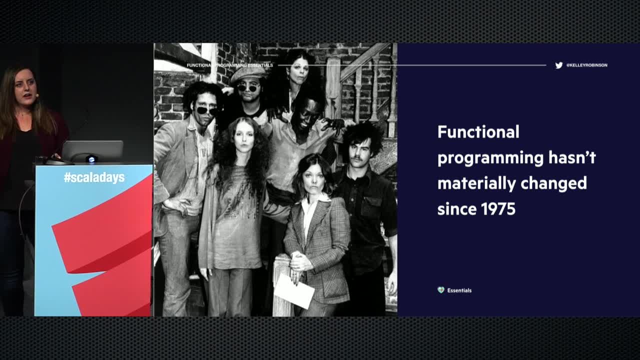 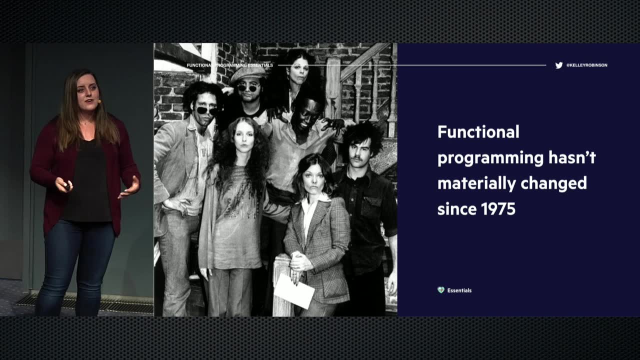 But this is a bit of an arbitrary date. but I wanted to bring things more into the modern era but also show you that functional programming it's not that different than it was in the 70s. A lot of the core concepts, The ideas of expressions and data structures haven't changed since then. 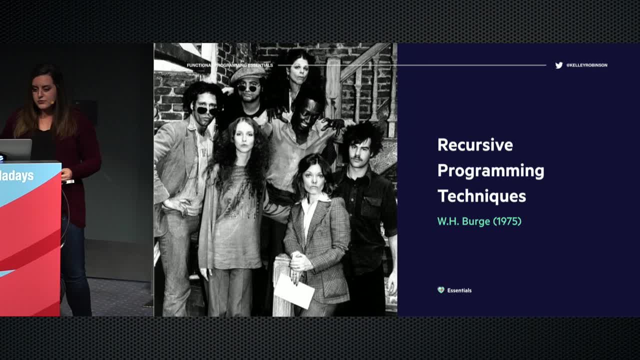 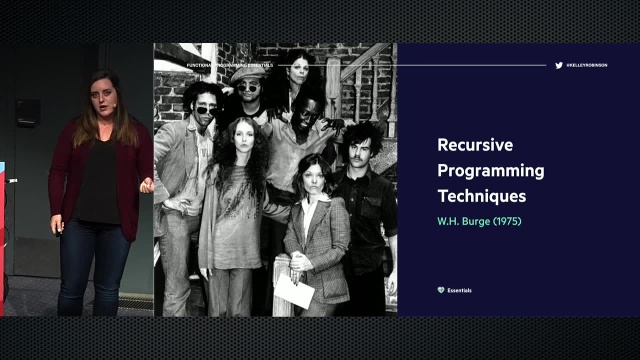 So Jose Calderon, who I mentioned earlier. he's writing a great series of blog posts distilling the work of William H Burge, And Burge published this book Recursive Programming Techniques in 1975, and a lot of the concepts. 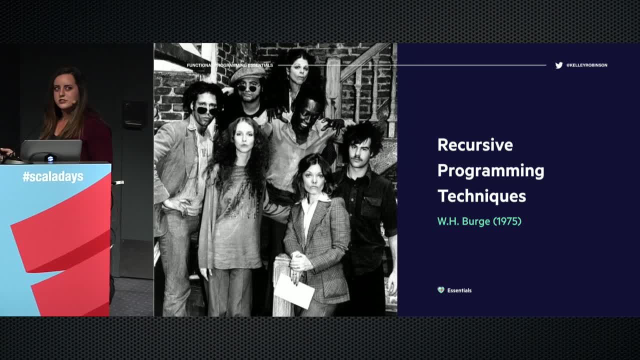 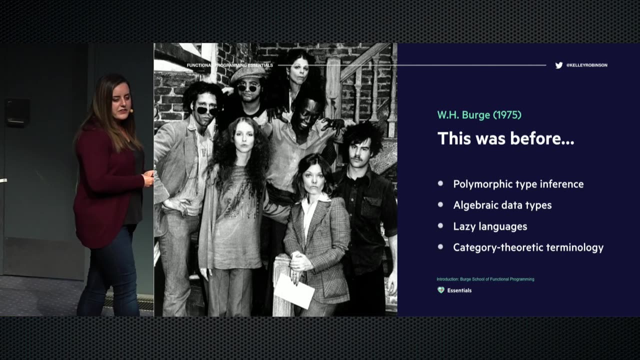 that he talks about, about defining functional programming. they haven't changed to this date, Especially because in 1975, we didn't have a lot of the fancy abstractions. So just for an example, things we didn't have, we didn't have polymorphic type inference. 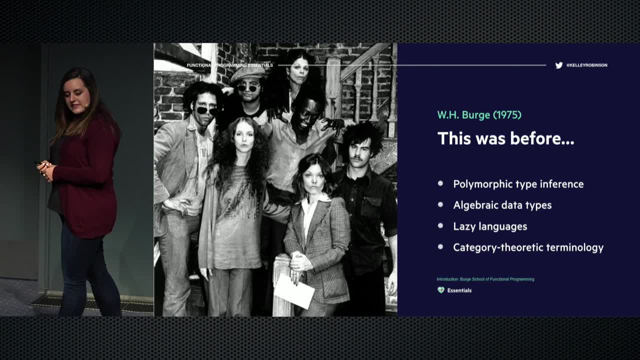 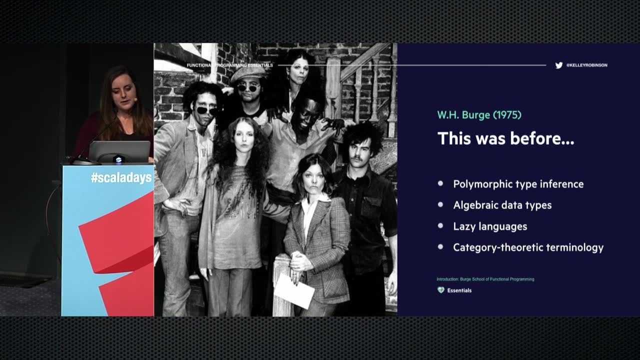 we didn't have algebraic data types, we didn't have lazy languages, so those came soon after and we definitely didn't have a lot of this category-theoretic terminology being applied to programming. It's okay if you don't know what half of those are. 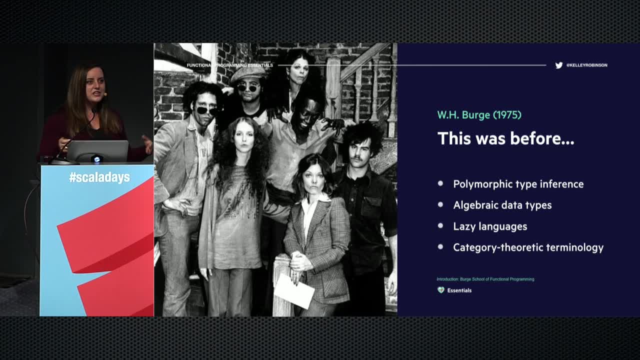 I'll show you the essentials and how knowing the essentials will give you the tools and the power to be able to do what you need to do in your program. And now we'll talk about what we do have the fundamentals that Burge mentioned in 1975. 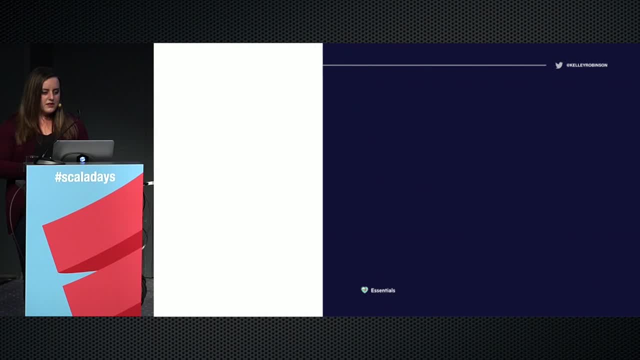 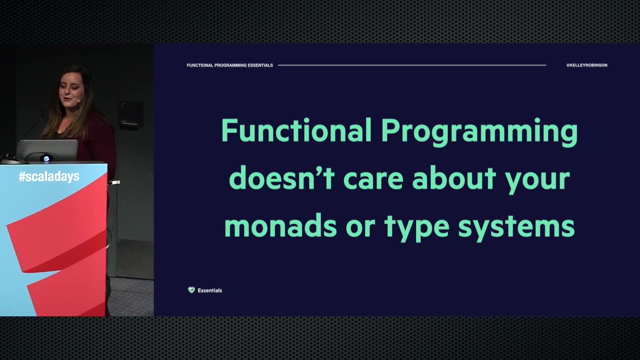 in order to define this paradigm. First of all, functional programming. it doesn't care about your type system. it doesn't care about monads. This is not what functional programming is about, And the whole motivation for this talk was to clarify that. you don't need to understand. 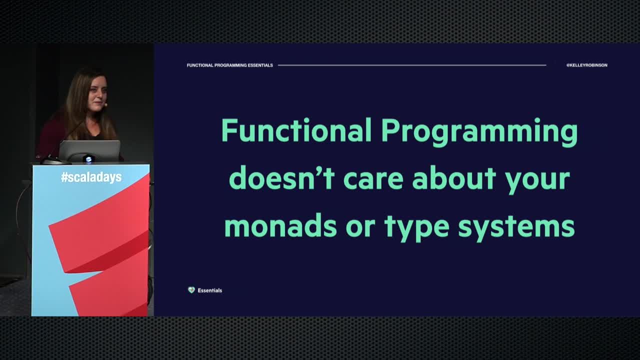 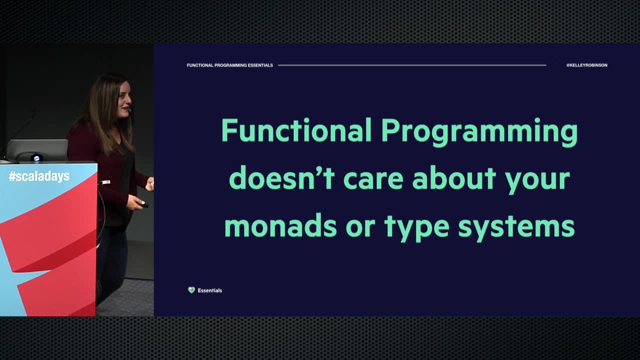 or know these things or be able to use this in your day-to-day programming, in order to be a competent functional programmer. Thank you. You don't need to be able to define these and be the person that's talking about this all the time in order to be a competent functional programmer. 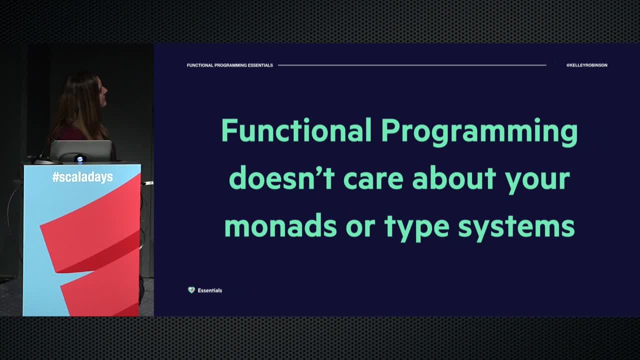 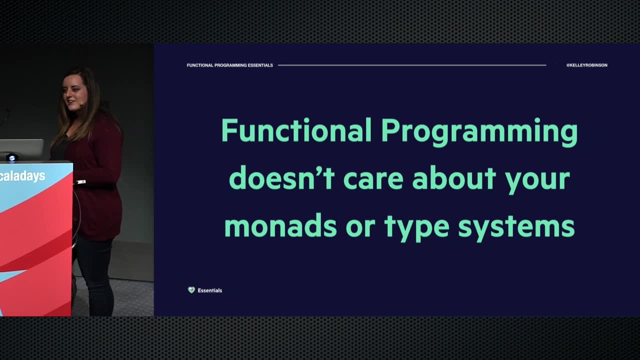 And you can replace monads and type systems here with whatever jargon you want. I think-what's the one I've been hearing about a lot at this conference: What is it tagless final-what is it Tagless final interpreters. 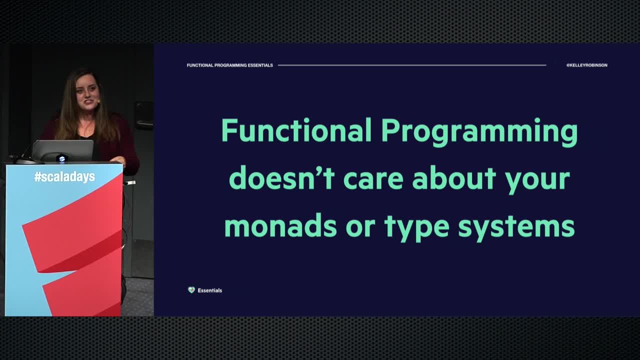 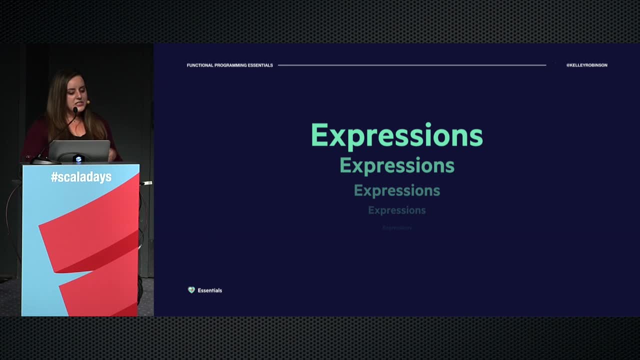 I don't know what that is, but it's not essential to functional programming. Functional programming is about expressions and data structures. Start with expressions. We talk about the essentials. Functional programming is all about representing your programs, the logic of your programs. 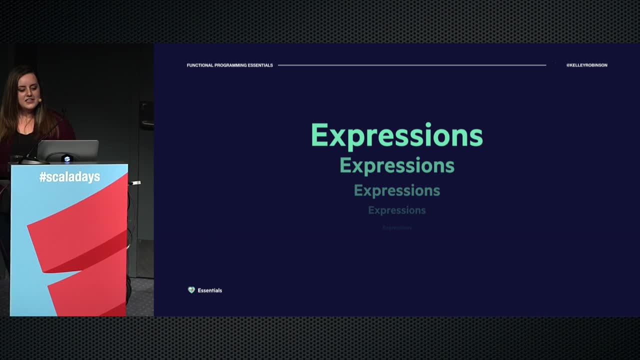 using expressions instead of statements, And the concepts and the skills that we think of as being functional programming, abstractions, those all have roots in expressions, This idea of expressions. it's expressions all the way down. What do we mean when we talk about expressions? 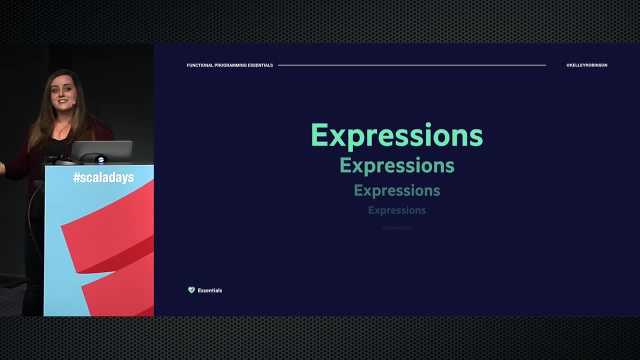 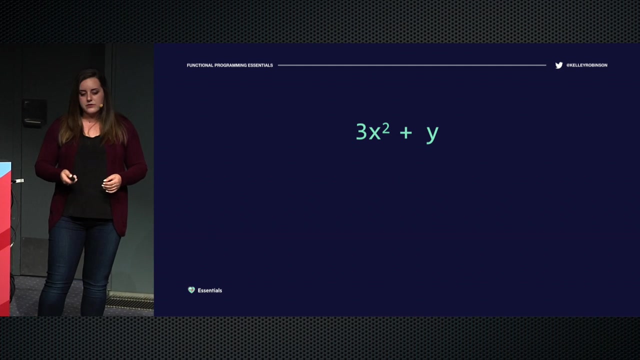 Well, it helps to think about expressions in terms of their constituent parts, And this allows you, the programmer, to isolate the different parts of your program and break things down so that they're more understandable. Here's a simple expression. We can more easily break this down if we represent it using infix notation. 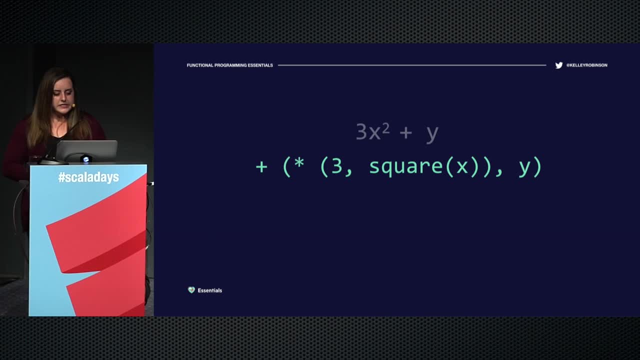 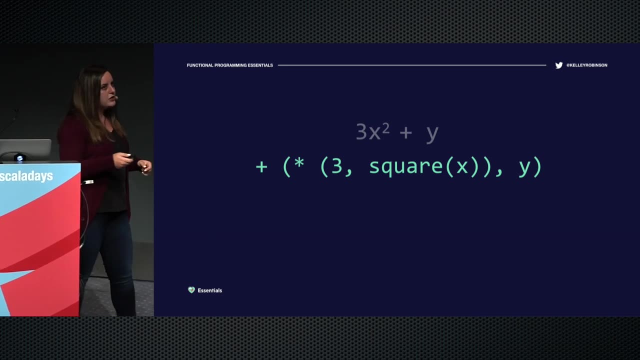 A little bit of middle school algebra for you here today. So here are the operators. Okay, So backing up a little bit, Burge emphasizes that you can break things down more easily by stressing the difference between the operator and the operand in your programs, and those are part of the isolation. 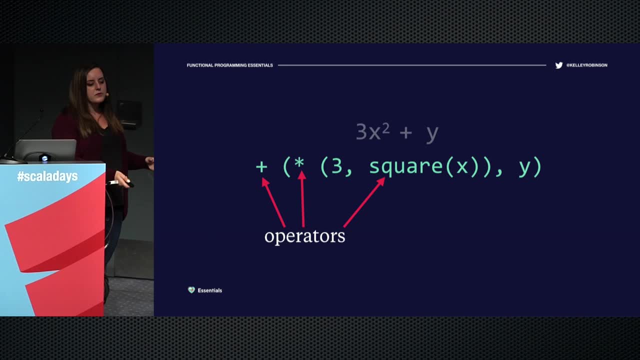 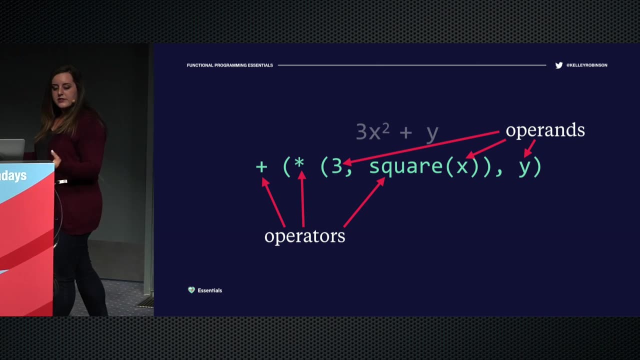 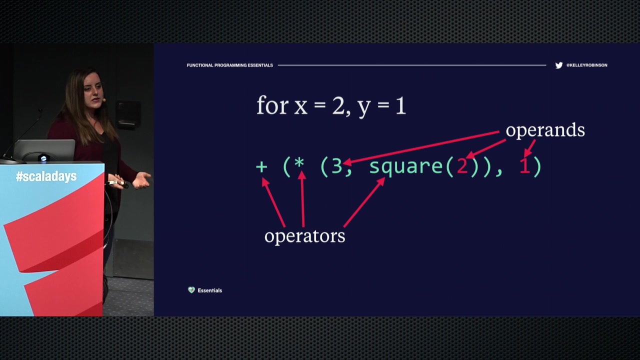 that we do in order to represent the computation, And here the operators are the plus, the times and the square, while the operands are the things that we're operating on, are the 3, the x and the y. If we give x and y values, we can look at how this expression is broken down into smaller. 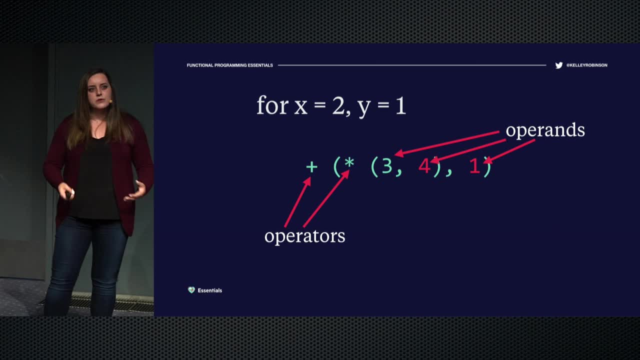 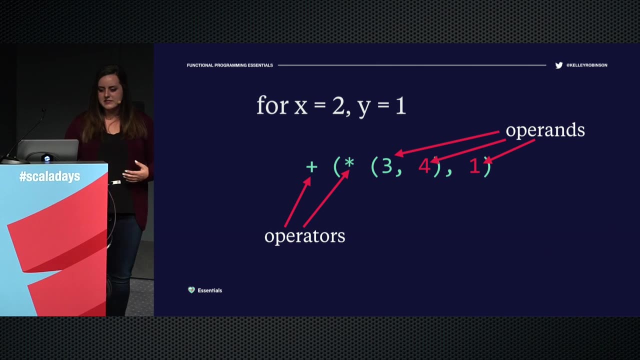 parts, And I hope your work isn't basic algebra, but this is the example to illustrate how we use expressions in our programs to isolate and break our code into smaller and more manageable pieces. This shows one of the tenets of functional programming that's essential to this idea. 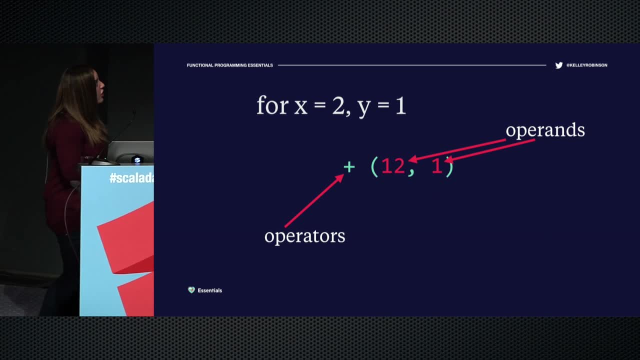 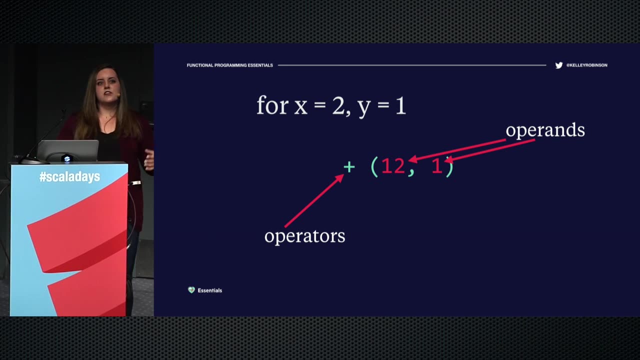 of using expressions. Functional programming encourages us to build bigger programs out of smaller parts and those parts that we can understand in isolation, And we do this in part by separating concerns, and that helps us build understanding. And you can see how we evaluated everything, piece by piece, in order to achieve our final 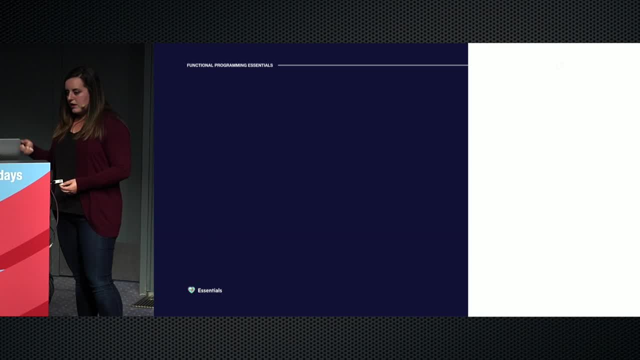 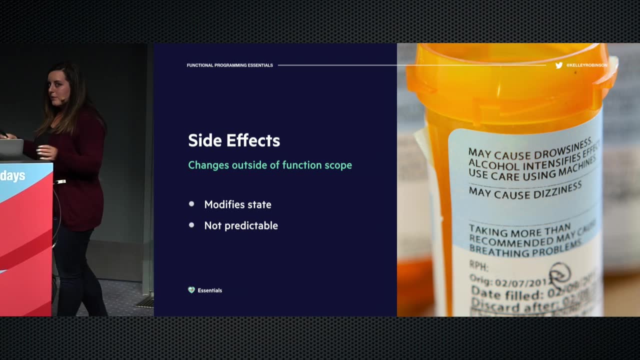 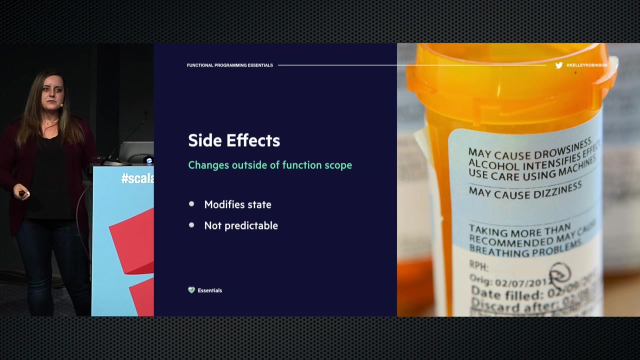 result. I wanted to quickly talk about side effects, because this is something that comes hand in hand when you talk about expressions, A reminder that side effects are not inherently bad. There are side effects that are necessary- things like logging- But they do have some downsides. First of all, the fact that we have a lot of storage, We have a lot of storage. First of all, we have a lot of storage, We have a lot of storage. And the second one is that we have our time and space. 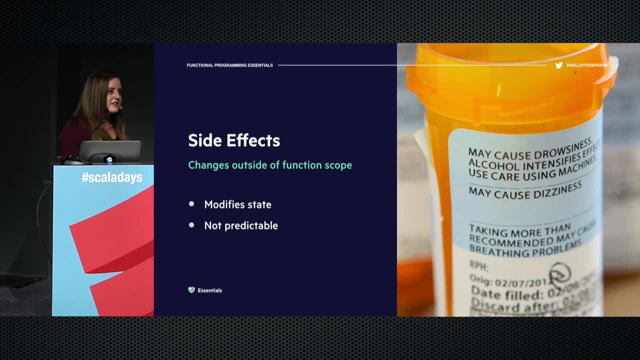 So it's a very important moment when we're talking about does is that you can reduce the time in the process, And we do this in part by separating and separating concerns, And that helps us build understanding. You want to program without side effects as much as possible in this style, because side effects aren't as predictable and they come with some. they can complicate things in certain ways. 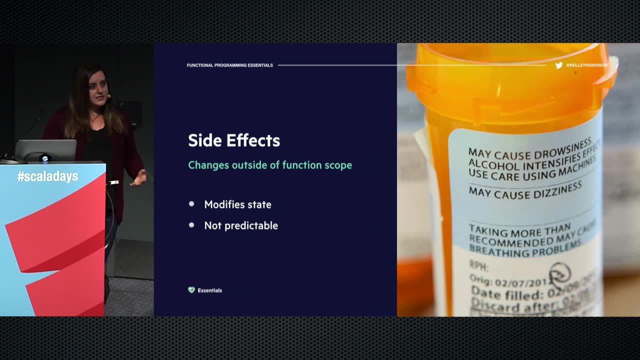 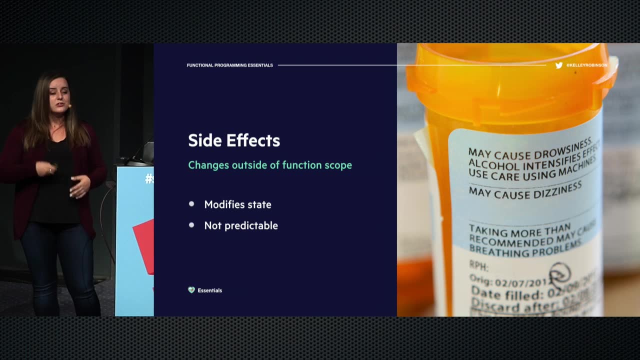 And we say a function is side effecting if it modifies state outside of its scope. so things like changing a global variable. every time you're doing a for loop in an imperative style language, doing that I++, you're modifying state. that's a side effect. 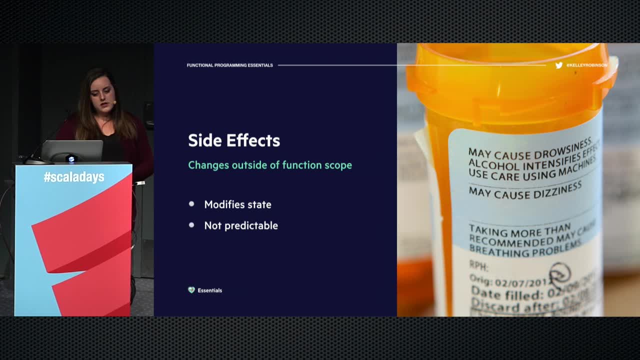 This is something that we see all the time in those types of languages. Side effects also occur when you're dealing with the world outside of your program. so any time you make an API request or print to the console, that's also a side effect. 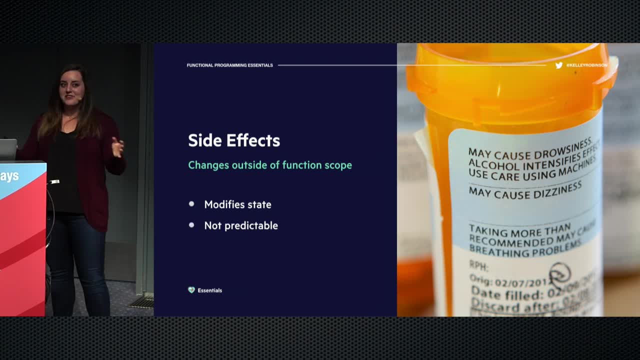 And this approach can be fragile. it's not as predictable. but again, you need side effects to do anything useful in your programs. You're going to have to interact with the user at some point or your program's not going to be very interesting or helpful to anyone. 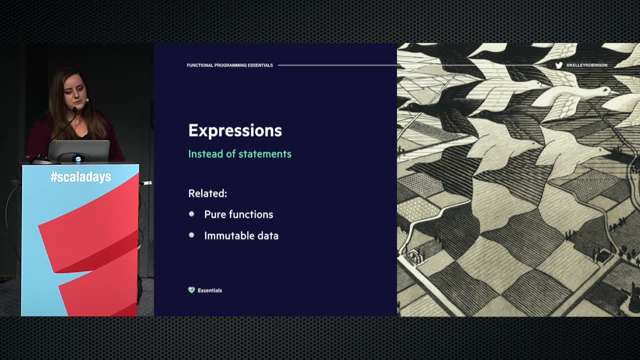 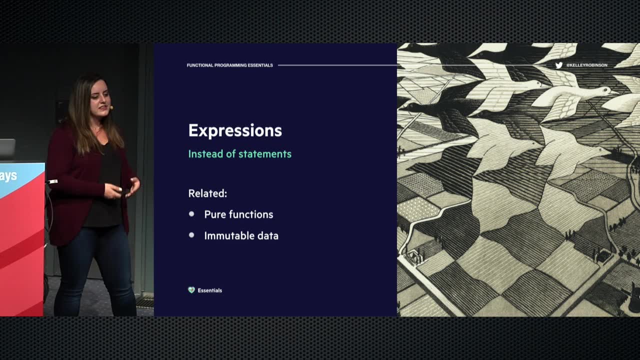 So it's a little bit about what side effects are. Now taking this back to expressions: We want to. We want to use expressions instead of statements and some related properties of expressions that we think about are these ideas of pure functions and of immutable data. 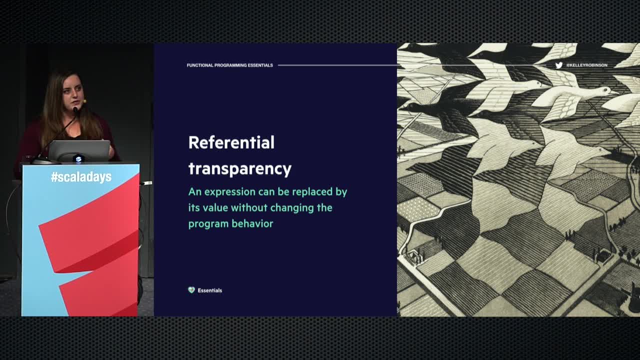 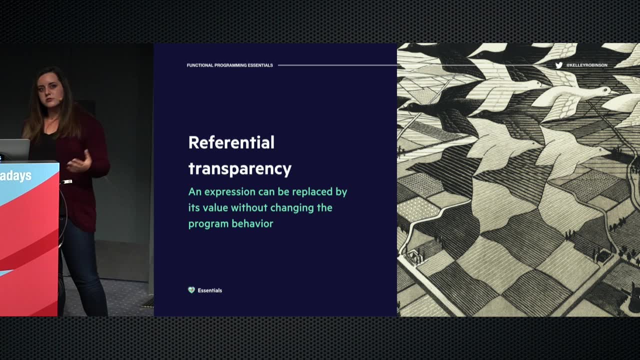 And when an expression has no side effects, we call it pure, and a pure function is also said to have this idea of referential transparency. Referential transparency is the idea that you can replace your expression by its value. so in the expression that we showed, we can replace 3x plus y with the values. 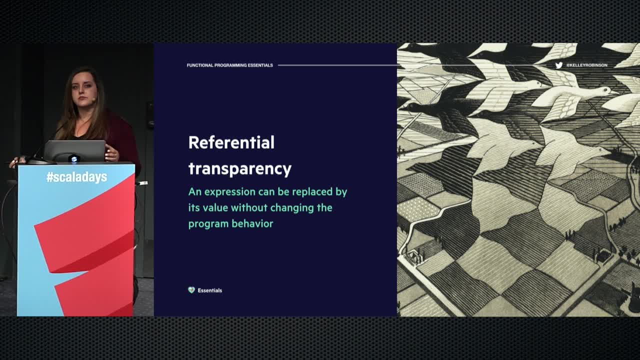 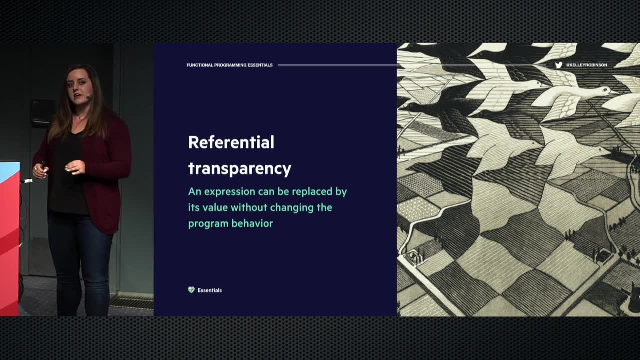 that we gave first. That's what referential transparency means. There's no side effects in there. We weren't expecting it to print anything out to make any other calls to tell somebody to do something. It's exactly the same as replacing the expression with the value. 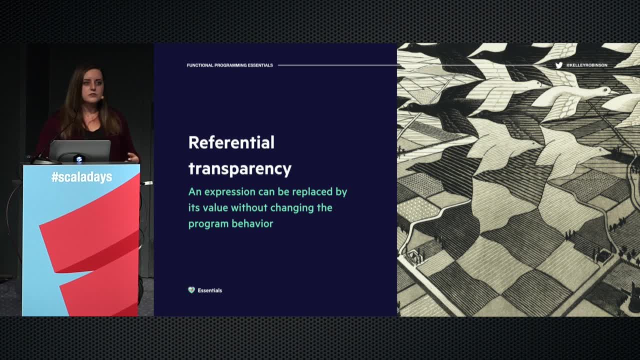 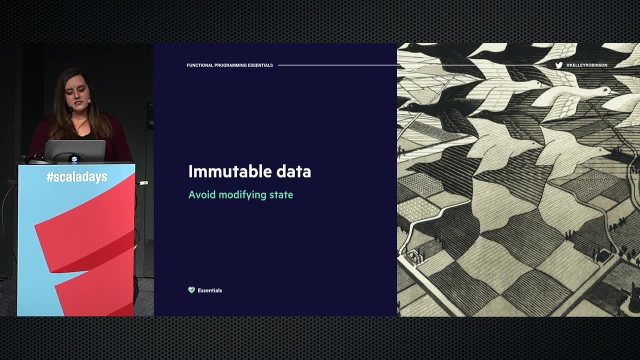 That's what referential transparency means, And this makes it easier to reason about the behavior of our programs. Immutable data is also a huge bonus for expressions. If we were modifying state constantly, we would lose a lot of the benefits that we talked about. 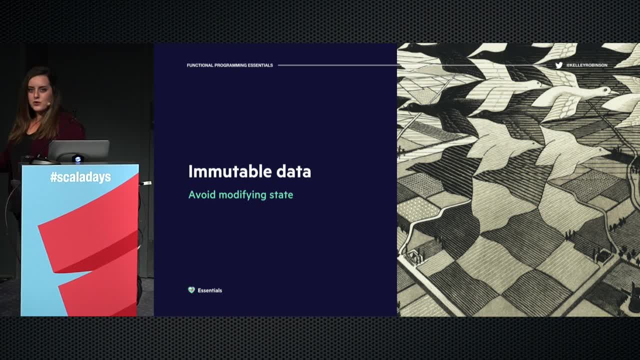 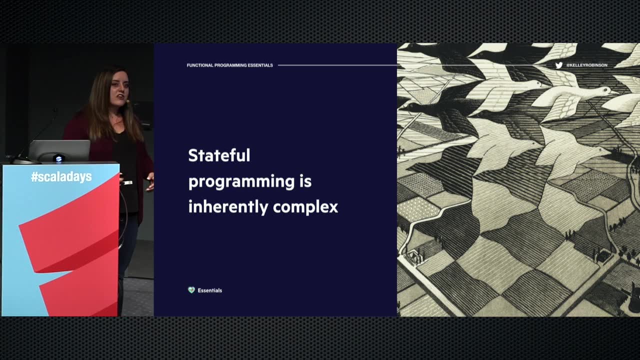 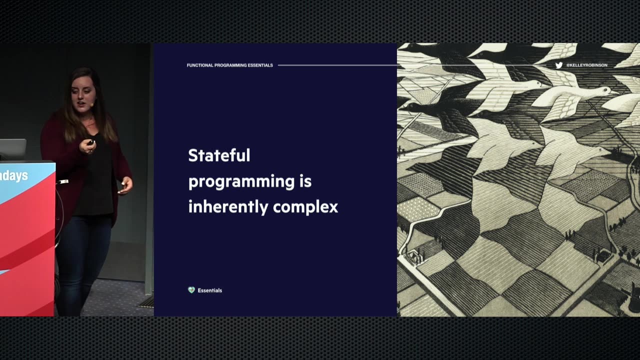 isolating logic and breaking our problems down, It wouldn't be as easy to reason about how things are working. Stateful programming is something that's inherently complex, and this is something that Rich Hickey talks about in his talk Simple Made Easy, which Martin referenced in his keynote on Wednesday. 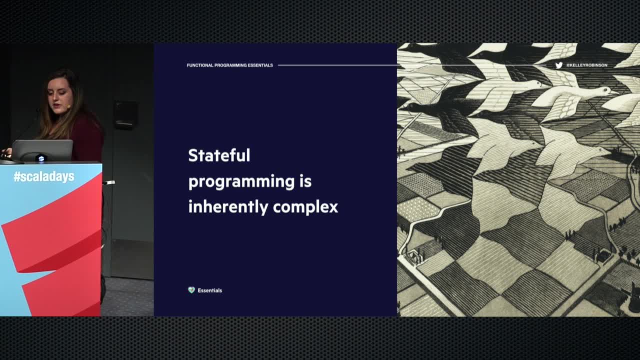 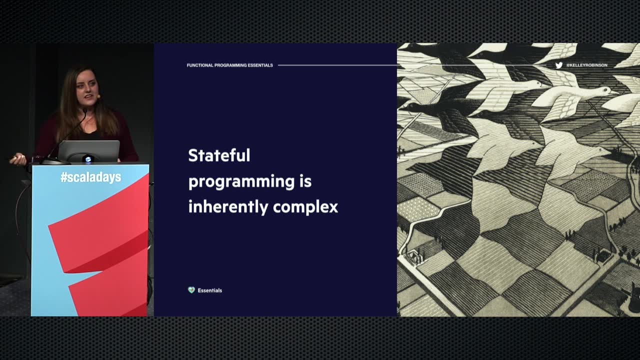 and I think it's a really great talk. first of all, if you haven't seen it, But the idea that programming with state is inherently complex comes from the idea that you're mixing data and time, and those are two concepts that are hard to predictably. 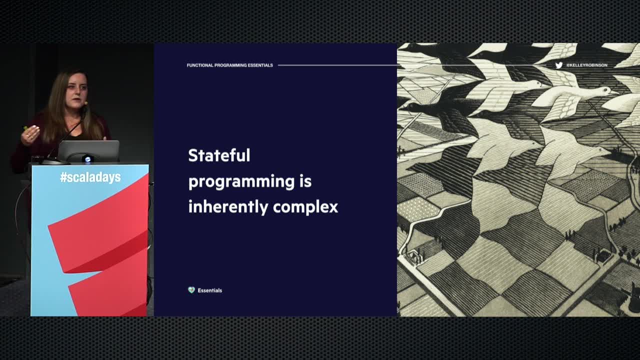 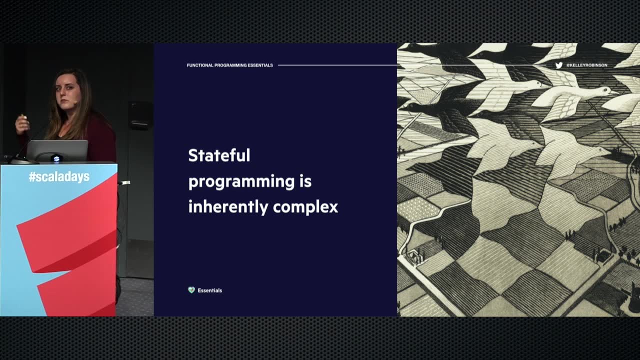 interleave, and that's why replacing state with values, using your data representing it using values, is really valuable to you, the programmer, in order to be able to understand how things are working. It's actually a lot simpler in the long run to think about data as values. 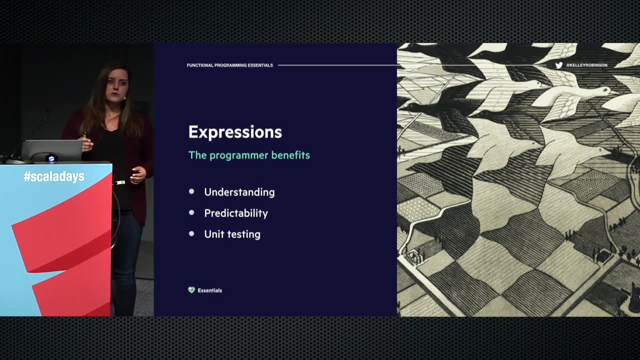 Bringing this together. most functional programming encourages the approach of using data as values. Most functional programming encourages the approach of using data as values, Using pure functions for as much of your programming as possible, of avoiding side effects until you need them to minimise the amount of unpredictability that there is. 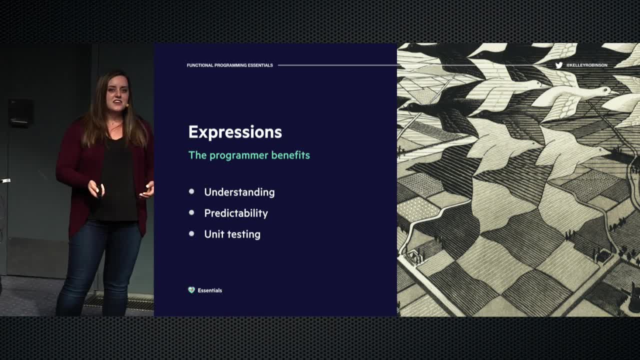 And pure functions are also infinitely easier to unit test, and so you can think about this. remember that this is a style. functional programming is a style. you can use this in any language, and so if you're doing any amount of testing in your code, which I really hope- 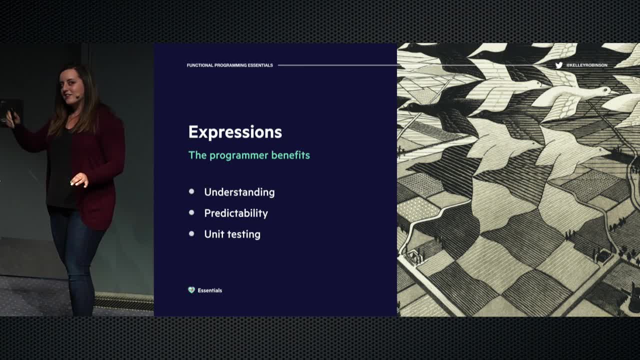 all of you are. you can program in this style in your Scala code, in your JavaScript code, in your Python code, in order to be able to better unit test these individual parts, these isolated parts, and be able to get the expected result back and know how your programs. 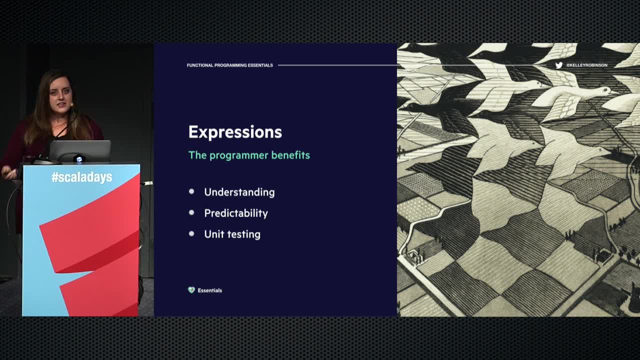 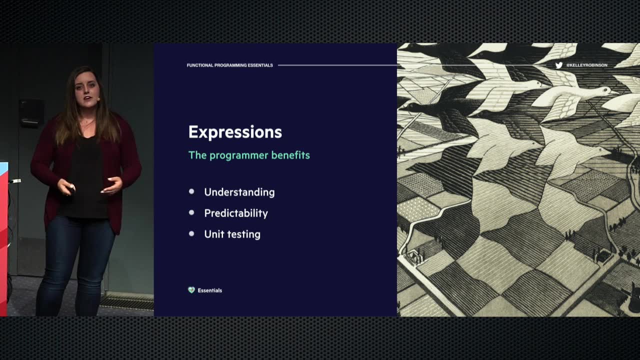 are behaving, and this is a way that you can avoid using things like testing mocks as much. If you're in a program and you have to write a lot of testing mocks in order to be able to test the behaviour of your code, that might be a sign that you need to break things down. 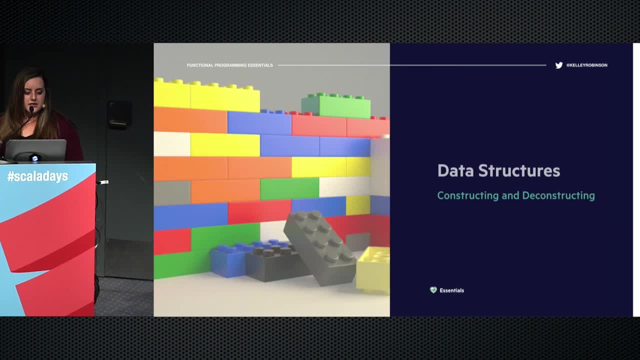 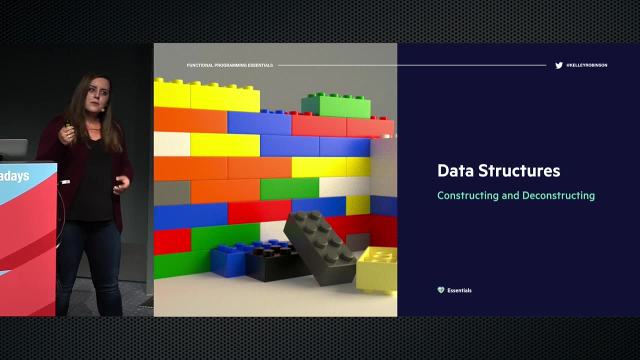 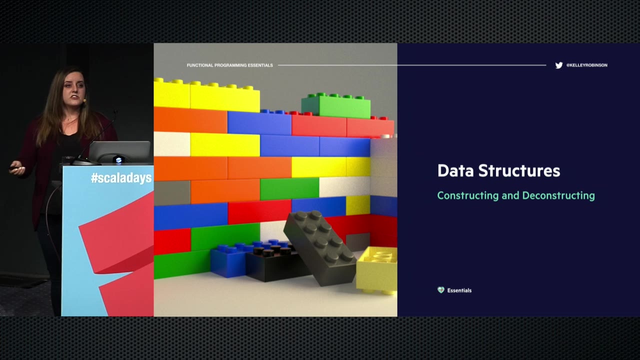 more. Continuing with Burge and his insights from his book, The next big insight that he had was in data structures, and so what Burge said was, instead of thinking about the location or the layout of data, he wants us to think of our data. 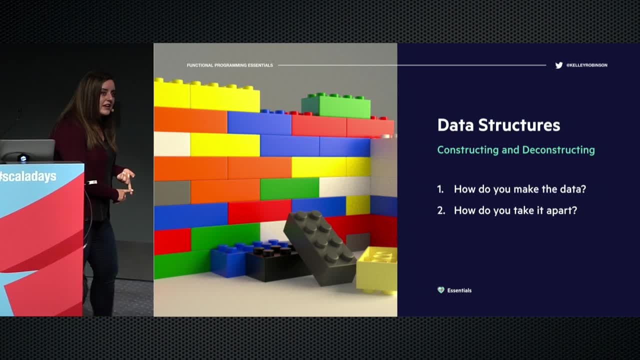 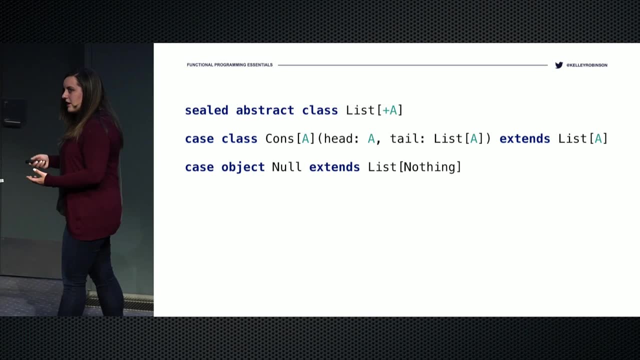 in a couple of ways. So, first, how do you construct the data, How do you put it together? And then, how do you deconstruct the data or take it apart? And in order to represent this using Scala, we're going to create a linked list data structure. 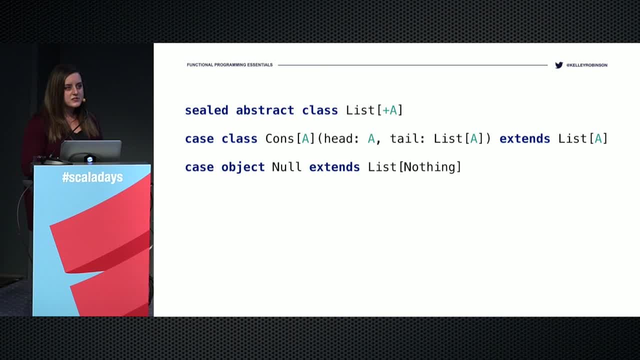 We can make this idea of constructing and deconstructing. We can deconstructing data more explicit by representing this in Scala and there's going to be some code in the next few slides. It's there to illustrate some patterns. Don't get too hung up on the individual syntax of the slides, but we can think about constructing. 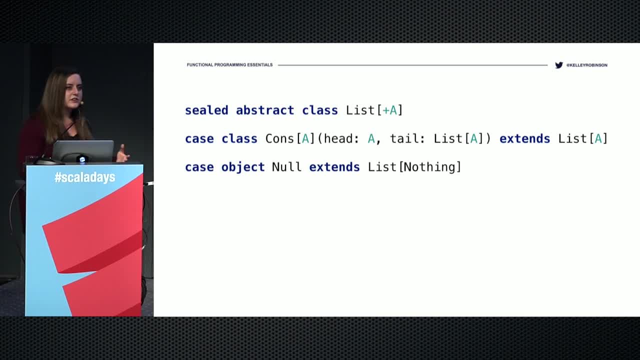 our list in a couple of ways. So if you're constructing a list, you're either going to have something- you're going to have a constructor, the cons- or you're going to have nothing- the null value- and then you're. 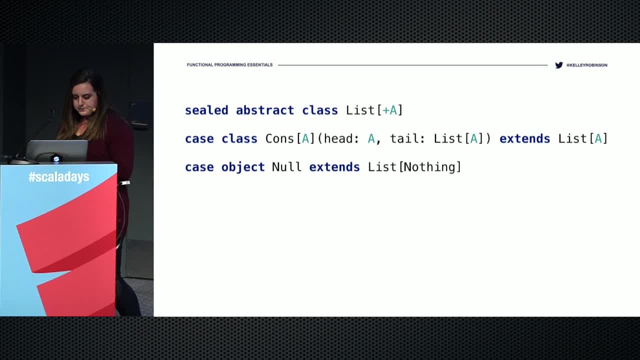 going to have to know what to do when you don't have anything to put in your list. And, in the same vein, you can think about what you're going to do when you don't have anything to put in your list. You can think about that when we're taking our list apart, when we're doing any kind. 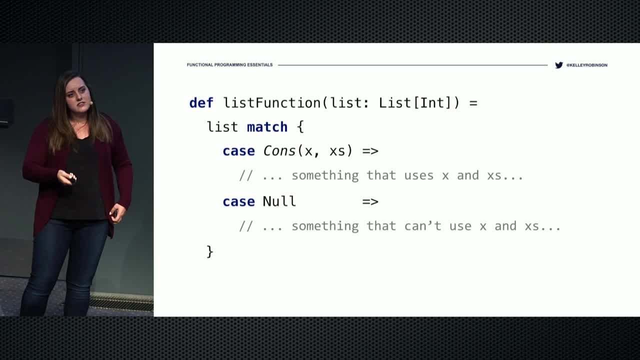 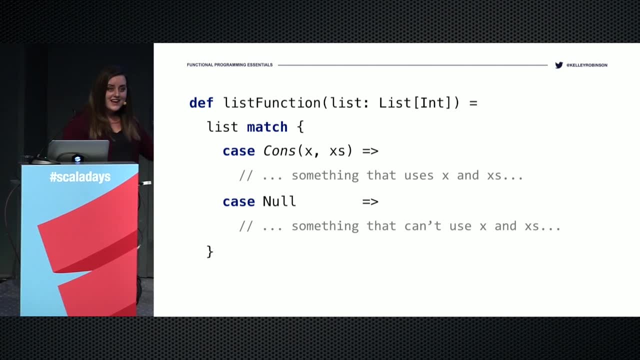 of operation on our list. every function on that would be deconstructed using something like this. Every function is either going to have to decide what to do when it has an element in the list or have to provide some kind of default action when it has nothing in the list. 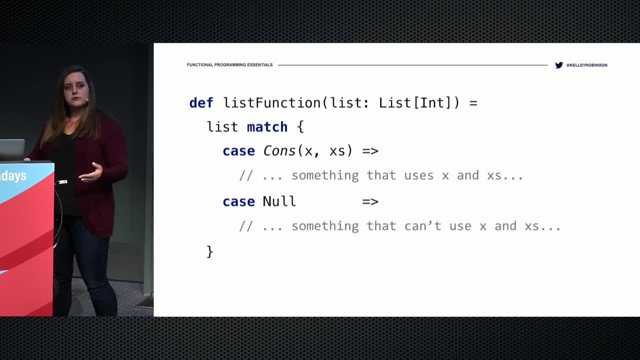 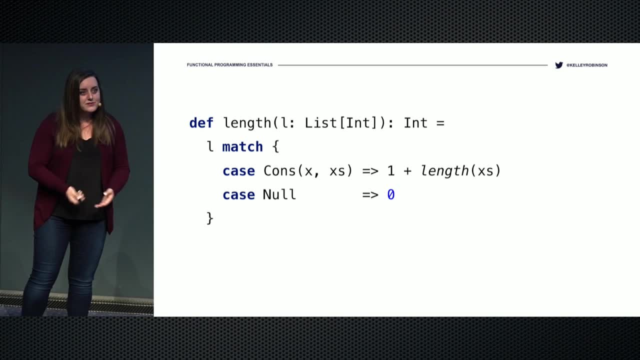 And once you have this kind of function, you can start to use this to define functions on our list. So, for example, we can write a length function on our list And in the case where we have something in the list, we add one. 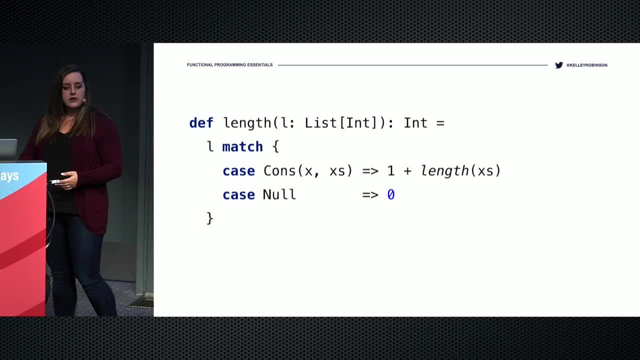 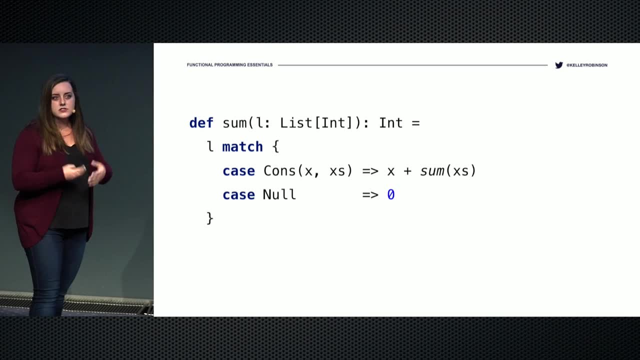 We have nothing in the list, we add zero. That's the default value. Similarly, the sum function on our list. if we want to sum all the elements in our list together, we add the head of the list to the recursive sum of the tail and again, if there's. 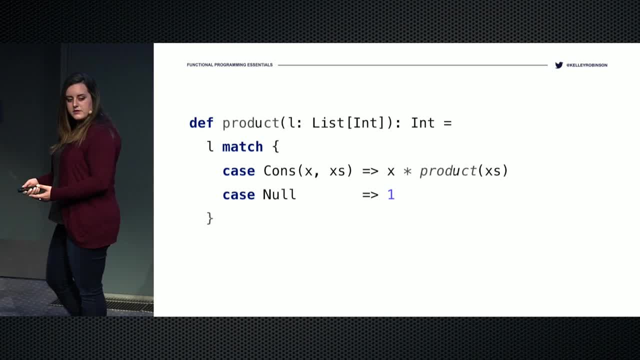 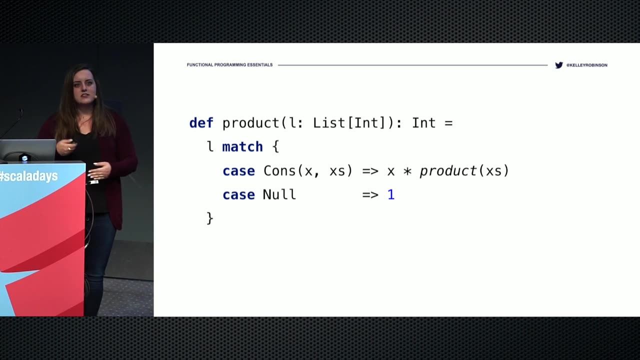 nothing in the list, we add zero. Very similar if we're taking the product of the elements in our list. we can add or multiply the head of the list to the recursive sum and then the default value there becomes one. So we want to see the pattern here, the pattern of how we're deconstructing the data, the 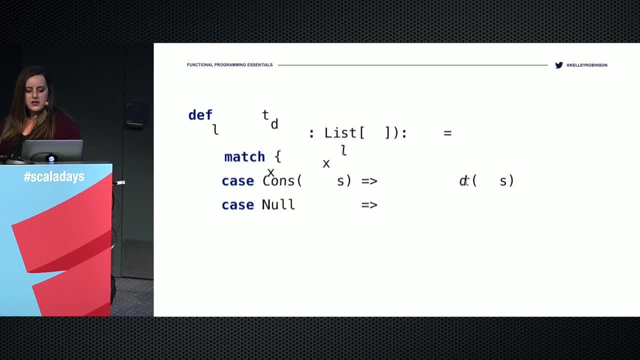 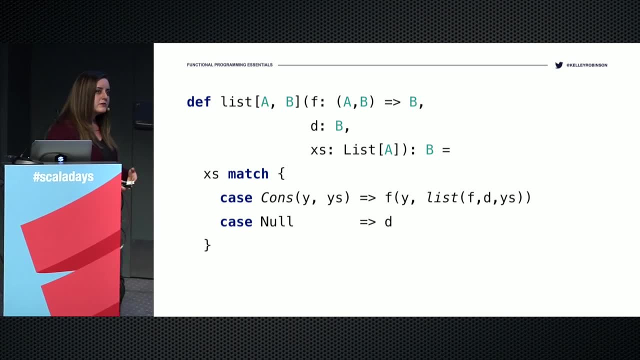 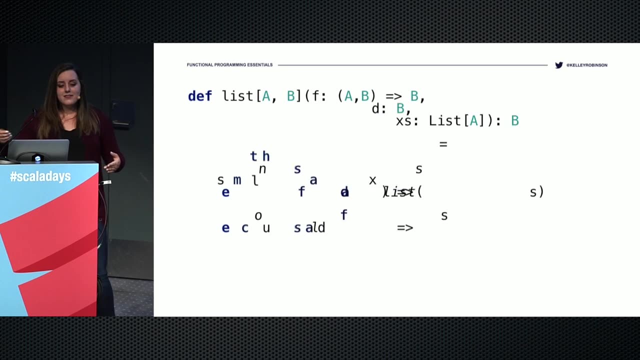 similarities of how we're doing these operations on our list And what we can do is actually represent those operations in a more generic form, And this is something that we can use to represent those other functions and abstract away that deconstruction in a more generic way that allows us to then rewrite our other length. 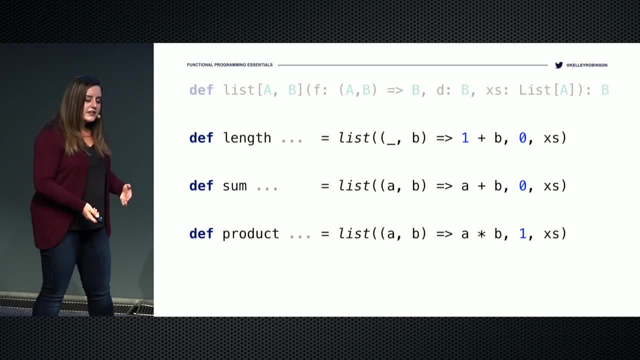 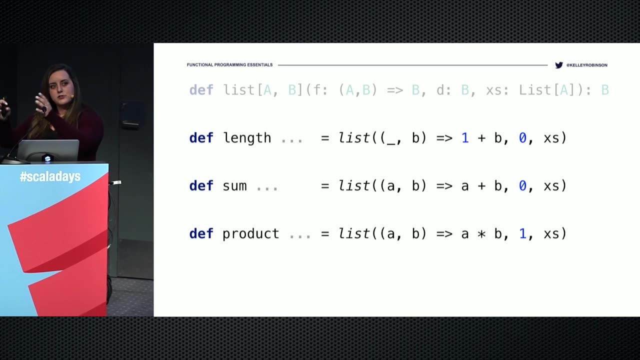 sum product functions like something like this, And so you do that. Take this helper function that we define, and then the idea of functional programming that comes into this is: we've isolated the parts of the program that are different. We've thought about how to deconstruct our data and abstract things away so that the 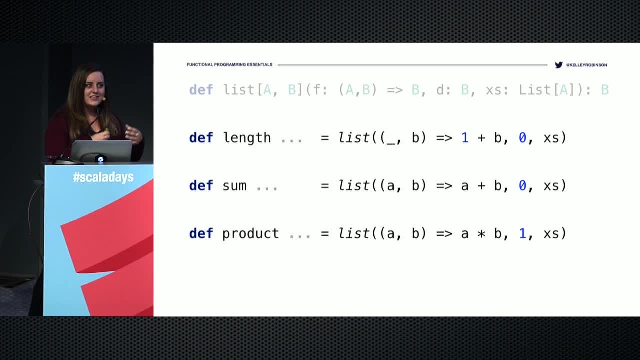 programmer, you is left with the interesting parts, the actual intelligent thing that you have to decide what to do with your program And this whole class of functions becomes apparent and you can think of how to define other functions using this kind of abstraction. 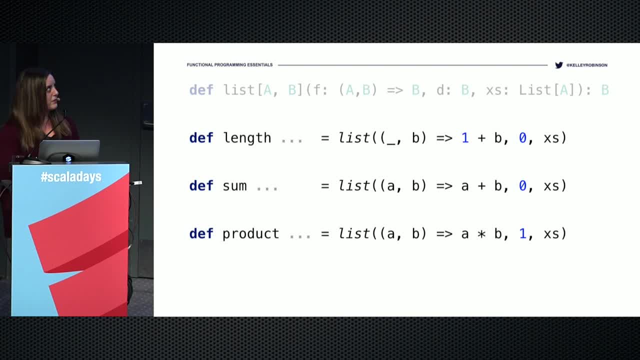 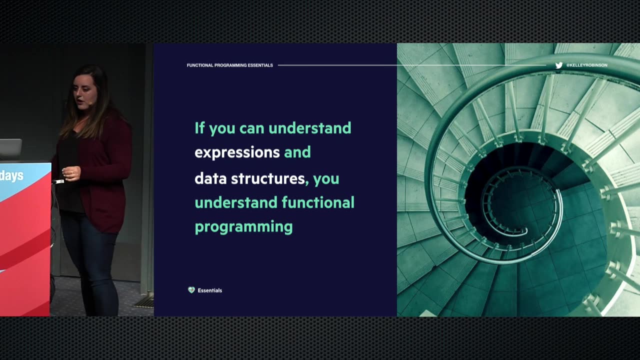 And that allows you to focus on the parts that are different, Focus on the logic that you want to add into these functions in order to make them work for what you need to do. And this is a huge thesis of Burgess' work: If you can understand data structures and expressions, you're good to go. 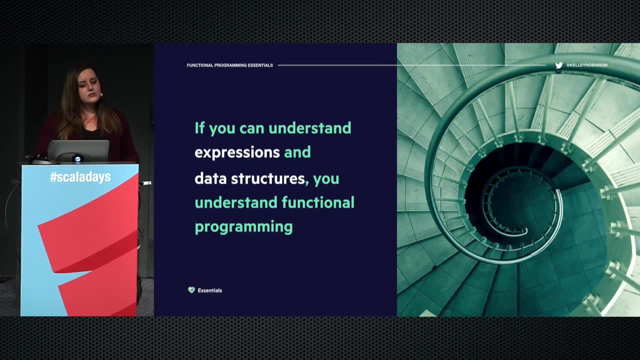 Thinking about data structures. even more functional programming allows the structure of your programs to match the structure of your data, and when you do this, you're left with the idea of focusing on the data structure, and then you're left with the idea of focusing. 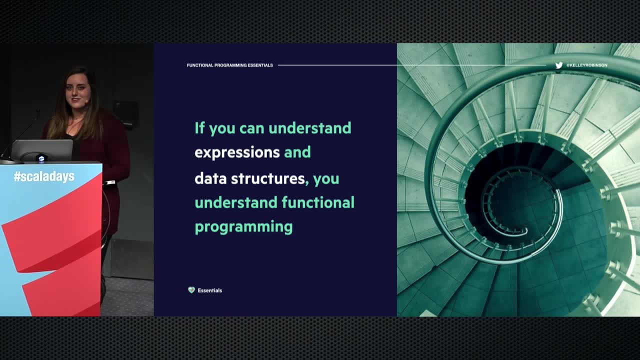 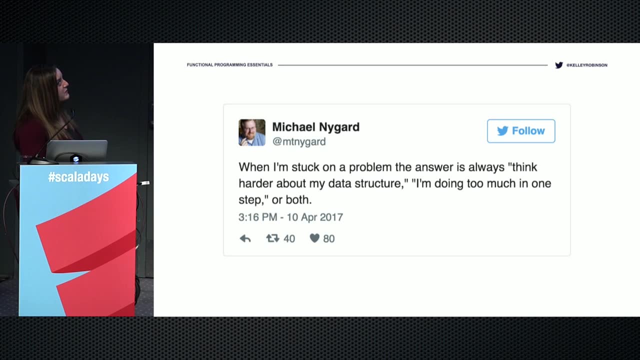 on the interesting and challenging parts for you, your business logic, that you actually need to spend time thinking about. So I thought this was pretty interesting. I saw this on Twitter just about a month ago. I don't know if this person has ever met Burge or read his work, but Michael here observes: 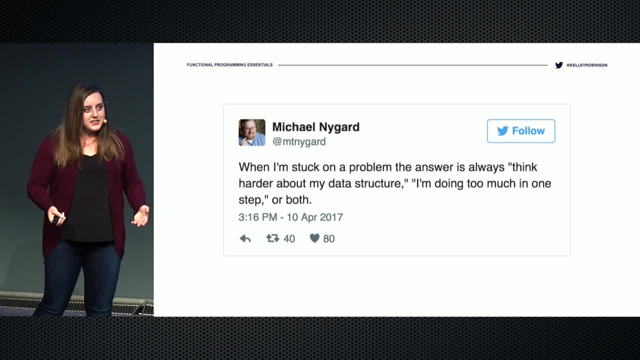 that when he's stuck on a problem, the answer is always: think harder about my data structures or I'm doing too much in one step. And so he's coming to the same conclusions in 2017.. And I think this goes to show that a lot of things haven't materially changed since then. 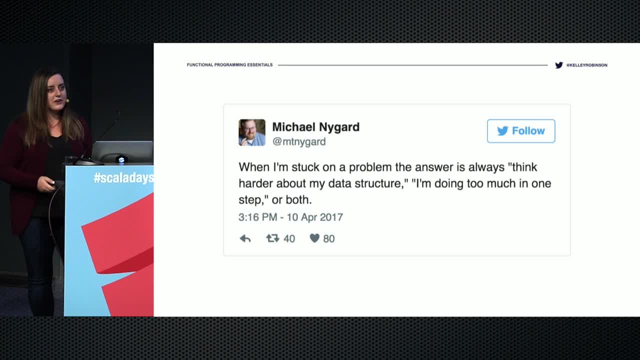 There's been a lot of innovations. there's a lot of stuff that we're doing now that's making it cool and more interesting and, in some ways, easier for us, but the core principles of functional programming haven't changed in a long time. They're not changing. 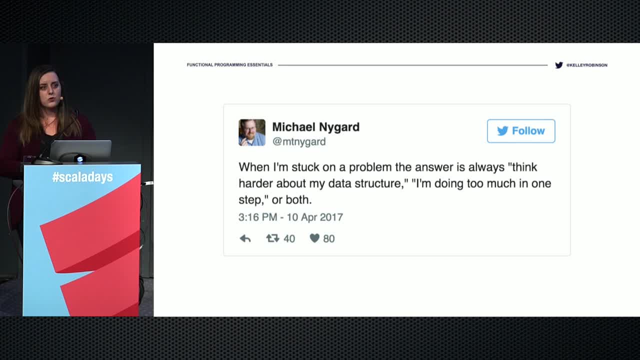 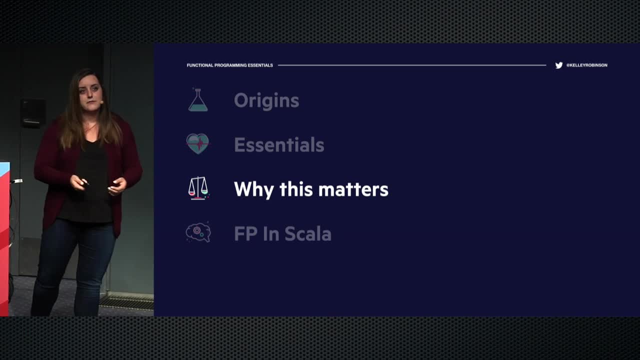 And we can be effective as functional programmers by keeping those core principles in mind. So it was a privilege. So it was a pretty intense distillation of functional programming. Now let's get into the fun part. Why does this matter for you? Back to this ladder. 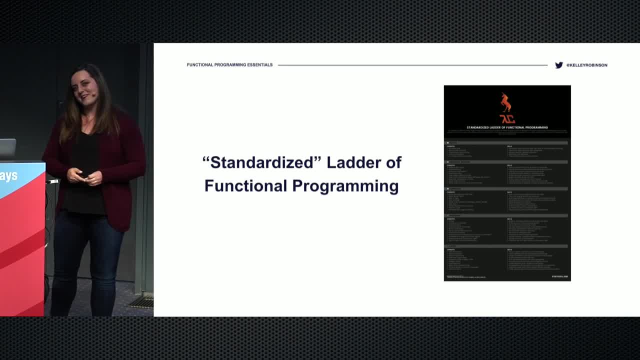 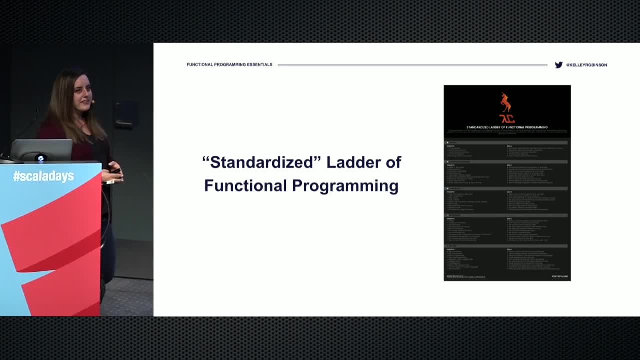 So there are 44 concepts listed here, 44 concepts. Last year I talked about the free mode out at Scala Days and it took me three months to really get a mastery on that. I did some math. If every concept on here takes me three months to learn, that's 11 years of learning functional. 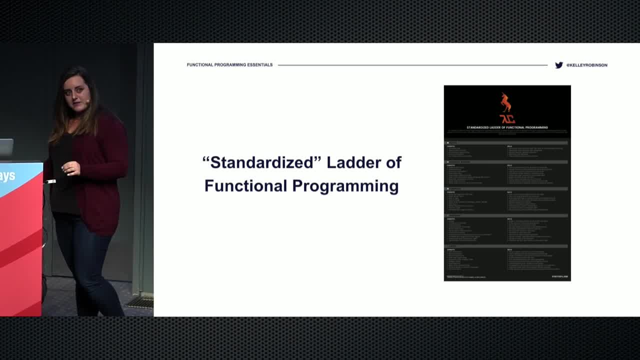 programming concepts, And so maybe some of you have a lot of fun. You have 11 years to do this. Maybe some of you are smarter than me and it's not going to take you three months to learn each one of these concepts. 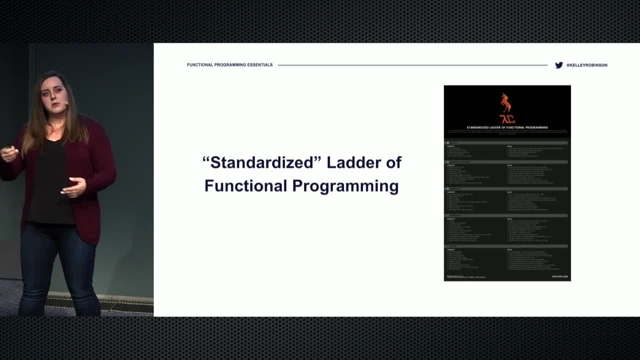 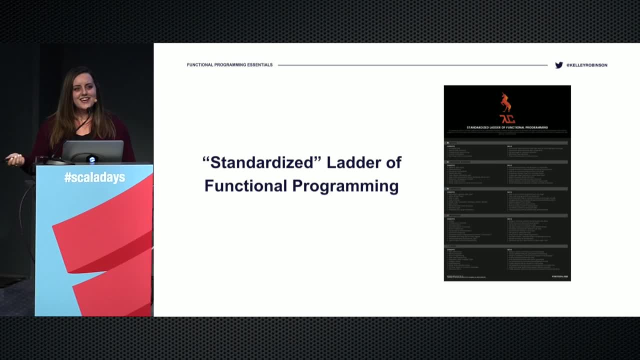 And maybe some of these things are the things that we don't think we know, but we do already know and we just don't know that we know them or we don't know that they're called those things that we know. but even if that's the case, that's still a problem, because 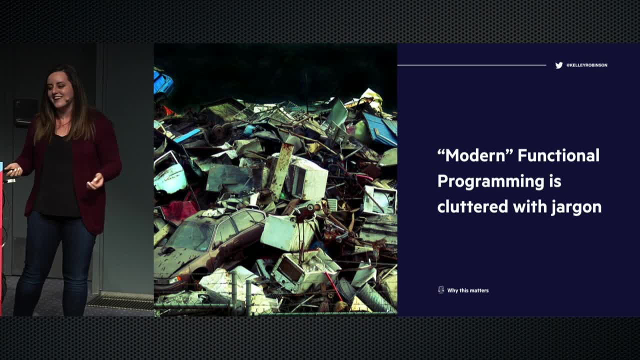 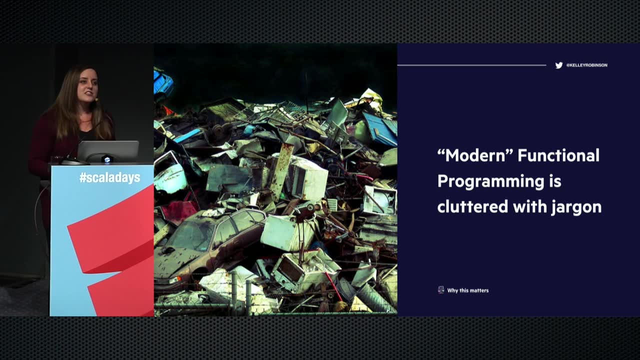 modern functional programming is littered with jargon. After the Northeast Scala Conference in March, A software engineer at Twitter gawked at all of the jargon that she heard. It was so complicated and so prevalent that they couldn't keep up. and this is a smart. 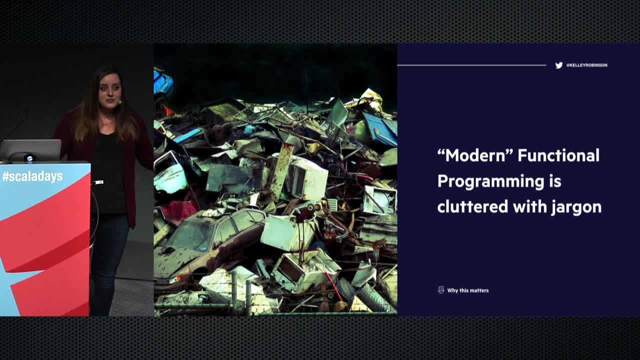 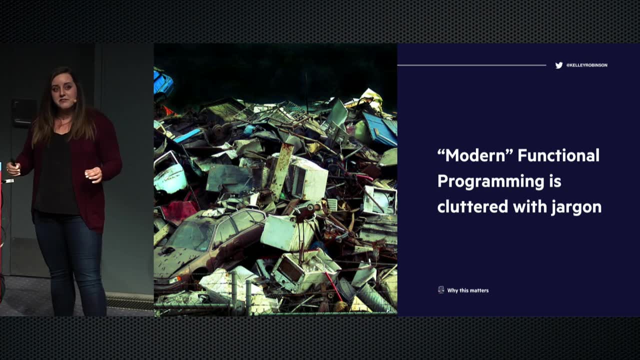 person. This person literally wrote the book on React Native and they're a software engineer at Twitter. Twitter has like hundreds of Scala engineers. They acquired a Scala training company. They've got a lot of good resources to be educating people internally on how to use. 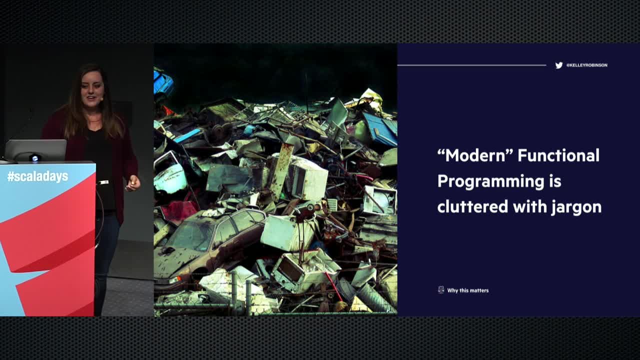 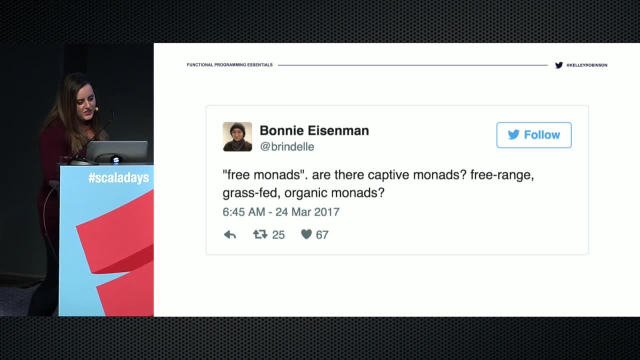 Scala at their company, but still it was overwhelming. This is what Bonnie observed. So the cool thing about this is Bonnie then took some of the concepts that she heard and looked them up, figured out what they were, wrote a blog post on it, spent her Saturday. 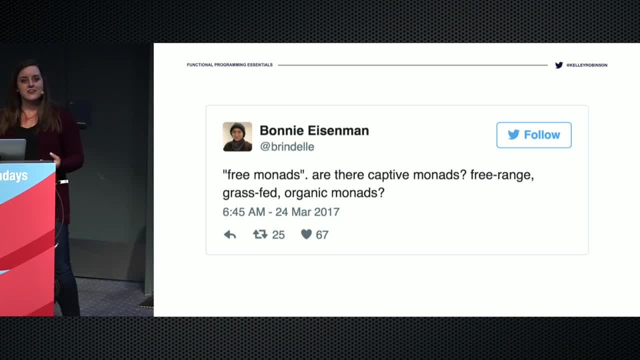 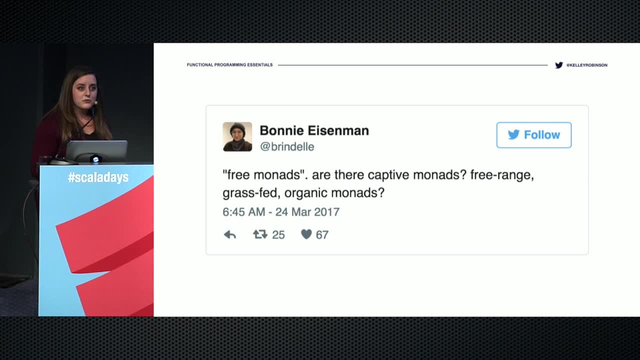 reading other blog posts, watching conference talks in order to get an understanding on a lot of this stuff, And it's really great that she did that and I think that was really valuable, especially the fact that she wrote up a blog post talking about her findings. 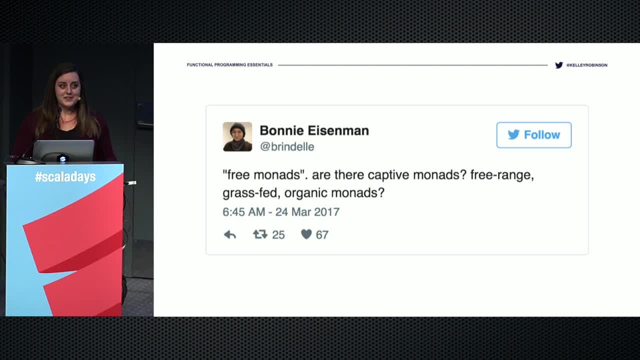 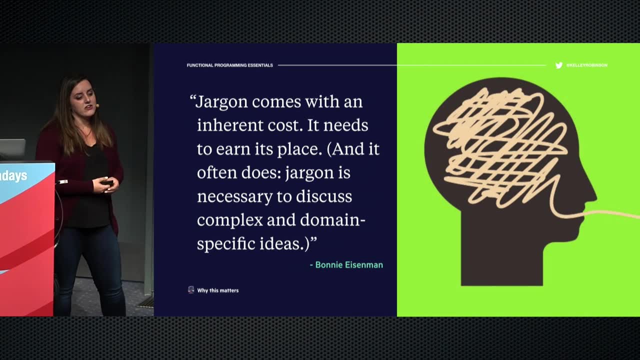 But not everyone is going to do that, nor should they be expected to. As Bonnie notes in the blog post that she wrote, jargon comes with an inherent cost. It needs to earn its place, And she goes on to say that it does. 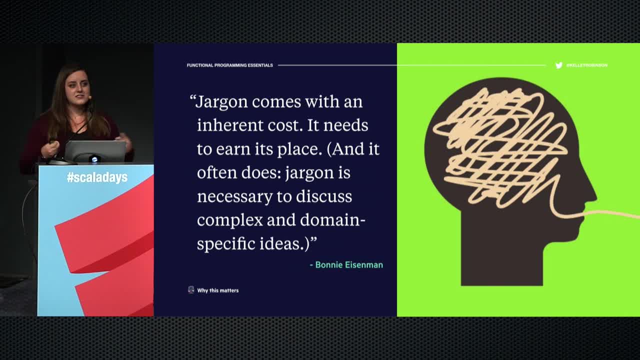 We use jargon all the time to share context and discuss domain-specific ideas, and that can be more efficient if everyone shares the same context. but that's a pretty big assumption right there Everybody's on the same page and it's a hard assumption to make, depending on the context. 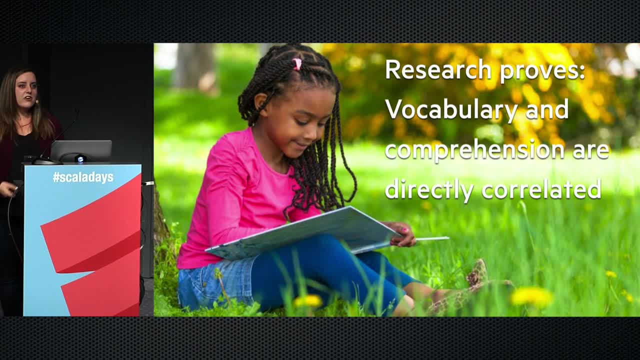 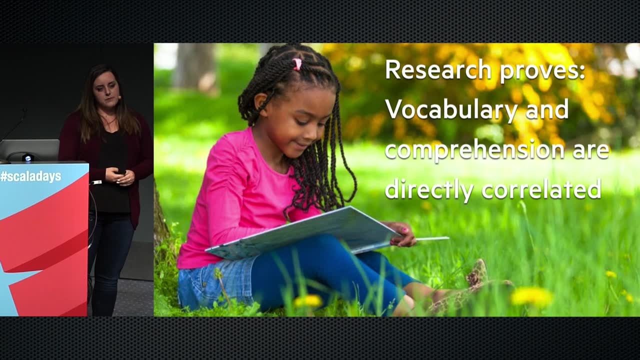 that you're in This inherent cost that Bonnie talks about. this has been well studied. We can look at years of education research to back us up. So, in education, if you're learning a new language, either for the first time that you're, 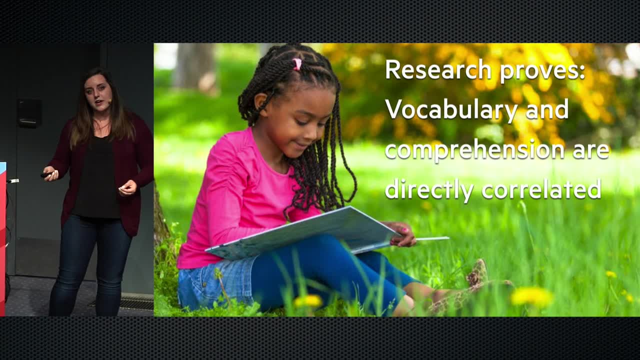 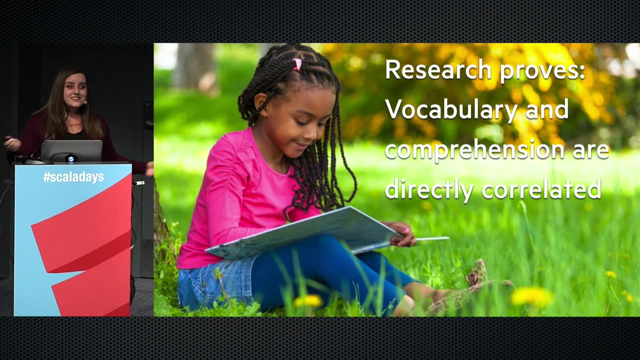 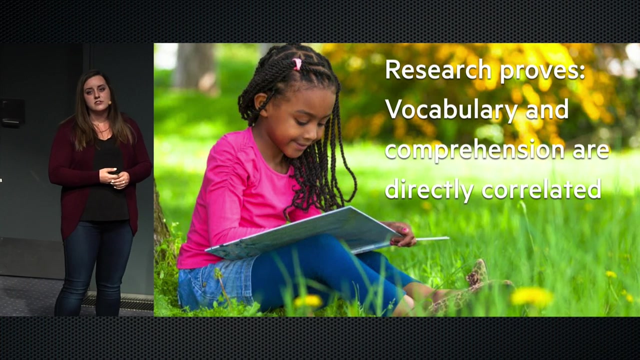 learning to speak or read, or if you're learning a new and foreign language. the size of your vocabulary is directly correlated with your overall comprehension. Oh and the interesting thing is that providing new definitions for words doesn't even cut it. So in a 2000 study, a couple of researchers provided vocabulary definitions for unfamiliar 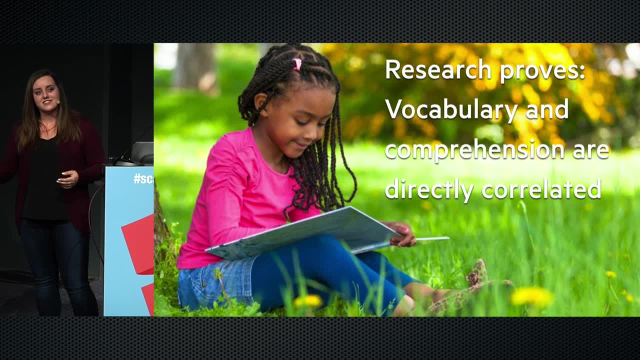 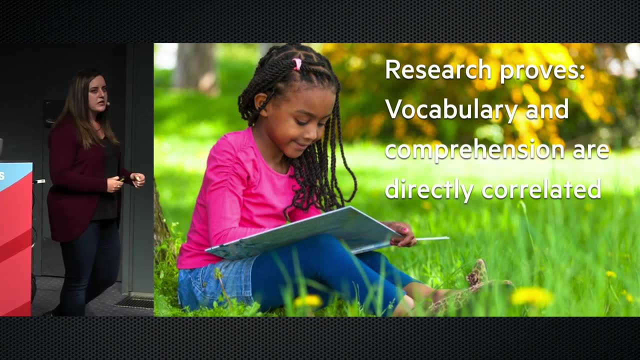 words to a group of people and asked them to construct a sentence using those unfamiliar words. And when they got the sentences back, they graded them And only about 25% of the returning sentences were deemed acceptable. So the researchers tried again. They rewrote the definitions more specifically for their audience, specifically for the participants. 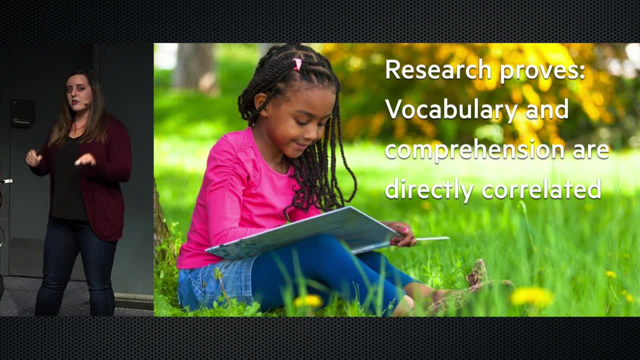 that they had in the study, who I think were like six-year-olds, And they crafted these definitions specifically in a way that they thought would be useful for those participants. So they made them very good definitions, And then they got the sentences back again. 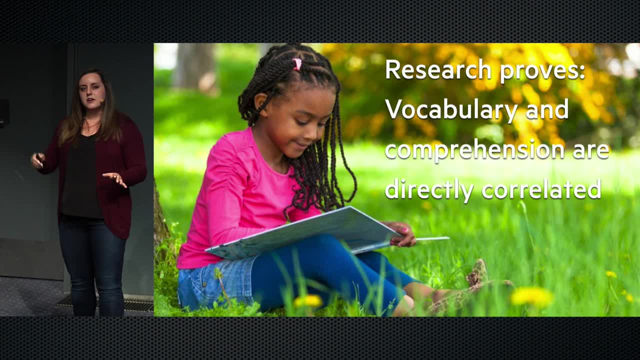 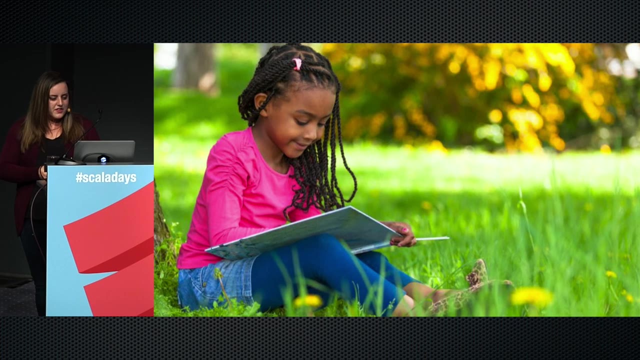 And the number of acceptable sentences went up. It went up to 50%, And 50% is a lot better than 25%, but 50% is still, probably, to most people's mind, failing. It's not great. And so the researchers observed the following: 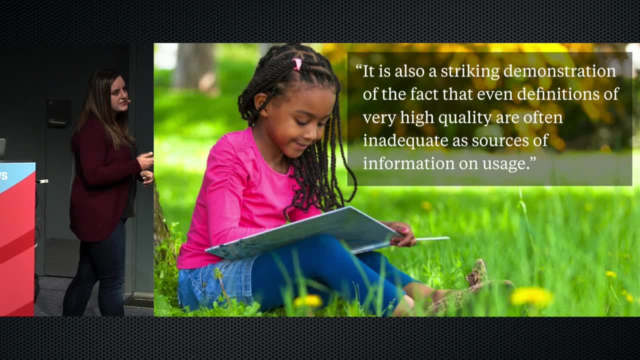 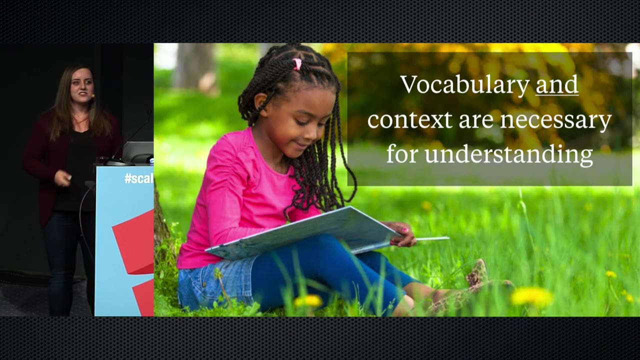 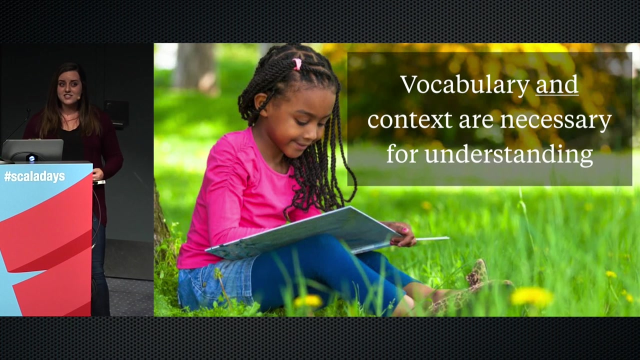 They said. it's a striking demonstration of the fact that even definitions of very high quality are often inadequate as sources of information on usage. People need context, They need practice to really understand these things. The more jargon that we start to introduce into whatever domain we're in, especially. 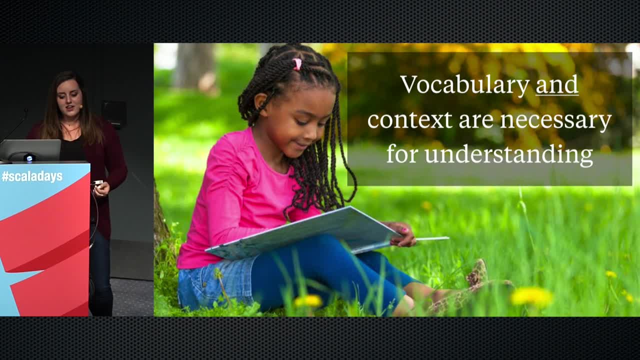 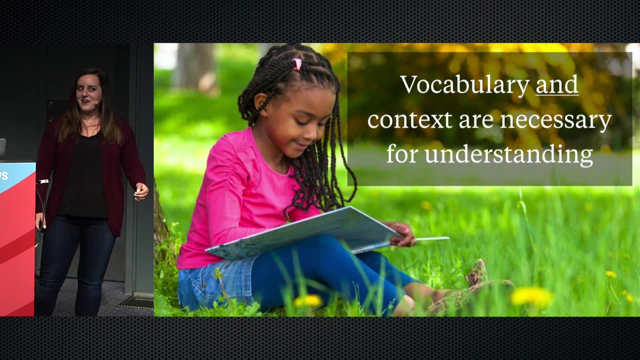 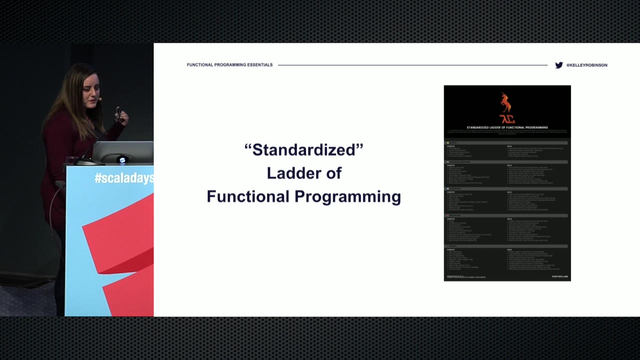 programming, the harder it becomes for someone to learn, And that's really scary, because even if someone does understand the concept, it doesn't mean they know how to use it. So people were mad about this, and the conference responded by updating the latter. 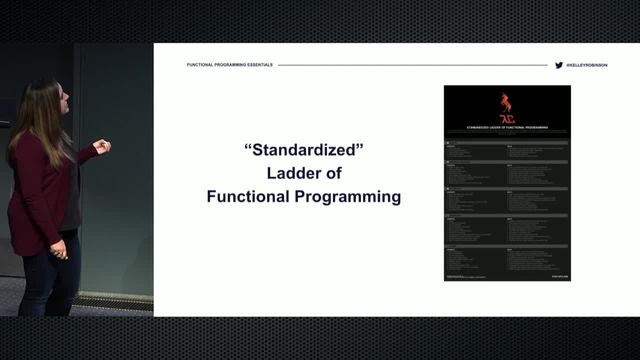 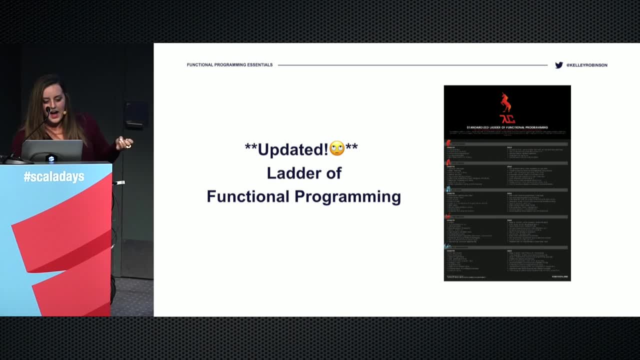 But they literally just introduced more jargon. The only thing that's different now is, I think, they changed the name of the section. so now, instead of being a beginner, you're like an ice caramec or something, I don't know. 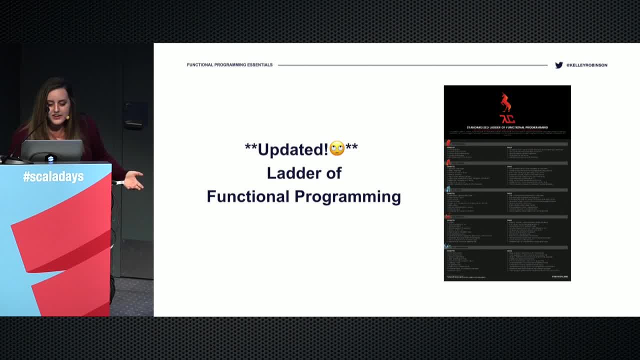 I don't know if I should be offended by being called a fire lub line or not. I don't even know what that means. I don't know if I'm pronouncing it right. The problem with this is not the jargon, It's not the names of the divisions. 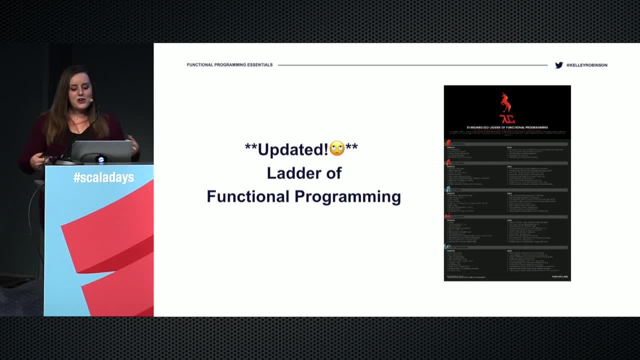 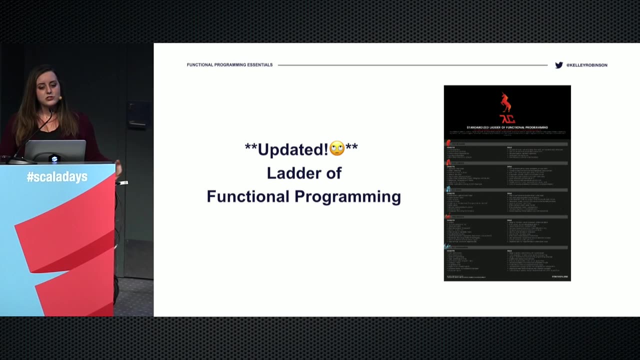 There's no context for any of this. Why does knowing advanced monads make you a better programmer? In my opinion, it doesn't. When you present something like this as a ladder, the connotation there is that you're expected to climb, that you're expected to grow and that, if you don't, you're doing. 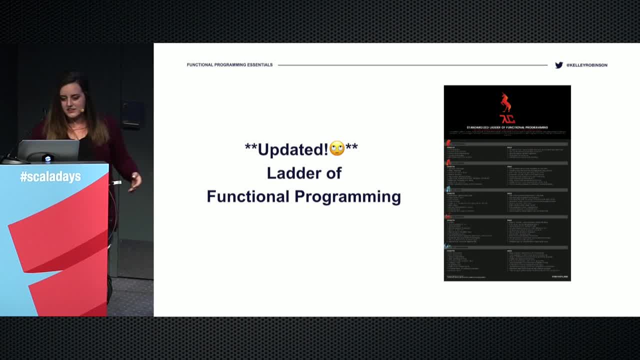 something wrong. You're expected to become the ice skrig or whatever that is, But that's not necessary. The essentials that we talked about, those are all caps. Those are all captured in the first rungs. So if you want to think about it as a pyramid, you need these fundamentals, the expressions. 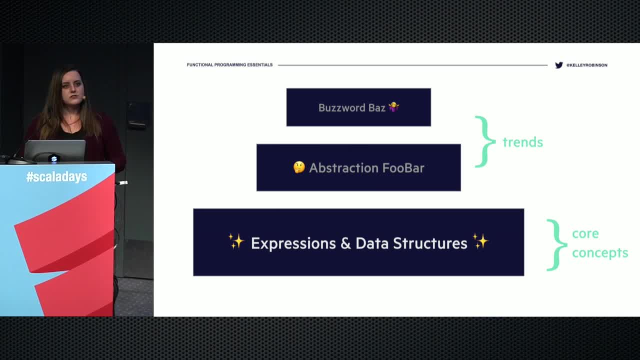 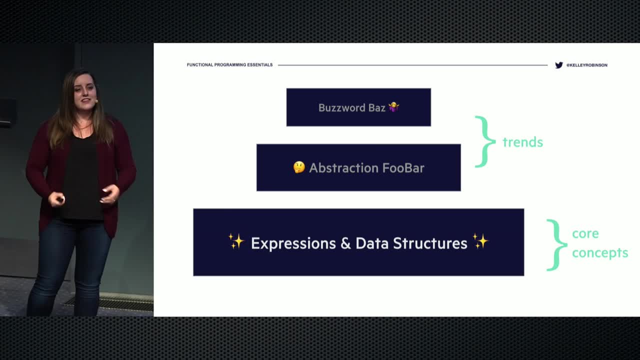 and the data structures in order to understand the essentials of functional programming and everything on top of that. the buzzwords, the syntactic sugar. those are trends. They may have staying power, They may not- We don't really know- but it's the flavor of the weak buzzword that people are using. 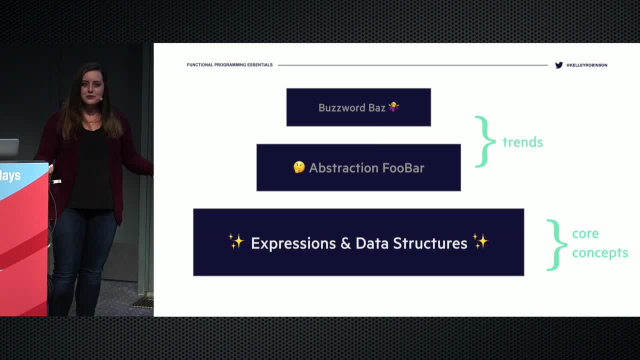 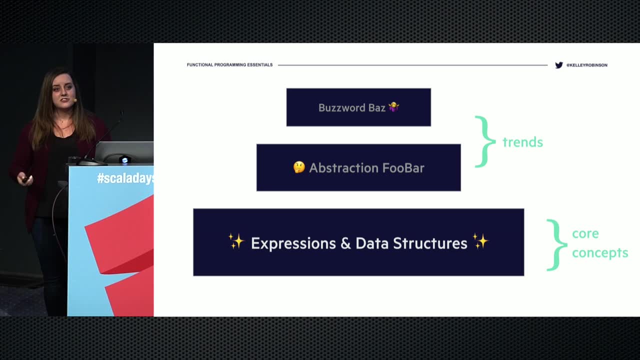 a lot and introducing into their projects, and maybe they're doing it in a way that makes sense and maybe they're not, But these things haven't been around enough, nor do they have enough context and shared understanding in most cases to really be useful. 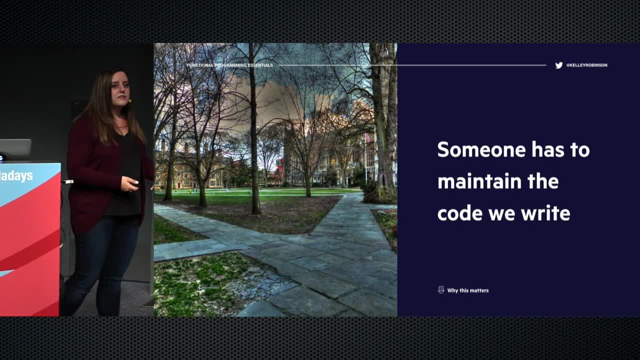 Something that these lists do give you is a list and idea of concepts to go out and learn about if you're curious and wanting to do that, and that's something like something that Bonnie did, And sure I can see the value in that. 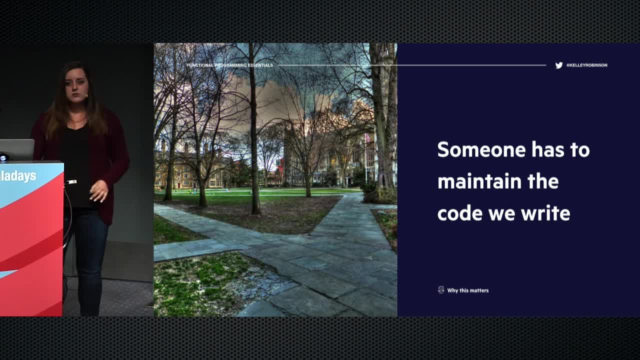 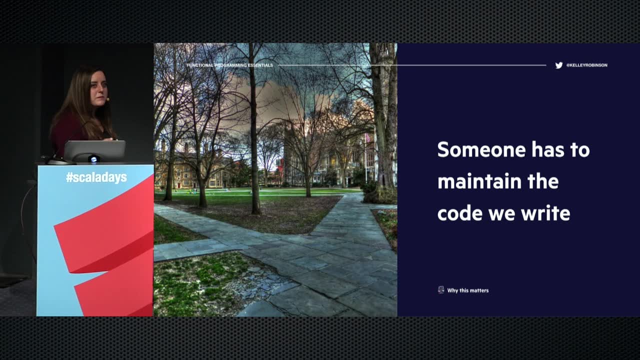 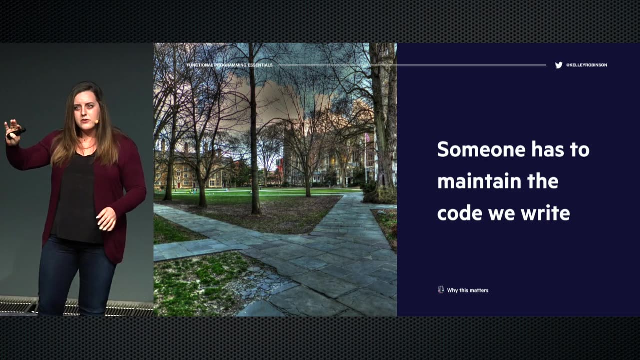 Learning for learning's sake is great. It's why we continue to fund research institutions. Thank you, EPFL. But where it becomes problematic is how many people in here are industry programmers And how many people are academic programmers. Okay, So there's a significant number more of industry programmers, and where things like this become 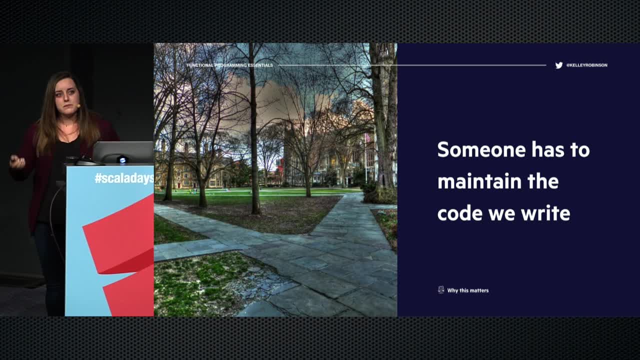 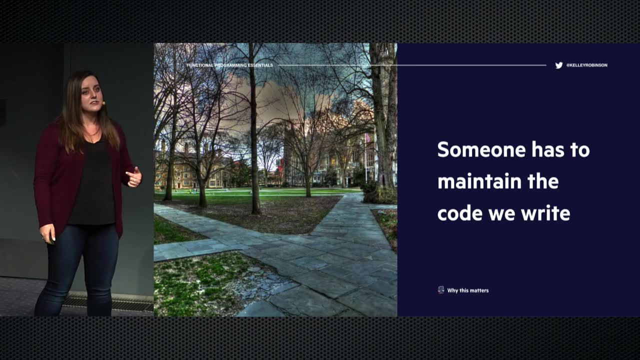 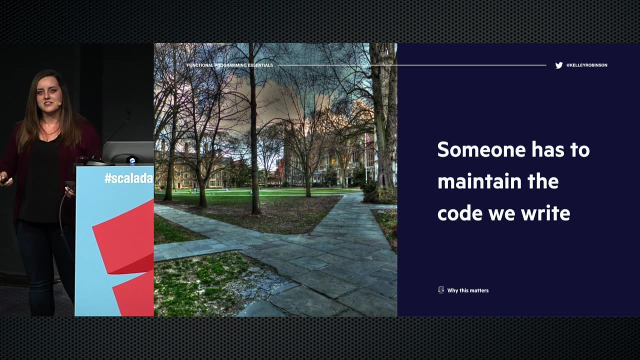 problematic is when you decide to take something like profunctor optics and build that into your feature release, because you heard me talk about it at this cool conference talk you went to and no one on your team knows what that does. It's learning some new vocabulary without knowing how to use it in a sentence except. 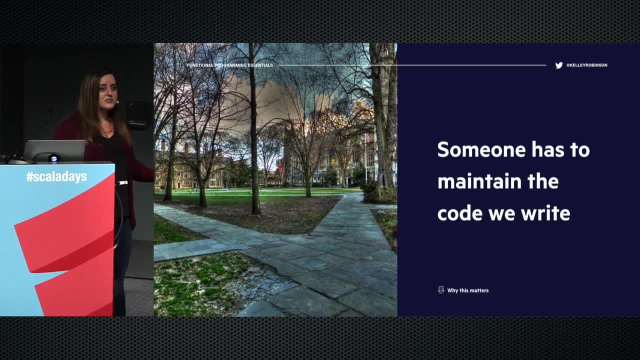 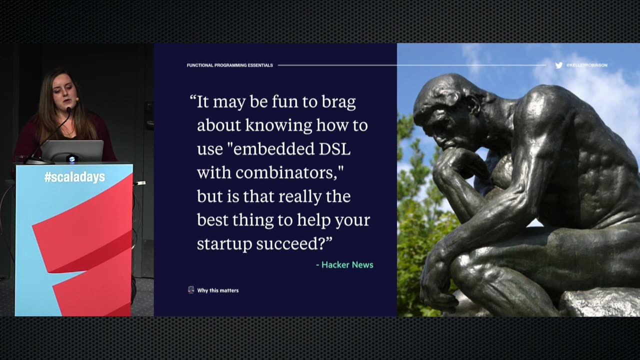 for now that vocabulary is something like free monads or tagless final interpreters, and the sentence is the production service that I have to be on call for, And for once someone on Hacker News agrees with me. So this person said it may be fun to brag about knowing how to use embedded DSL with. 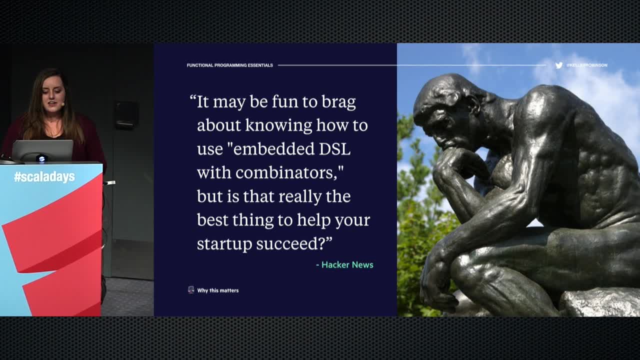 combinators, but is that really the best thing to help your startup succeed? I'm a big proponent of that. I'm a big proponent of that. I'm a big proponent of using the right tool for the right job, of finding. 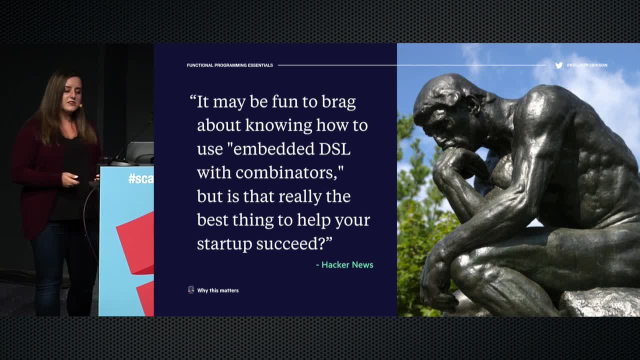 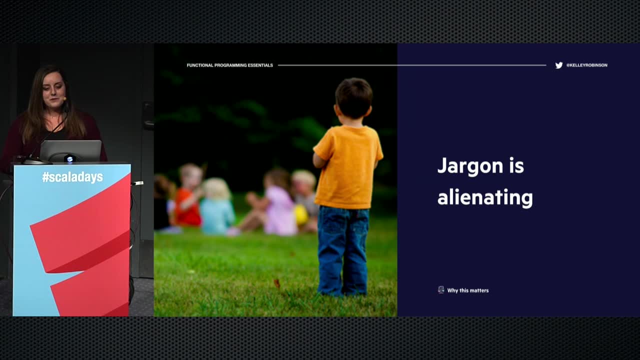 Of solving problems rather and not just building solutions, Not to mention that jargon is super alienating, especially for new programmers. A large amount of this category-theoretic terminology that we hear hasn't earned its place. At one of the first Scala meetups I ever went to, there was a panel. it was a panel discussion. 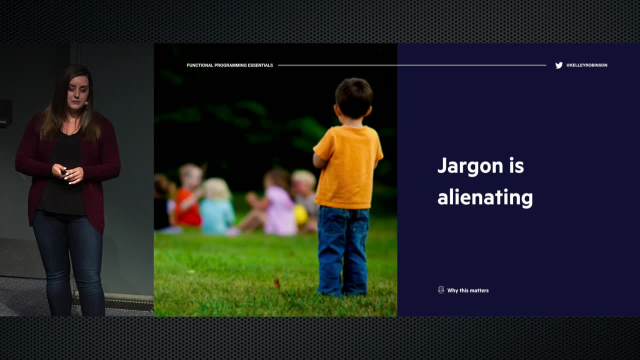 and someone on the panel said that it was good that Scala was hard to learn because that made sure that only people that were serious about it were the ones that stuck with it, And that's really hard to hear. It's really hard to hear when you're three months into learning a new language you gave. 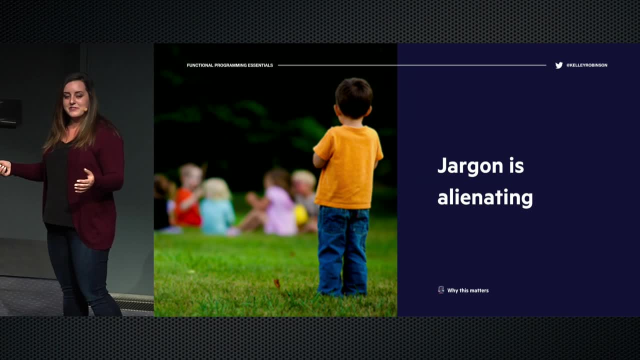 up your Wednesday night to go meet people in the community, learn some stuff, and somebody's up there being like, eh, you're probably not going to cut it. If you're someone that's heard these things, that's felt alienated like this, I'm here. 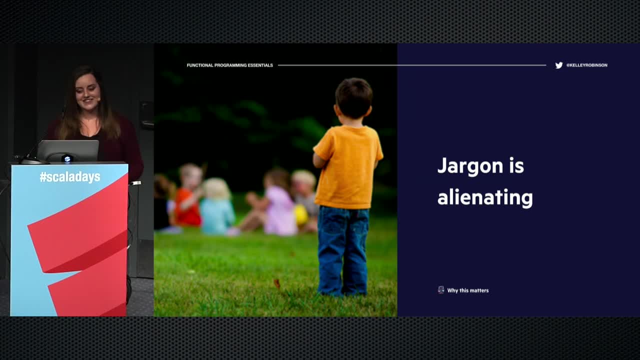 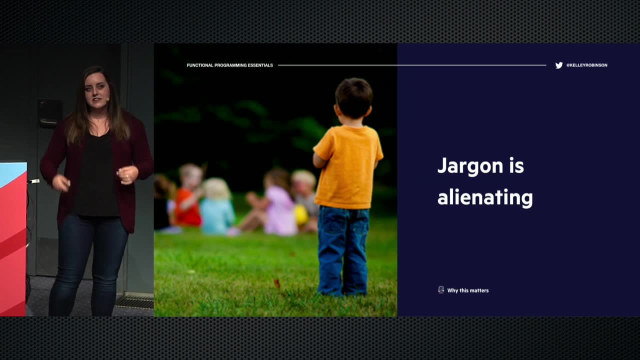 to be a voice of reason. I don't think that we should be saying things like this. Too many conference talks focus only on the syntactic sugar and not the reasons why you might use these things. I think that we need to get more focus on the why of things and not just the how or 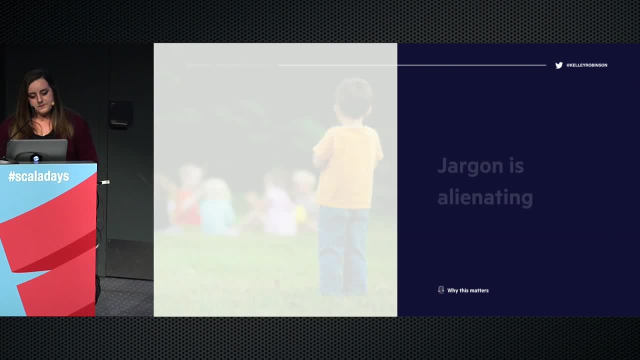 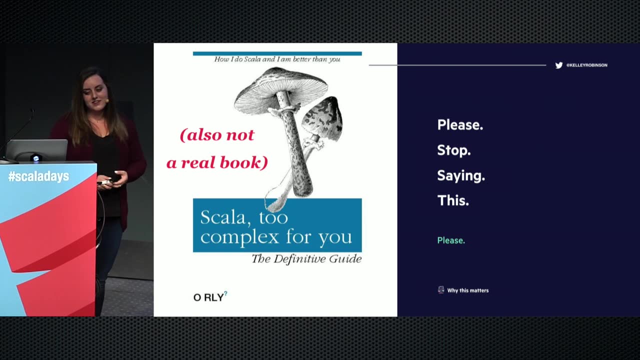 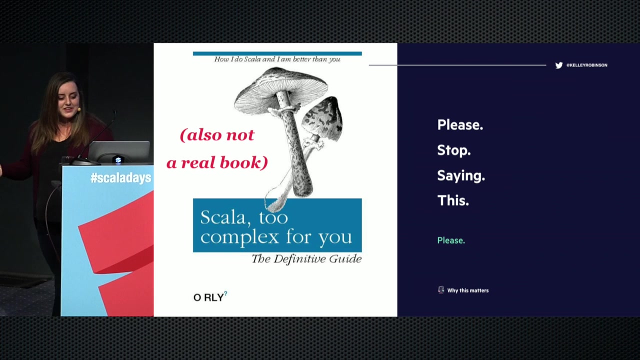 the what. So please stop saying things like this. Scala is not too complex for any programmer. This is funny because it's a widely held belief- also not a real book, by the way. Please stop saying that you have to know things like advanced monads in order to be an advanced 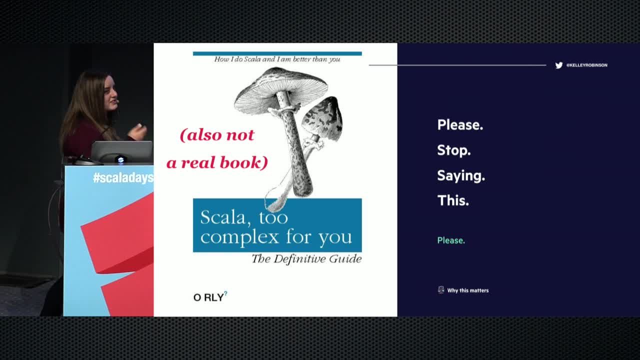 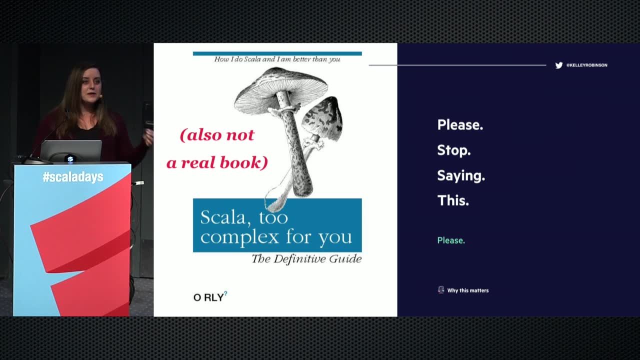 functional programmer. If you understand the essentials that I mentioned, the data structures and the expressions, you can accomplish a whole hell of a lot, And the rest comes down to the dynamics of your team and the culture that your individual team has figured out. 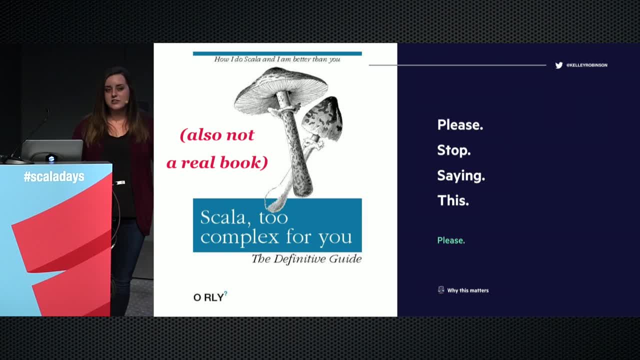 Perhaps you're working on a team that has interest. Introduce certain abstractions, introduce certain syntactic sugar, and that's great, But make sure that you're keeping in mind the overhead there, that you have a plan for bringing new people into your project and an understanding that these are concepts and 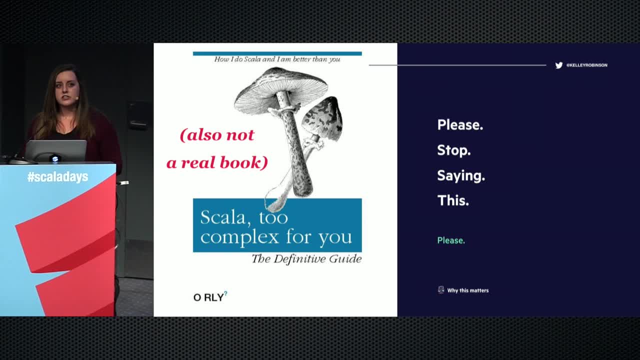 jargon that people may not be familiar with, and they're going to increase your ramp-up time. If you're someone that's writing more blue sky Scala, as Jessica Kerr coined it, you can still be an expert functional programmer without this stuff. 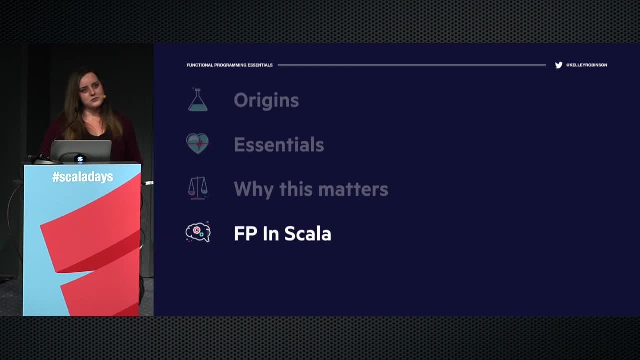 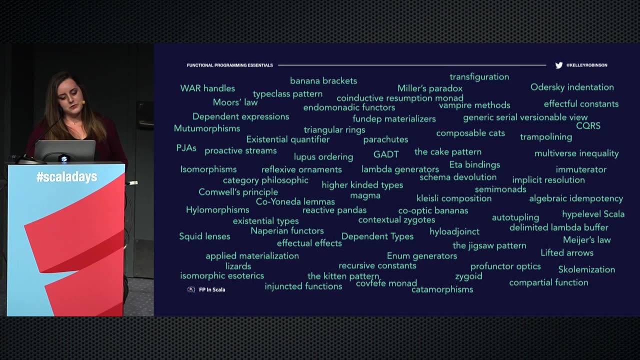 And that brings us to the end of the session. I hope you enjoyed it. That brings us to functional programming in Scala. There are a lot of things that you can do when you talk about functional programming in Scala. I'll give you a minute to take this in. 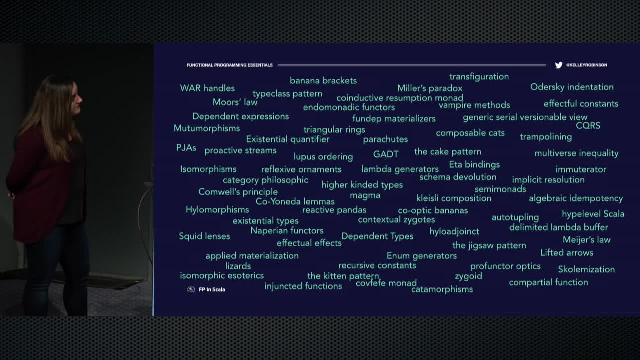 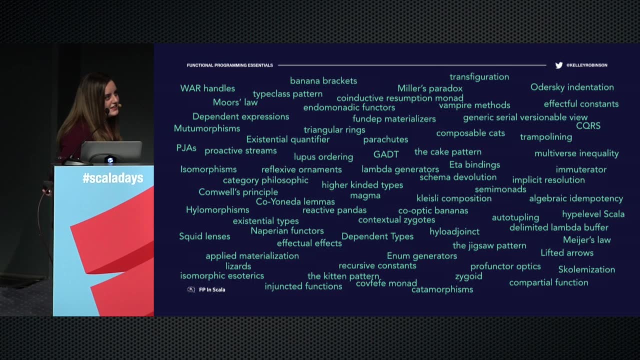 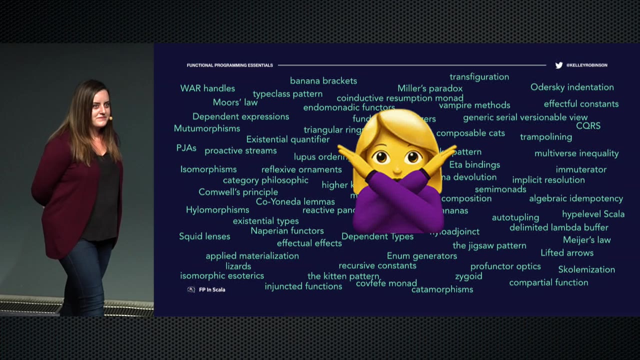 I think I've read about 75% of these and that's why I'm here. So some of you probably figured out about 75% of these aren't real, But the challenge is figuring out which 75% that is. It's hard. 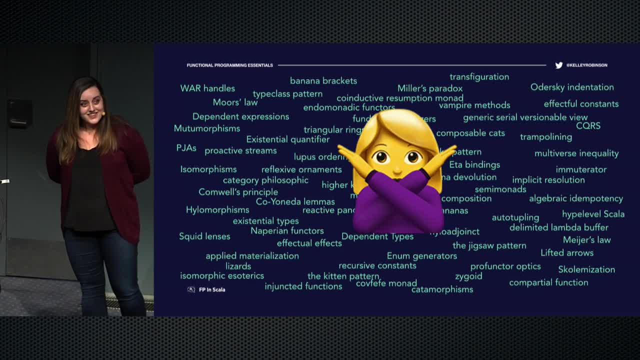 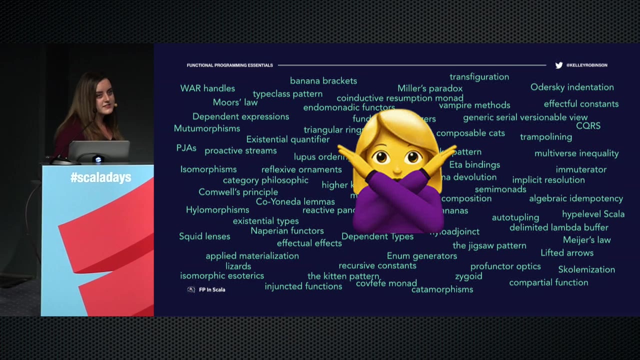 We made some of these up and I accidentally invented real ones. Apparently lifted arrows exist, But some of the stuff, so some of my favorites- recursive constants- that can't happen. transfiguration is a class that you take at Hogwarts. immuterators are not real. 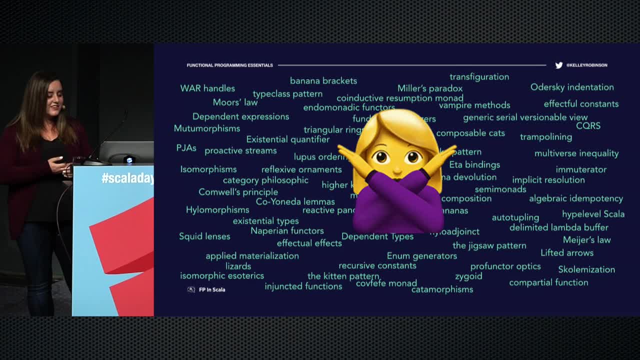 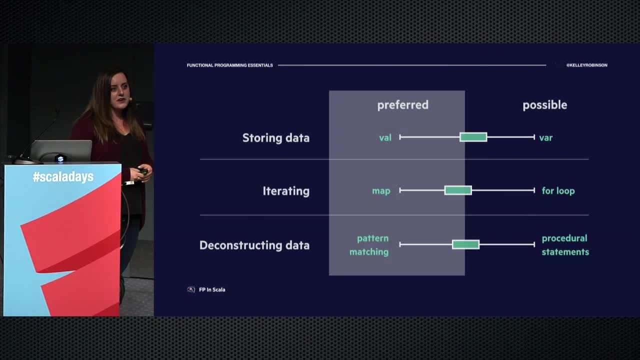 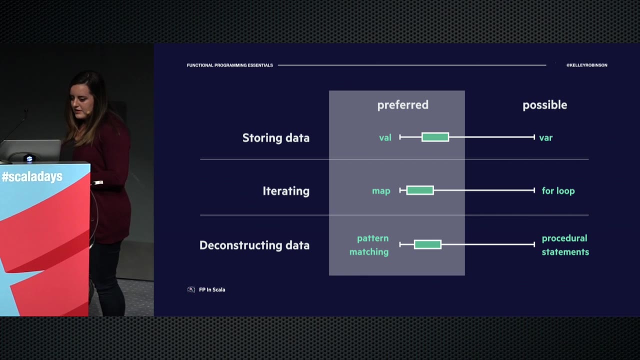 So these are things- these are jargon that we hear about in the scholar community a lot. This is not what we're talking about when we're talking about functional programming in Scala. What we're talking about is this: A series of tradeoffs that you have to make every day as you're writing your code. 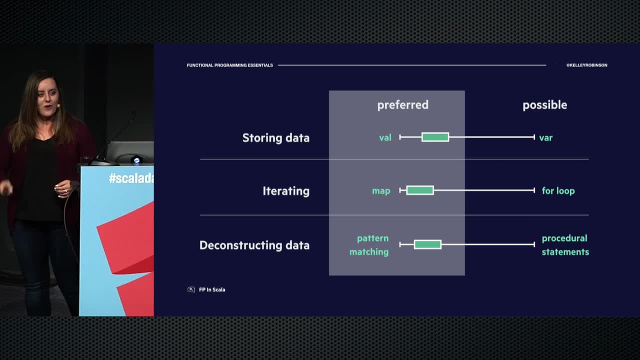 Scala makes functional programming easy. It also doesn't require it. So when you're thinking about how to write your programs and how to be more functional, think back to the essentials, to expressions and to data structures. maybe using some buzzword makes sense in your domain. It makes the thing that you're trying to solve possible, but don't forget the overhead there. You might be wondering what I think about the libraries dedicated to functional programming abstractions. These libraries exist and all I can say is that your mileage may vary. libraries like 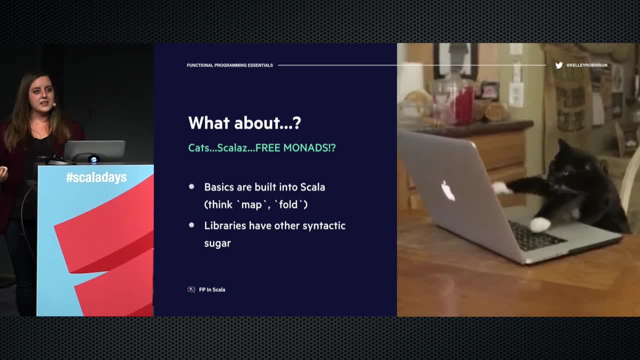 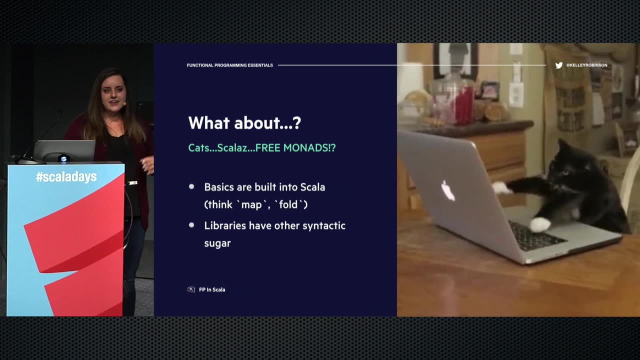 CATS promote themselves as functional programming extensions to the Scala language And there are completely practical reasons that you would pull these into your projects. but they can get very complicated very quickly. Okay, Okay, Okay, do appreciate is the folks at places like underscore and type level that are doing a? 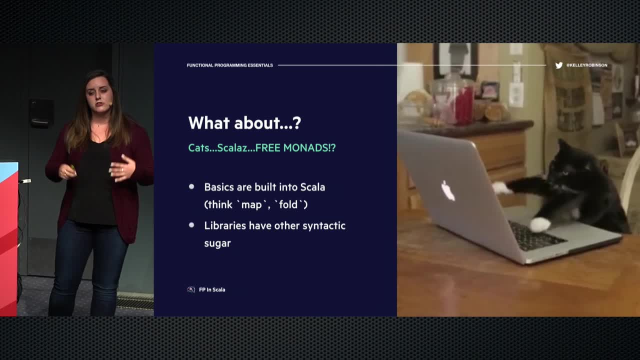 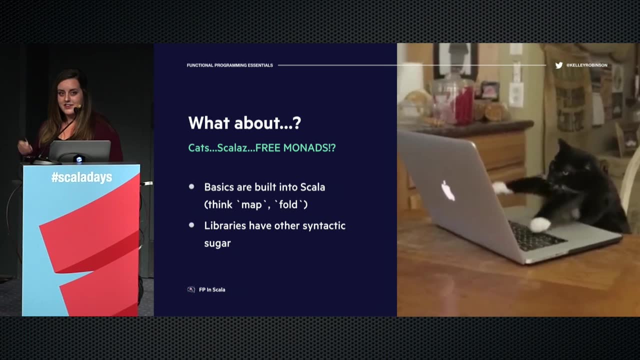 lot of stuff to contribute knowledge back to the community, contributing more than just these libraries, but also documentation and learning resources and how to master some of this stuff. That stuff matters. If you're interested in getting into open source. the easiest intro in my experience is contributing to the documentation. Earlier I talked a lot 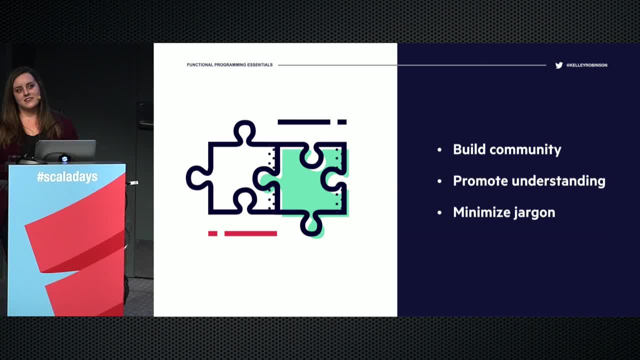 about the history of functional programming That doesn't end in 1975. It doesn't end in 2017.. At the risk of sounding cliche, we're still building that history today. We're still building the future and the past of the functional programming community. We have a lot of work. 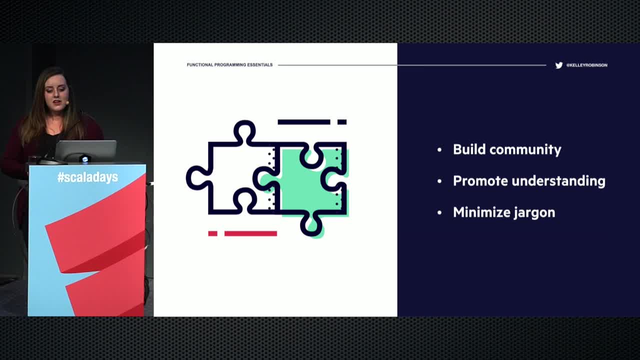 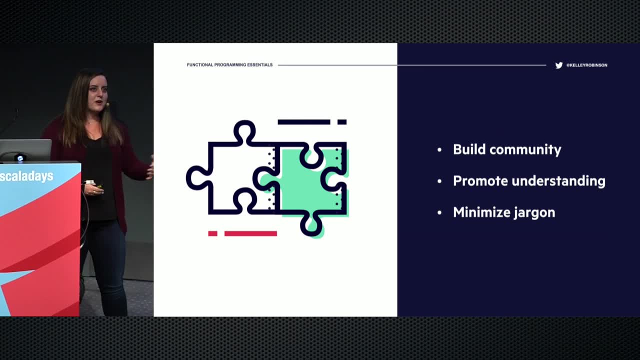 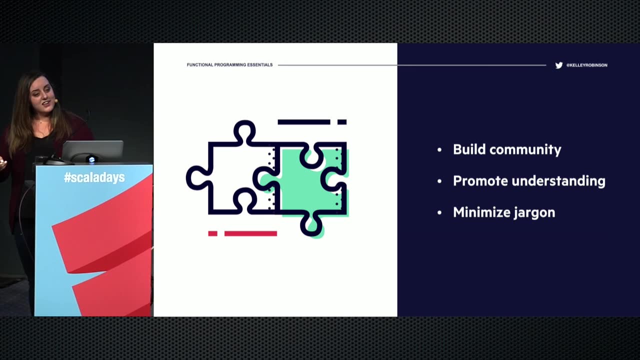 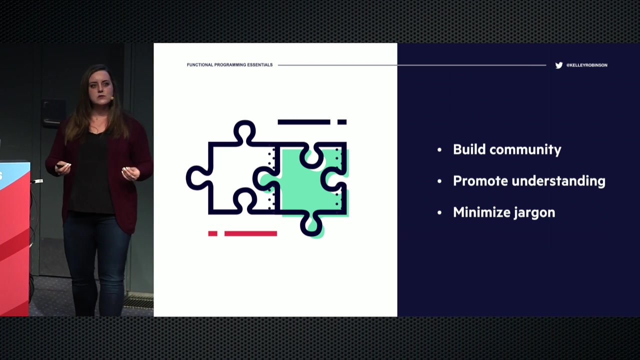 to do to make functional programming and Scala more welcoming. but by focusing on the essentials and bringing the definition of functional programming back to expressions and data structure, I think we can accomplish a lot. This paradigm exists because thousands of people- all of us included in this room- decided there was more than one way to write programs. People, 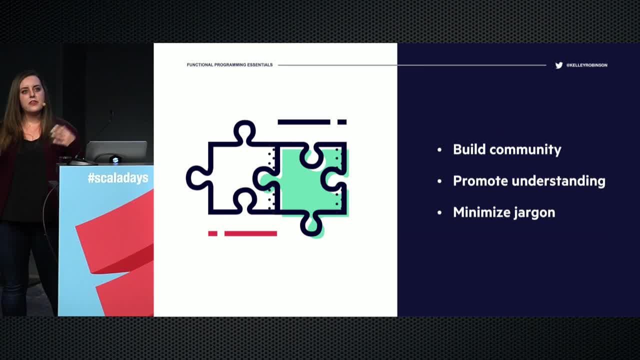 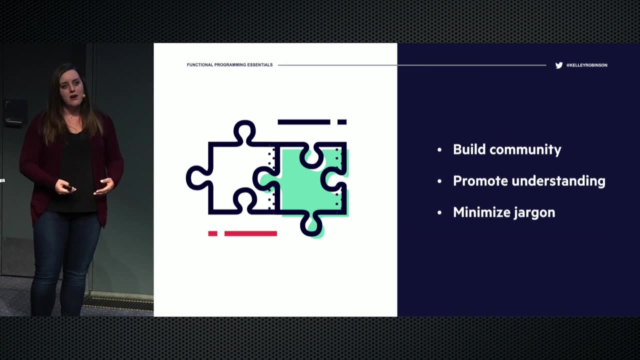 like functional programming because it's elegant, so have fun with that, but think of the principles that we discussed in order to make your data match your programs and break things down into more manageable pieces. Functional programming also exists because we needed to be able to this, because those long procedural programs are really hard to follow And so think back. 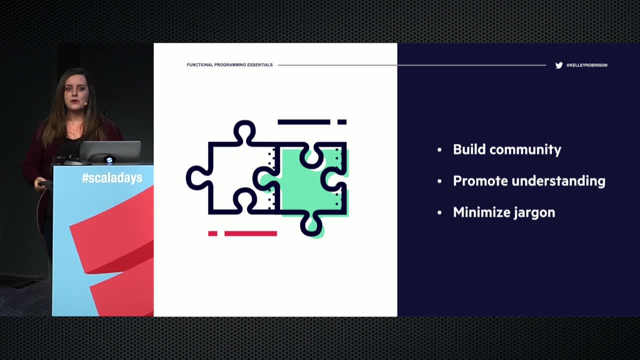 to this first principle that I mentioned From the very beginning. the whole point of the Scala and the functional programming paradigm is the idea of writing small and reusable subroutines in order to make things more understandable to the user. Do your part to encourage that. 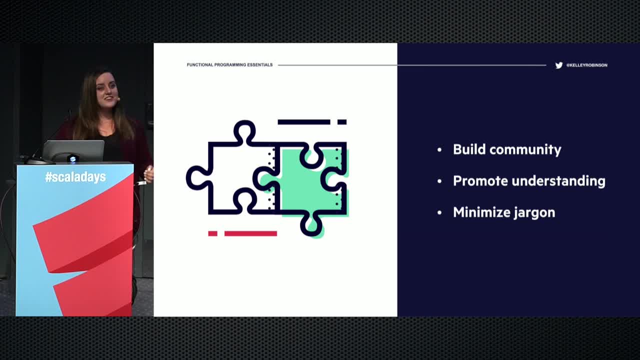 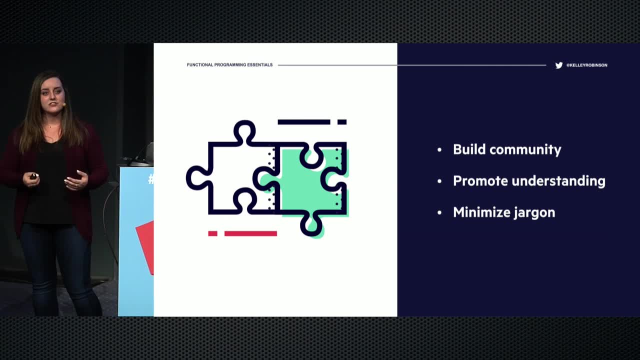 understanding And, most of all, be kind. Be kind to yourself, be kind to your teams, be kind to the community. Try to recognize when the abstraction or the syntactic sugar has gone too far or when you shouldn't introduce it at all. You always have the essentials. 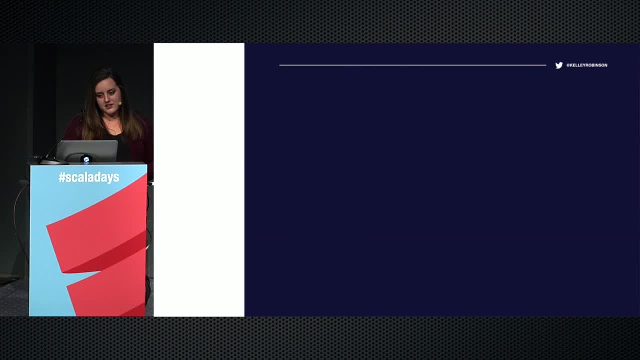 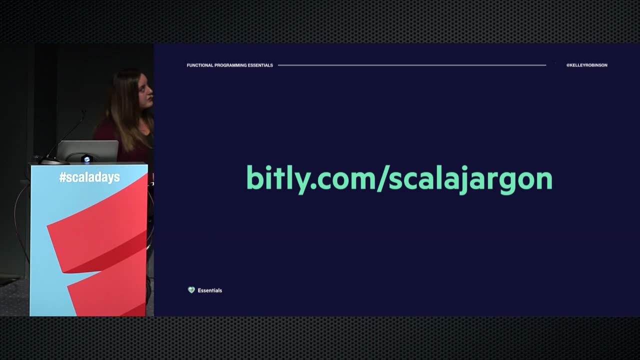 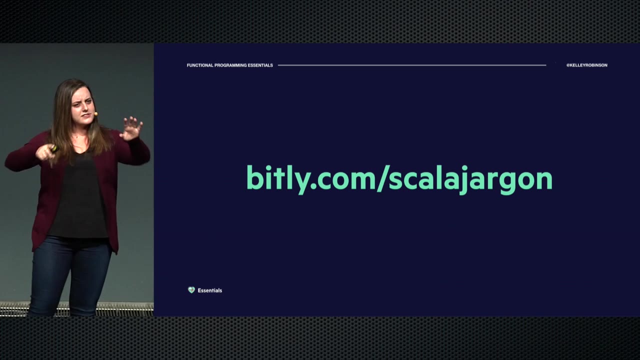 to help you achieve your goals. Speaking of jargon, we made a quiz, So you can thank Heather Miller for this. You can test your knowledge, Martin. are you here? Martin got four out of. he got about 66% on this one. 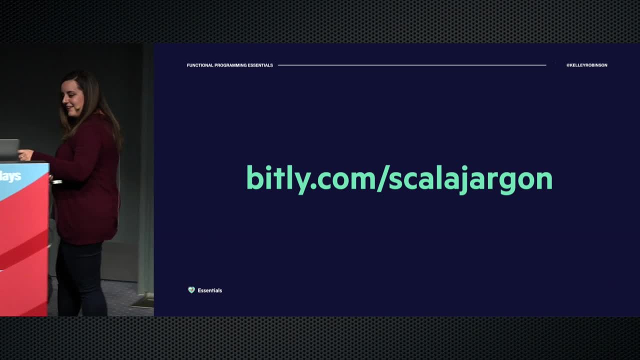 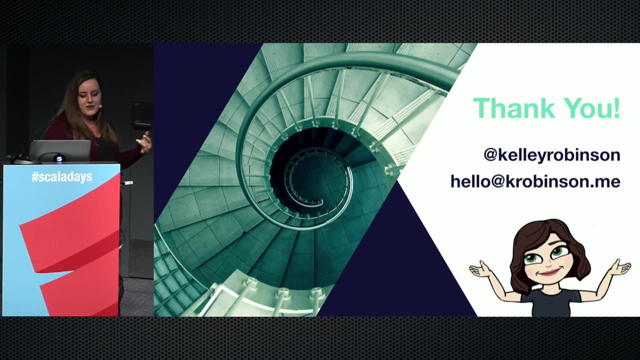 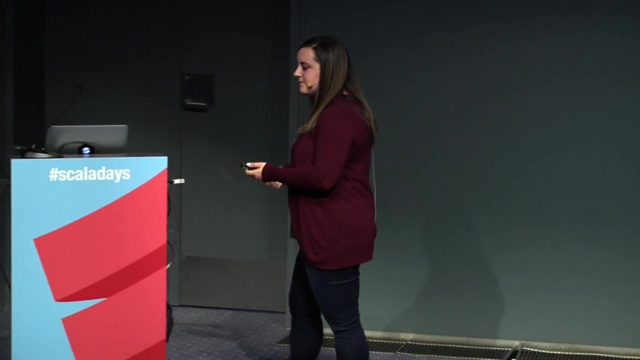 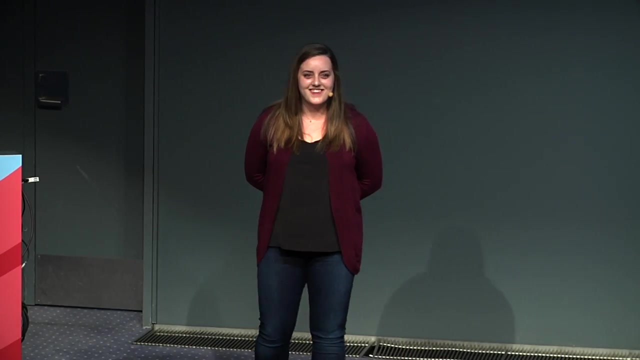 So if you can beat that, you beat Martin. It's surprisingly hard, And no cheating. Come on people. Once again, my name is Kelly Robinson, Here's my contact information And thank you for listening. I think that was really great. One remark on the word functional programming, I guess. 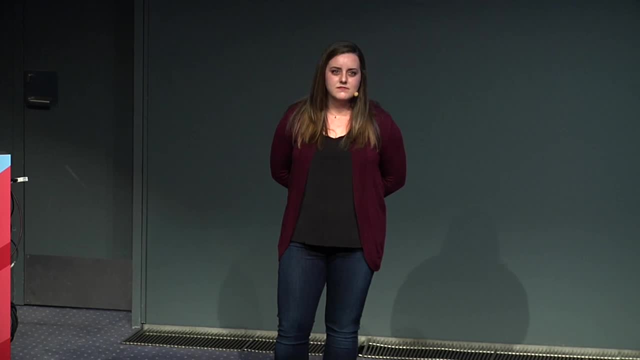 you? Yeah, I think that actually is the name of the program here, and they have actually showed its history really well. So often in this industry, which is hype-driven, there's sort of a fight for words. The last time that happened was with dynamic programming around. 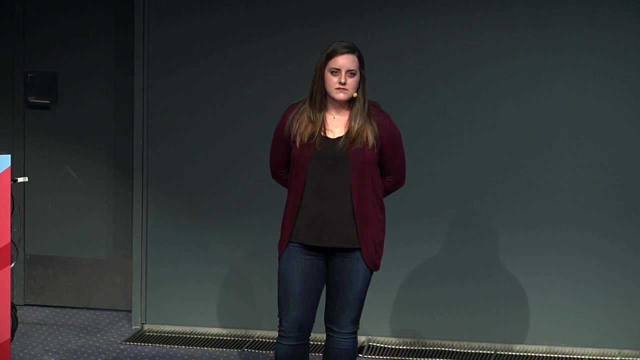 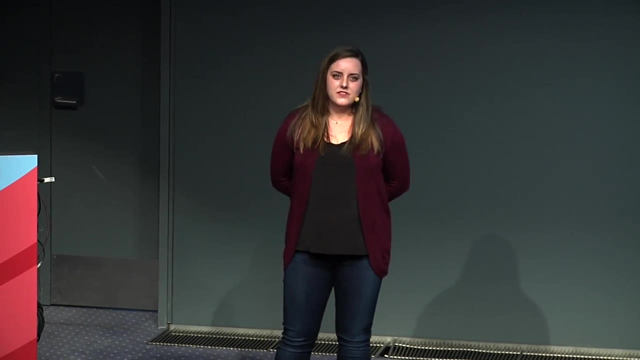 2000, which essentially was a brilliant way to essentially introduce a new term for dynamically type programming, because after all, who wants not to be a dynamic programmer? Static is boring right. I think that essentially influenced the industry for about 10 years And I believe we see something like that as functional programming. 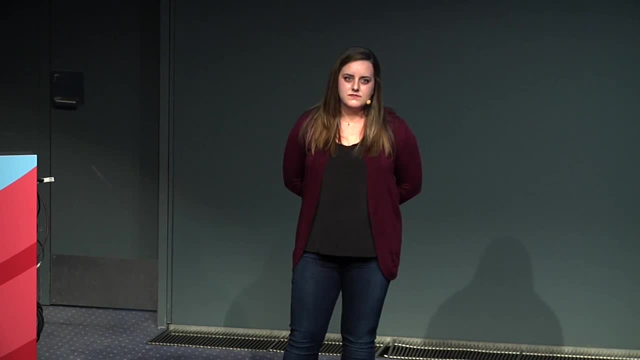 functional programming as well, because I'm in the WG 2.8, the functional programming working group, essentially of all the academics, Phil Wadler and everyone, and I can assure you that functional programming is not pro-factor optics. That's some part of functional programming. 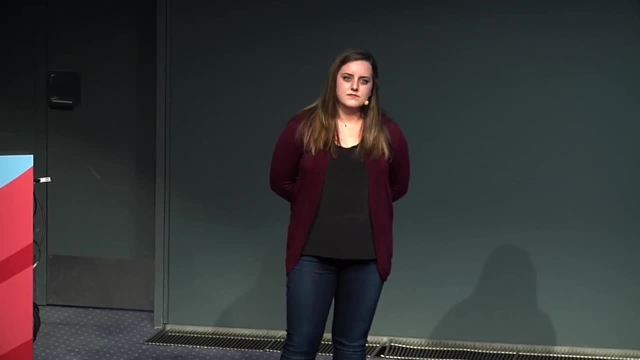 but it's essentially the part that comes from category theory. So I think a much more accurate name would be categorical programming, because that's what it really is. Functional programming, as you say, is much, much wider. It's essentially every programming that uses functions and that. 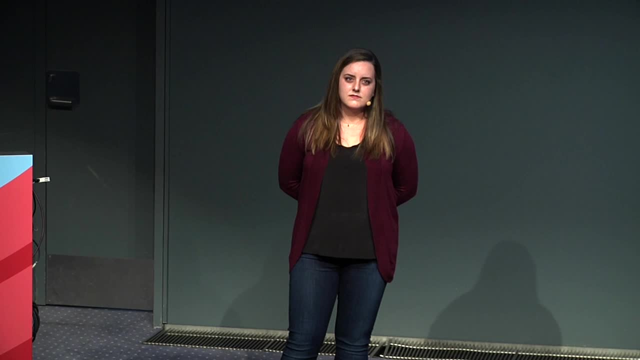 essentially tracks effects. It tries to be pure in as large a program footprint as possible and by whatever it means that achieves that. that's functional programming. Well, thank you for raising that point. I just wanted to reinforce it. Thank you. 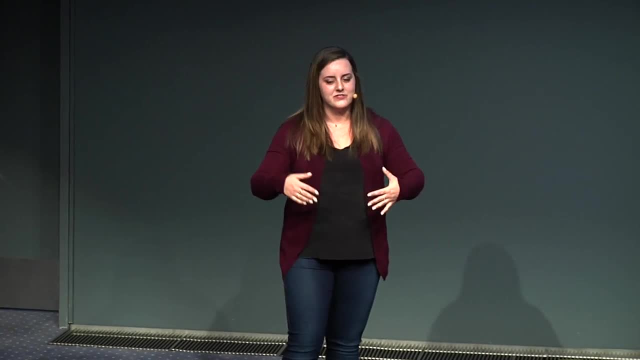 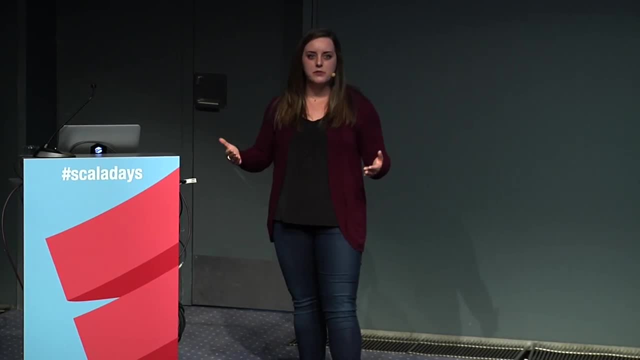 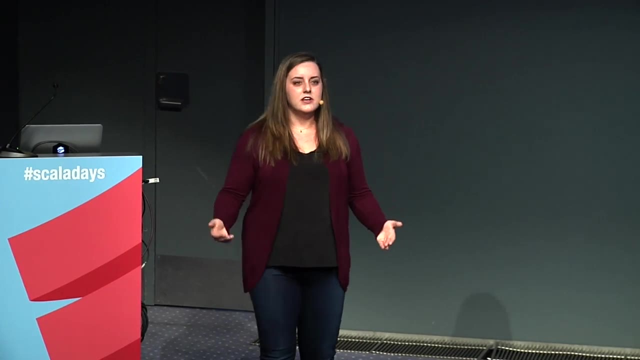 and trying to call it functional programming, and I think that's problematic, because then you get people that are interested in learning functional programming and on day two they're like: well, now I have to know what type class is and the reader monad is, and it's like: 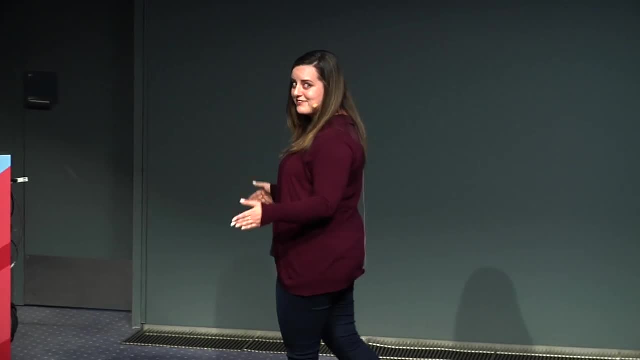 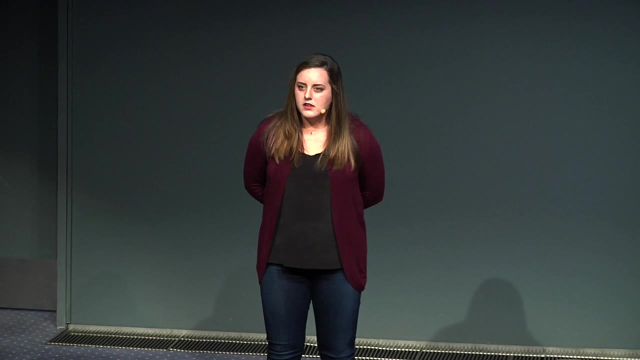 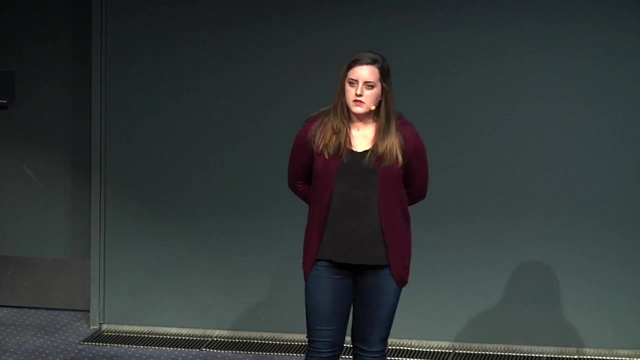 no, you don't have to know that on day two, Maybe day 200, but even then, probably not. From your experience, how do you balance between using these tools, which are category theory, implementations, and how do you implement, And which are the borders that you define in your teams? and so what's the practical? 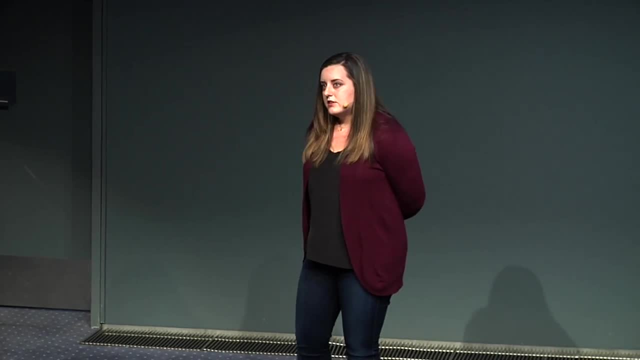 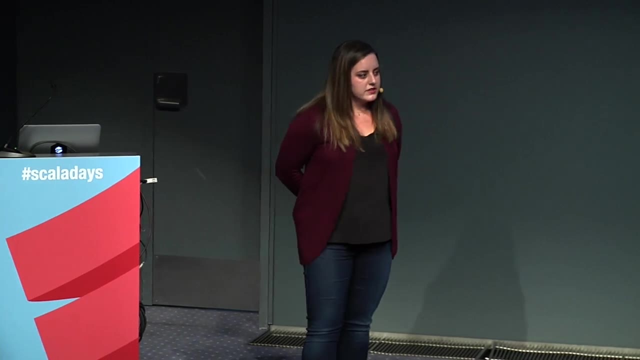 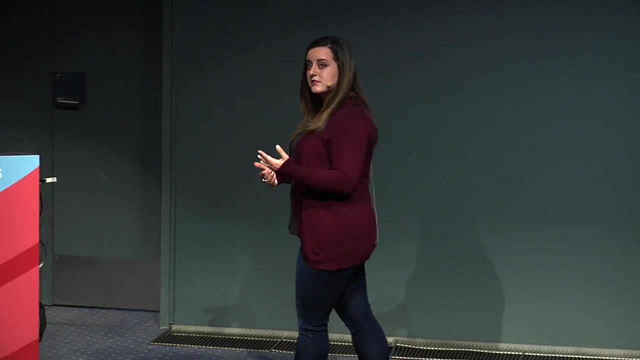 advice for usage of the libraries. Sure, so I think it really depends on who your team is and the problems that you're trying to solve, and so one of the things that I've said before is: a lot of my team comes from a Java and a Ruby background, and so when we started writing things in Scala, 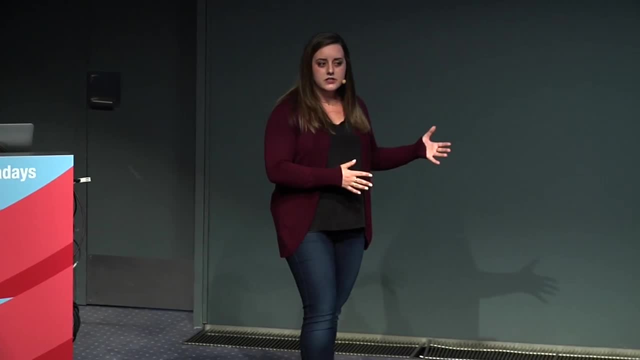 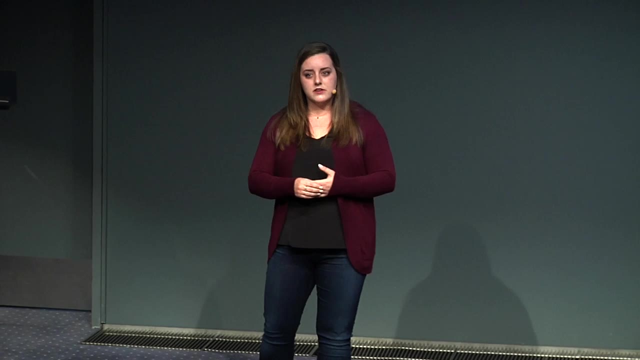 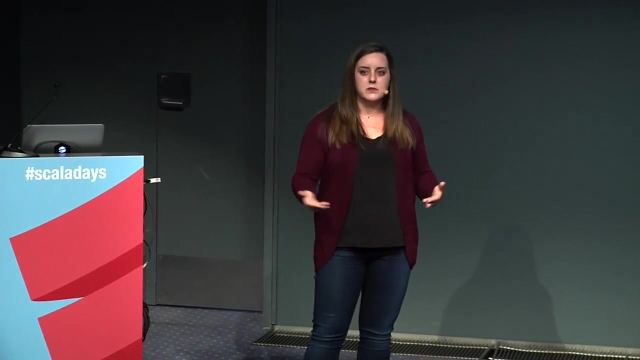 people were coming from the domain of an object-oriented language, and so there weren't a lot of people that had a lot of the category-theoretic knowledge, and so we decided to pick up Scala from that domain, and so there's not a lot of this super Haskell-y stuff that appears in our code, and that's the agreement. 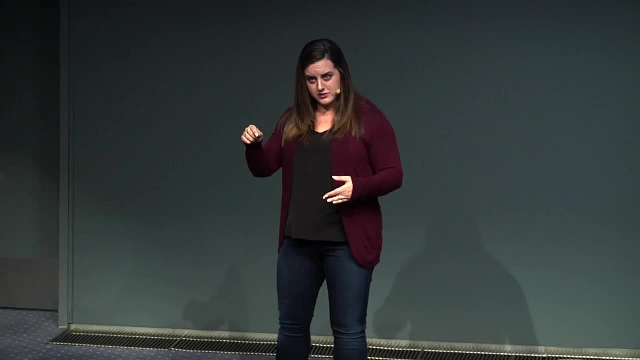 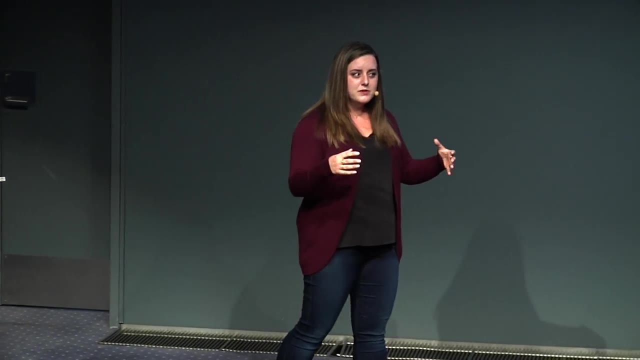 that we've come to as a team. I'm actually going to pitch a talk that's today at like 340, I think, The CTO of TapAds talking about how to build some of these principles around building teams in Scala and he has a lot of really great points around this: how you 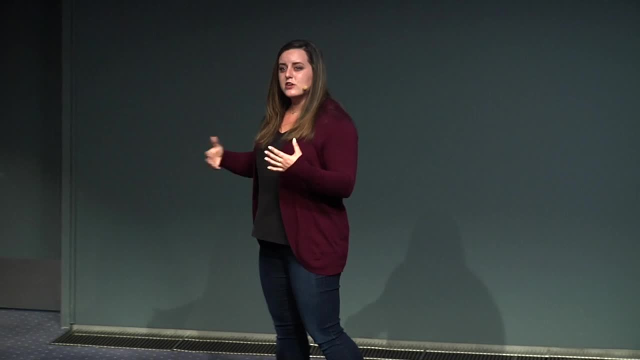 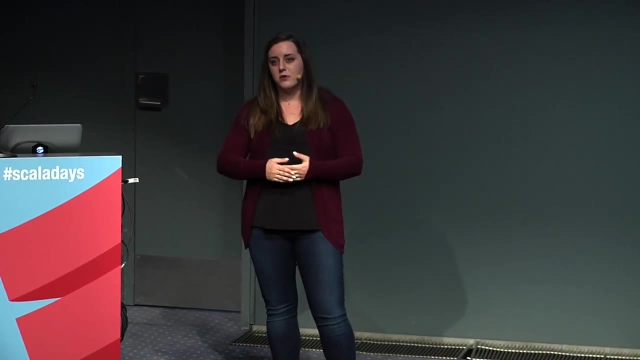 can kind of condition your teams and agree on a set of rules, and so I think it's really important that you have principles within your team in order to do that. but I don't know anything about your team. I don't know what the backgrounds of the people are. If 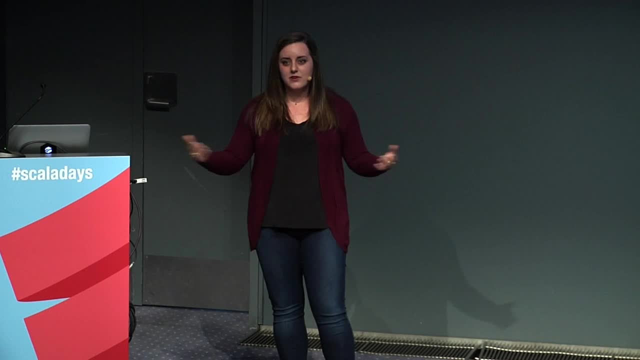 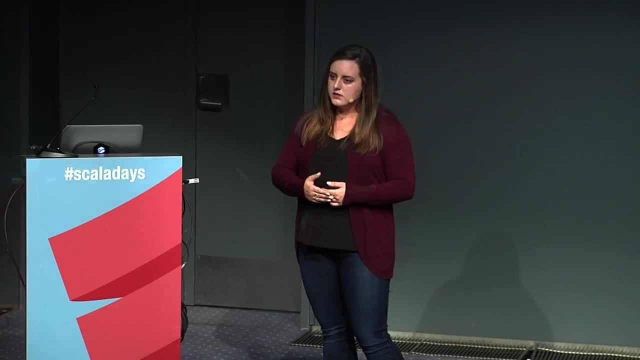 you were all coming from math PhDs, then yeah, maybe it makes sense to write everything in a very type-level, categoric style, but I find that a lot of the teams that I've worked on in Scala aren't like that. First of all, thanks. It was a great talk. You raised very interesting points on the 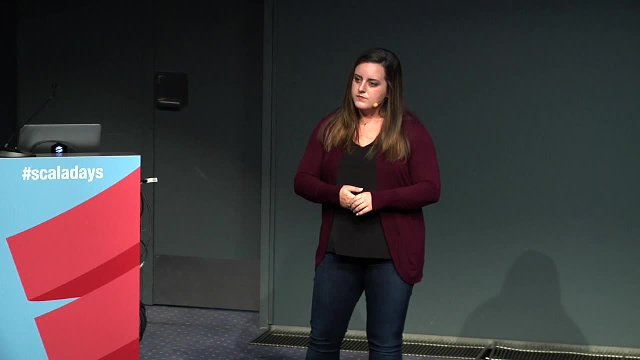 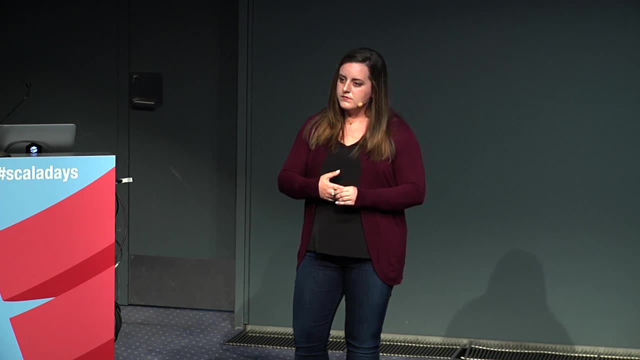 function versus categorical programming thing. I'm wondering when you speak about minimizing jargon, because to me in the process of learning concepts, even from category theory, sometimes jargon or precise definitions were actually very useful because I know what I don't know and I know what I can Google and I can find material on that. So when you 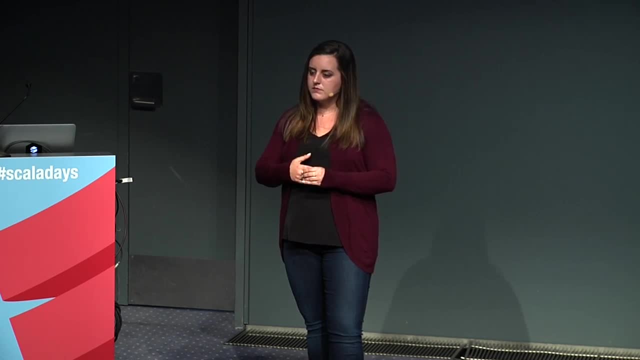 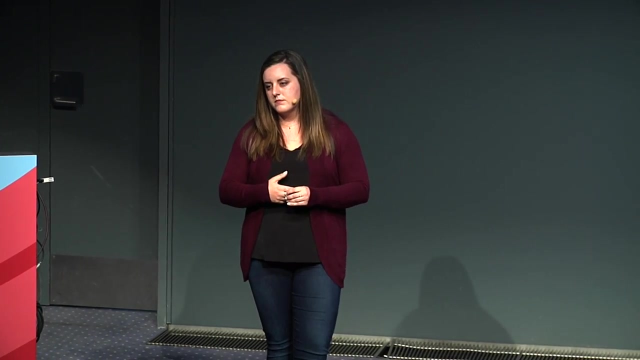 say minimize jargon, I'm wondering how does it fit in the process of learning? It seems like a cultural problem, like, essentially, don't be a jerk and don't use those words out of context, Provide context and words, Yeah. So I'm wondering whether you mean by minimizing jargon, like don't use it, when you 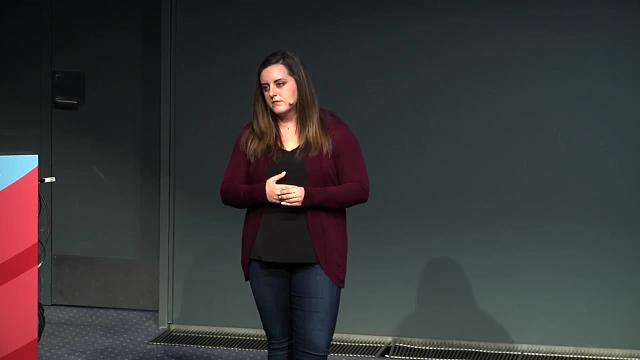 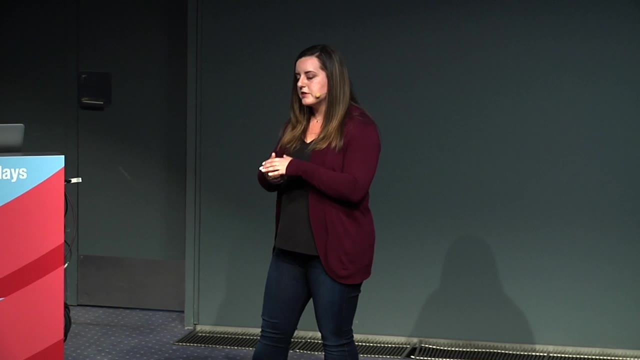 don't need it, but when you actually need it. I don't know if you have any tips for helping learners and learning Yeah. So I think it comes back to focusing on the problem that you're trying to solve, and solving that problem with the pattern or the style that you think makes sense, And 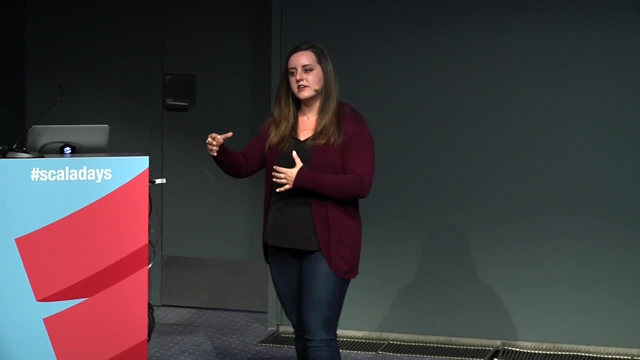 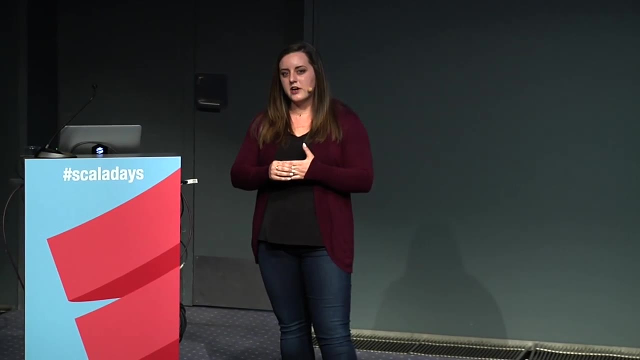 then if at a later point you recognize or someone on your team recognizes, that pattern has a name, then you can start to name things. But I think the problem where jargon comes in is if you're talking to someone and you're assuming knowledge and you're not providing.